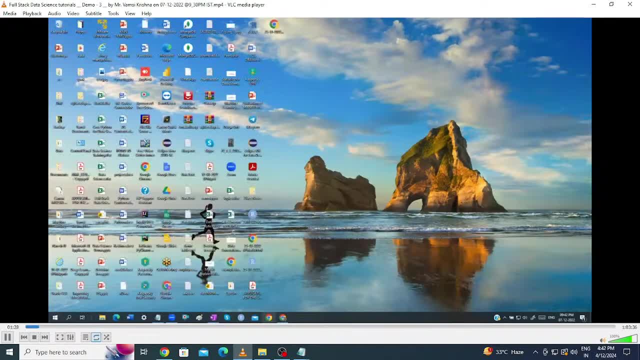 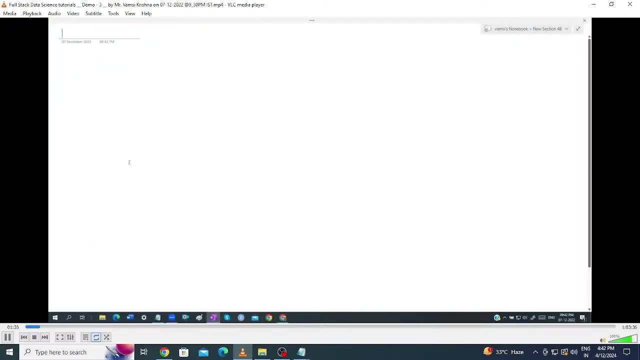 Just give me a second Right Right guys. So let us continue the session. guys, from the last discussion, what we have been gotten, So mainly, guys, we have been studied about mainly two different objects. we have been got discussed about that. 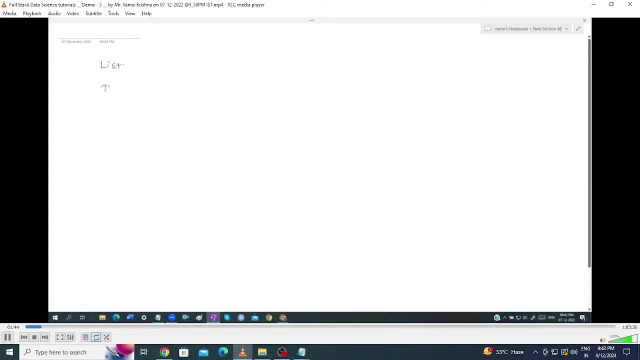 One is going to be the list and the other one is going to be nothing, but it's a tuple actually, guys. So we have spent a little bit time on the list, concept guys, because that is the first object we have been got created. 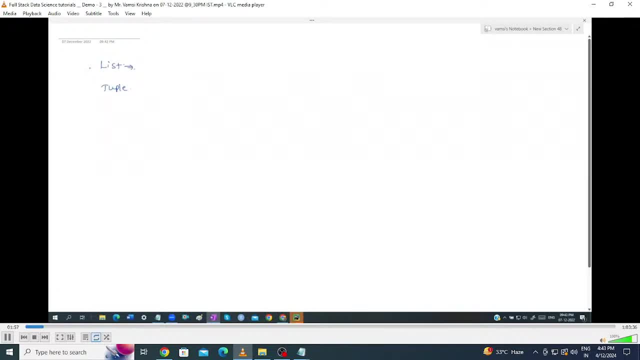 So We have to understand all the methods. It has been taken some time actually. So mainly, we have been seen how to create a list And, apart from that, how to index and how to slice them. actually, guys. 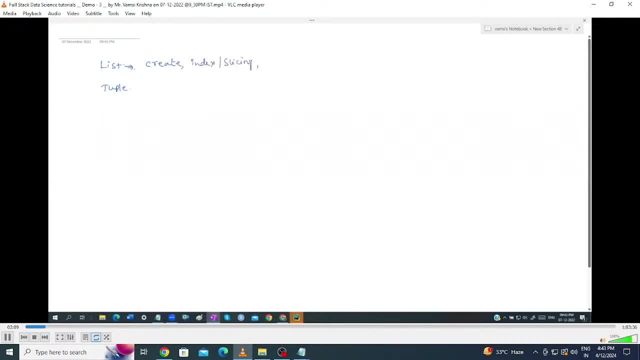 We know what is indexing and slicing. Maybe some guys who has been joined lately maybe they don't have the idea about what is indexing and slicing, but does not matter actually, guys, And apart from that, we have been discussed about the different methods actually. 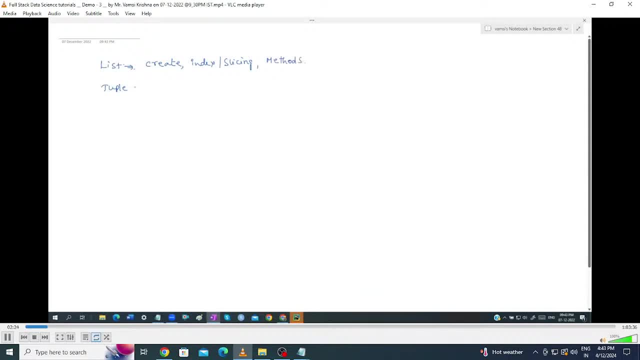 So at least we have discussed about the different methods. Same tuple, Also, guys. creating is the same. Only difference is: put them in the square brackets is a list. Put them in the parentheses is a tuple, actually, guys. Same concept. indexing and slicing is going to be same technique, actually, guys. 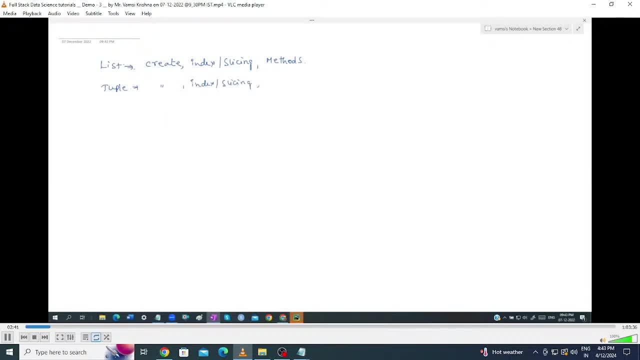 There is nothing difference will be there And, apart from that, coming to the methods. Just a minute, guys, Right. Coming to the methods. we have been seen some kind of a methods, but all the methods, whatever that appeared. So all the methods that appeared in the list may not appear in the tuple, actually, guys, because list is a different object, whereas the tuple is a different kind of an object. But similarities are there, but only the difference here is: tuple is going to be a mutable object, guys, whereas a sorry tuple is going to be an immutable object, whereas a list is going to be nothing but what. we are going to call it as an immutable object, actually. 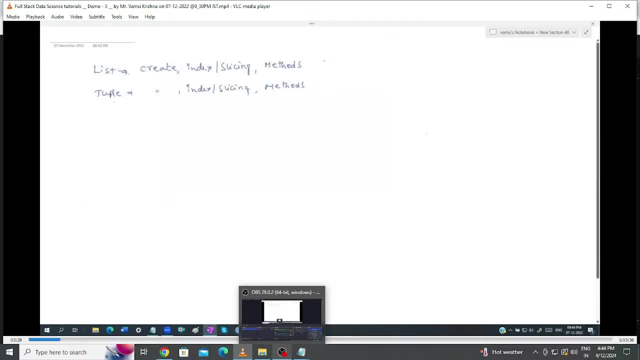 So what is the definition of, what is the meaning of mutable and immutable? actually, guys, It can be modified, guys, It can be modified. Once it has been got created, it can be modified, whereas tuple is going to be what we call it as an immutable object, what we can say it actually, guys. 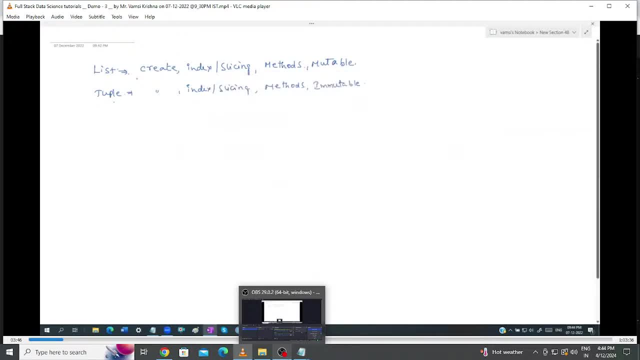 So that is the difference between what we have been got discussed about a list and a tuple, But slicing, indexing is the same actually, guys. Methods: only two methods are there in the tuple guys. What are the two Two methods we discussed, guys? 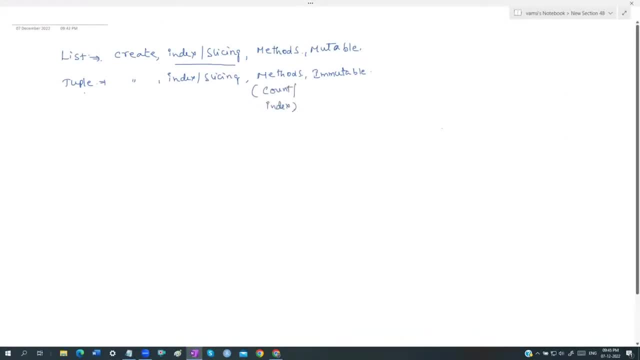 One is a count and one is an index. Only two methods are there actually, guys. Remaining methods won't work. Why? Because this we know that clear- will try to remove the element from the list. We can't add the elements. 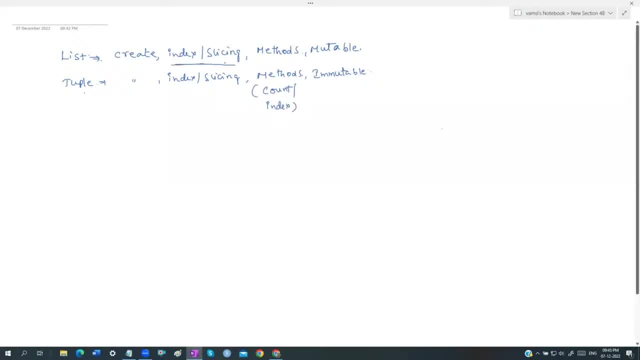 We can't remove the elements, We can't modify the elements, But indexing slicing is the same technique actually, guys, How to index and how to slice them. we know that Both of them are going to be a collection of heterogeneous values only, but not homogeneous values. okay. 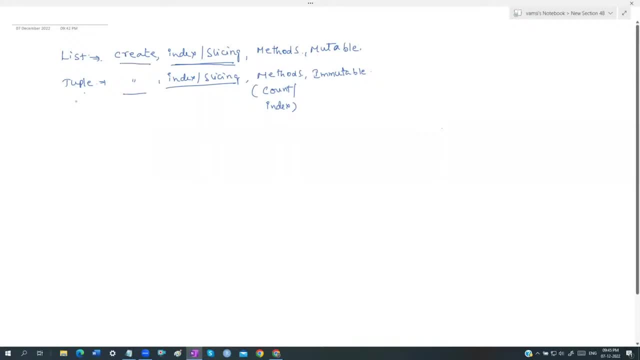 It need not to be homogeneous, But how to create a list and how to create a tuple. we have been got discussed about that, guys. okay, And just before starting the session, guys- I hope all of you have been anybody guys who has been joined for the today's class- 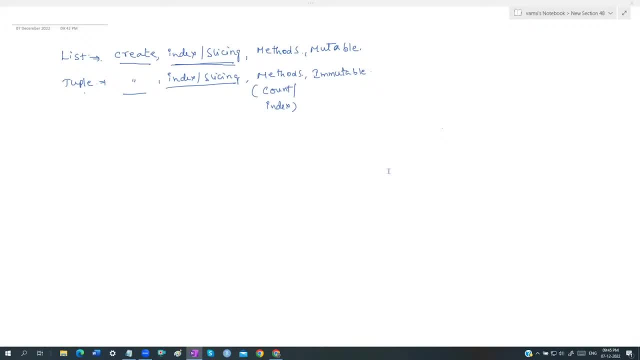 I think I can't see anybody who has been joined for the today's session. Syed, I think is your first session. Syed Hussain, No, no, I actually have joined yesterday. Okay, okay, you joined yesterday. 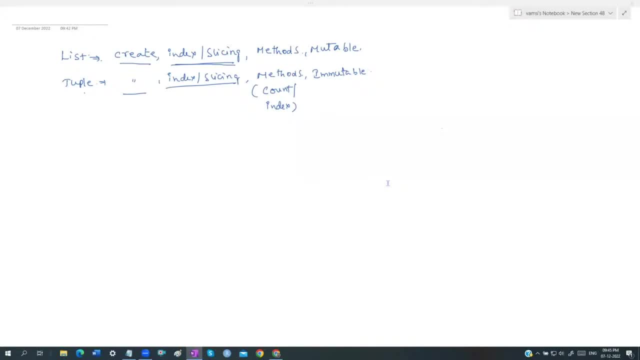 Okay, Keshav Manohar. Yeah, I think all the guys has been. you have been joined yesterday, so maybe joined yesterday or the day before yesterday, So I think. so guys, nobody is there who has been joined for the today's class. 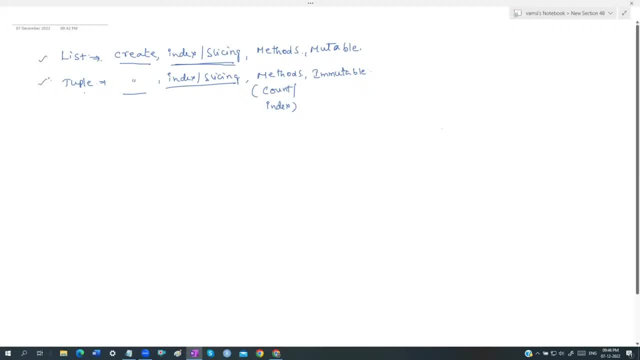 If anybody is there, please let me know, guys. Just I'll tell you what has been happened actually and how to cover the previous sessions. okay, So once again, guys, there is a list and a tuple concept is going to be there, guys. 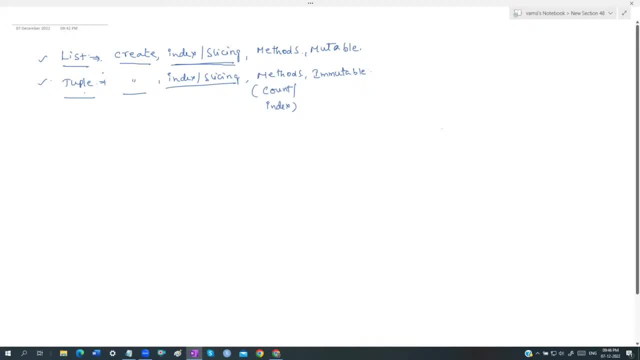 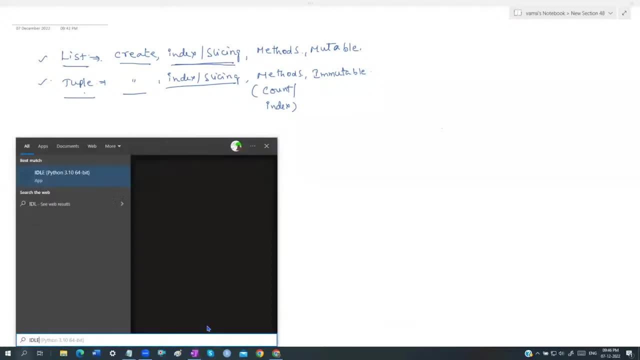 So how to create a list and how to create a tuple, just once again, quickly, two, three minutes. I'll just finish off it, guys, So that we can get some again some context And of a conclusion. what I can do is, guys, so let me open the ideal. guys, let me open the ideal. 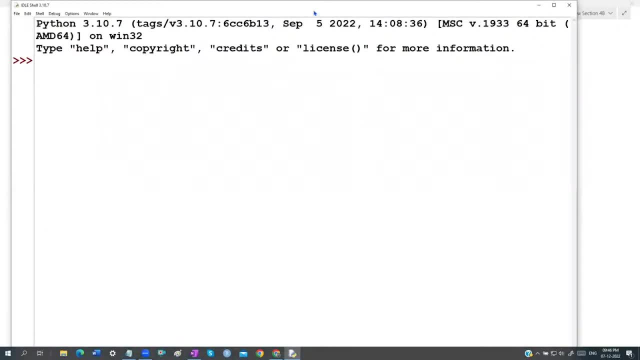 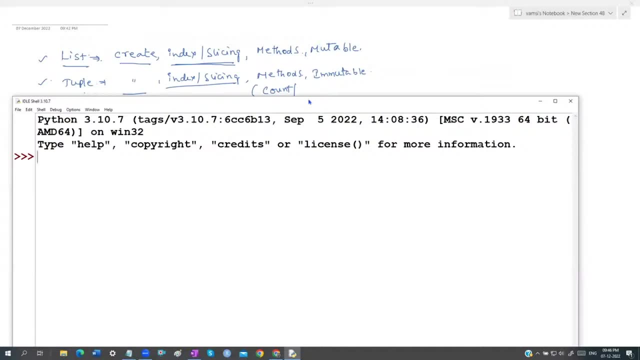 Let me open the ideal, guys. But as I told you, no, guys, we don't work with the ideal for completely. that means complete course. we cannot run it on the ideal, actually only as a beginners, only we can study them. 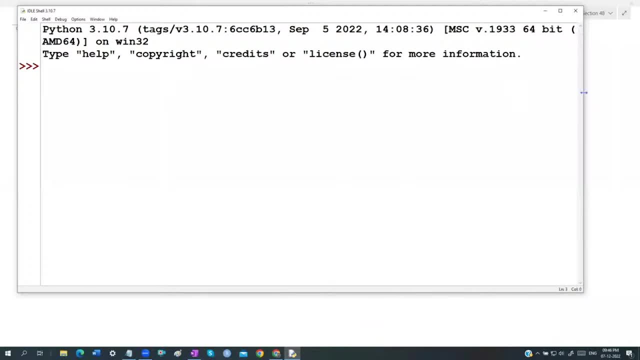 But after that we are going to use- And a better idea is we are going to be using them actually. Better ideas, we'll use it actually. Once again, guys, a quick understanding guys. let us say x is equivalent to nothing, but either I told you we can give a sequence of numbers or don't give it. 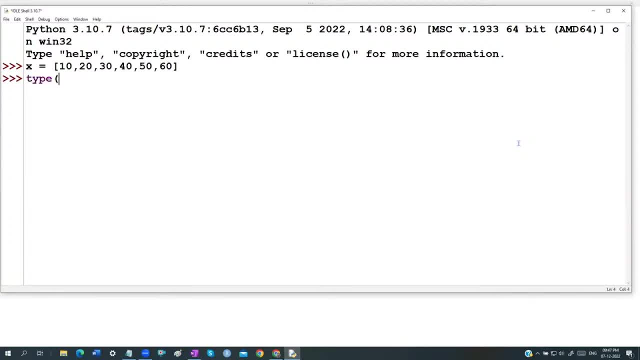 Easy to understand. I'll take it actually, guys. Type of the x. very clearly we can see x is a list. You can also ask what is the length of the x? Same example, guys. I said y equals 2, which is going to be same numbers, same numbers. I'm giving it actually, guys. 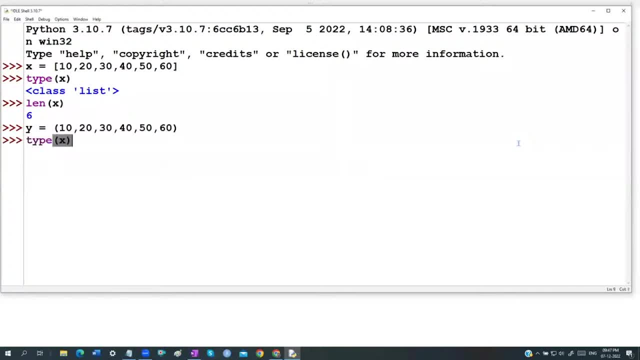 But it is going to be a tuple. actually, guys, What is the type of the x? Type is a function which will let you know about what kind of an object it is going to be there. So class x, which is nothing but it's a class list. 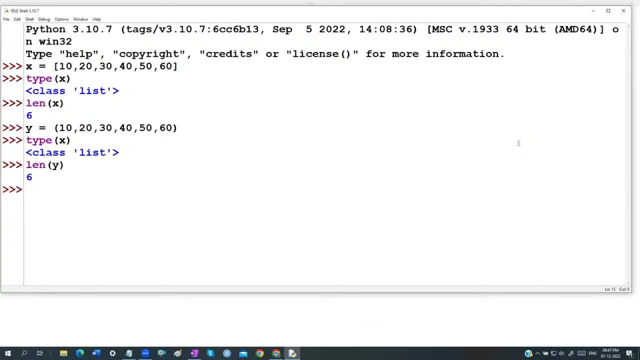 And what is the length of the y? You can see that it is going to be nothing, but the 6 is the result. Same length, same data. Print the value of x. print the value of y. Both you can find it in a same values, but both of them are going to be represented in a different way actually. 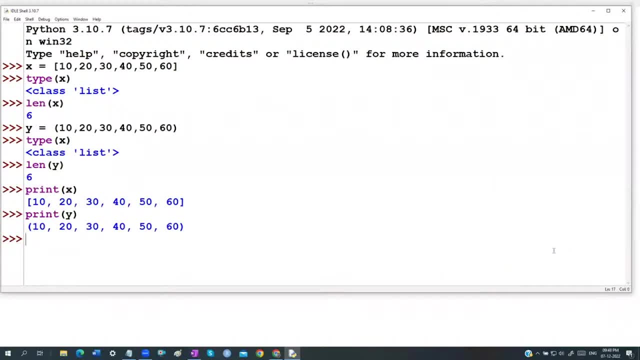 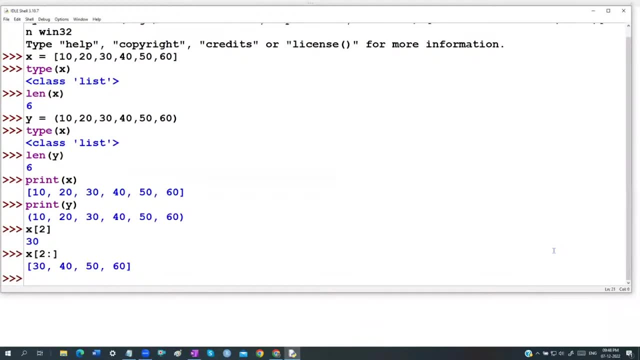 So How to slice and how to index? actually the same technique as x of 2.. We know that we are going to get a third element. x of 2 is 2, starting from the third element, we'll get the remaining elements. 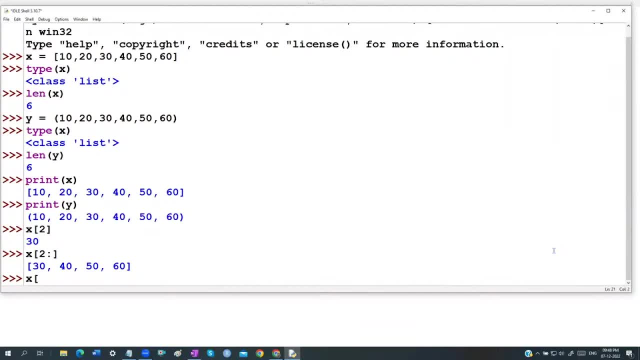 If I said x of which is going to be minus 3, minus 3 is 2, actually, guys, it is going to be nothing. but the last three elements will come. actually, Even if I said y of 2,. also the same result will come even if I said y of 2 is 2, actually, guys, but one slight difference. you have to find it off. 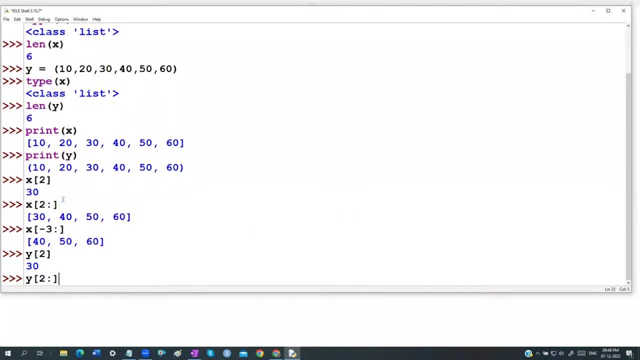 You know what is the meaning of a slice. Slice is nothing but a piece. So if I take a slice from the x, the result is again a list. only guys, You have taken a slice from a list, the result is again a list. 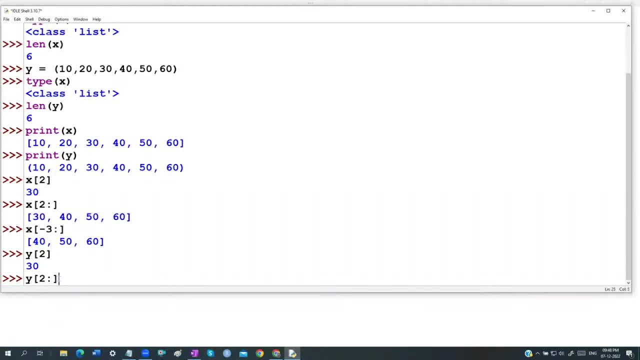 You are taking the slice from a tuple, so the result is going to be again a tuple, guys. The result is the same, but here we are getting a list and here we are getting a tuple, actually, guys. Same technique Whenever I say: y of minus 3 is 2.. 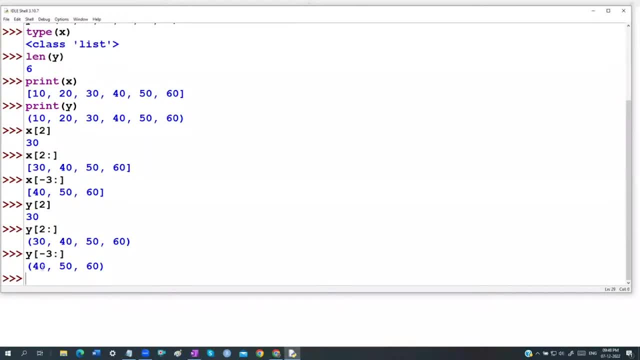 Result is the same. What is minus 3 is 2, actually, guys, It is going to be nothing but last three elements. we have to get it actually. So whenever I slice a list, we got a list. When I slice a tuple, we got a tuple. actually, guys. 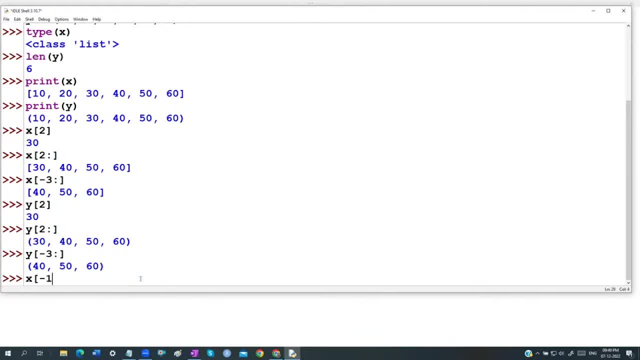 Same technique, same application. If I say x of minus 1, it is an indexing, actually guys It is y of minus 1, actually Result is the same result. Both of them are giving you only as an integer value. we are getting it actually. 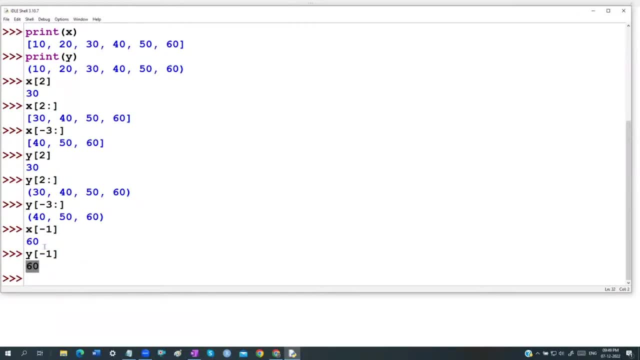 Because indexing can give you any value, But slicing will always give you a list. slicing will give a list, A tuple. slicing will again give a tuple only. But what are the methods associated with? actually, guys, When I said x dot, I told you: no, there are totally 11 methods will come. 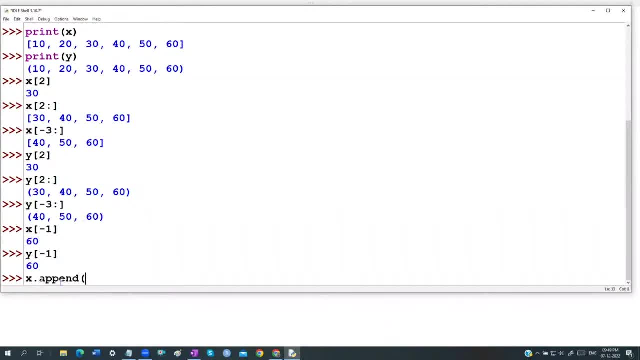 I can append the data. actually, guys, I can append the data to the x, actually 70. I can append it. But same example: if I said y dot append of 70, you will get an error actually. 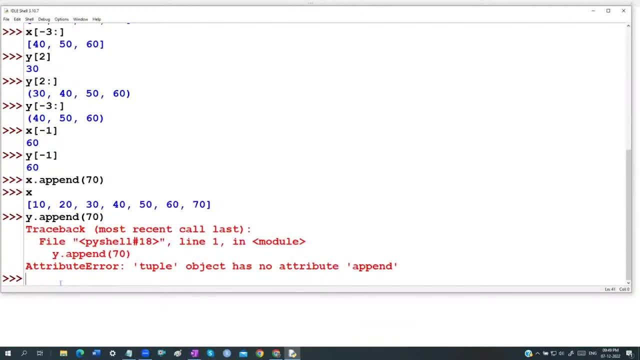 Why? Because append is a method which is associated only with a list But not with a tuple class, And tuple is an immutable object. When I said y dot, only two methods will come. actually, guys, What are the two methods we can see? 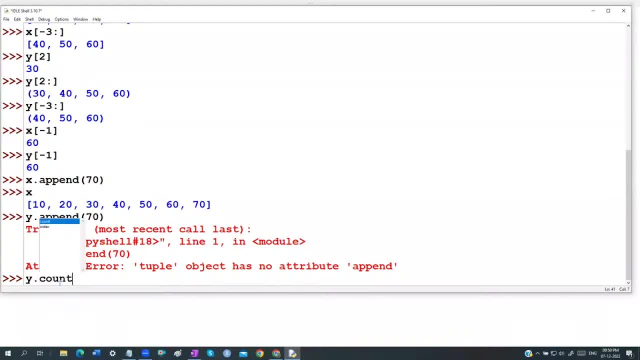 Only count and index. Only two methods. actually Count will count how many times the given value is there. Index is going to tell you where is that particular value is going to be there. actually, guys, Where is that? 30 was there. 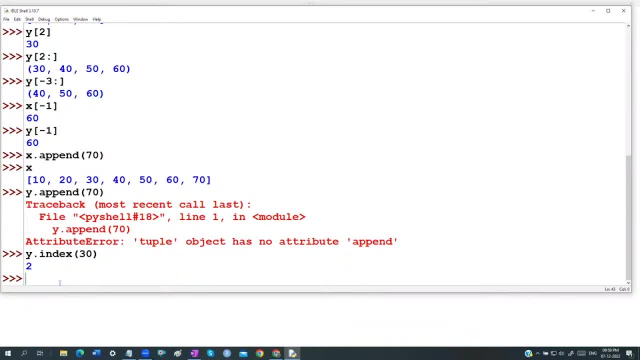 It was there in the second index. what we can say? So concept is very straightforward, guys, There is nothing complications, Nothing logical part will not be there. Everything is just. we have to know how to use it actually, guys, Okay. 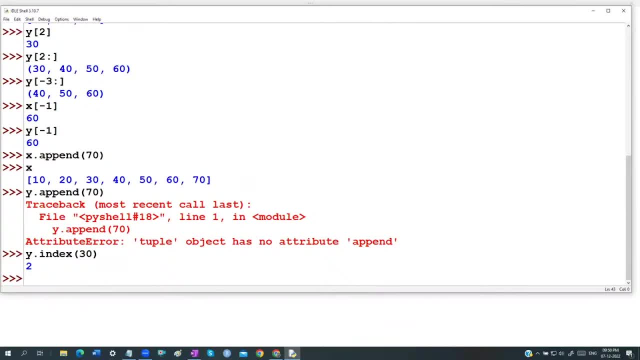 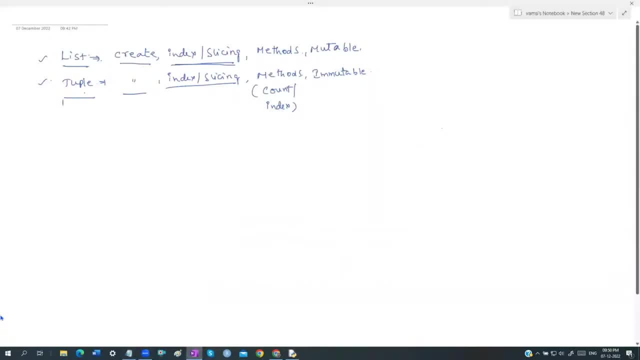 So there are two more objects, are there guys? Let me complete the two more objects And then I'll go back to the backup sessions. guys, I'll talk to the guys And then I'll decide it. Really, do you require a backup session? 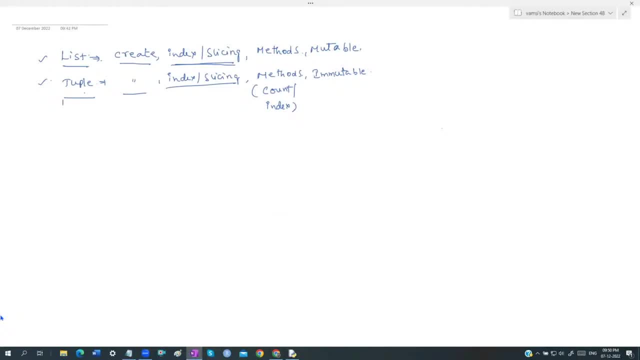 Or do you can manage, I can explain them. According to that, I will take a backup session. Let me complete. Maybe today, tomorrow I'll complete, of it actually guys. So today we are going to be discussing: 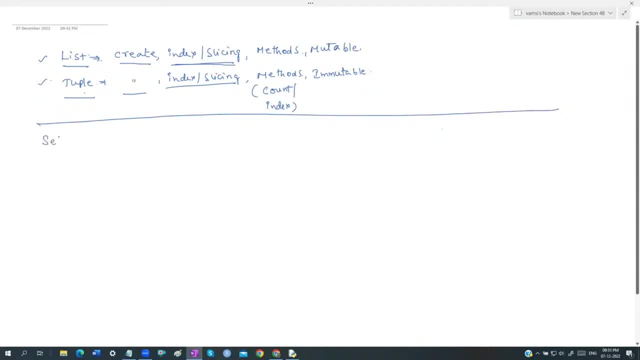 About a new object called as, which is going to be nothing but a set object Completely. the today's session will be on the set object. actually, guys. Concept is simple, But only the thing is: more and more functionalities are there. 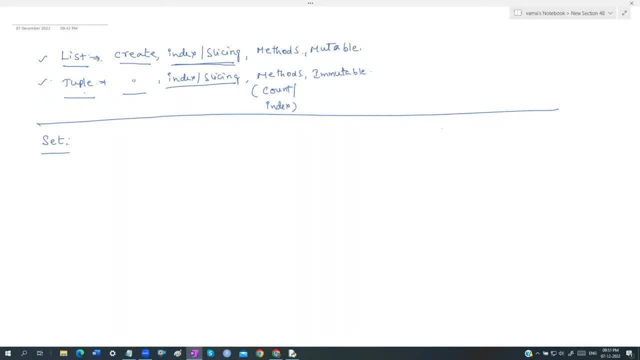 So I have to explain those particular topics, actually, guys. So once again, which is going to be nothing but the same concept, what we are going to be doing is going to be nothing but what we can say, that it is going to be a set object. actually, guys, 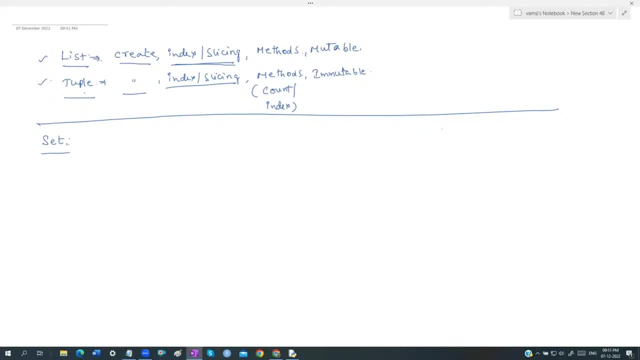 Okay, It is going to be a set, Set object. what we are going to be gets calling it as actually guys. So whenever I'm talking about, whenever I'm talking about a set object, you can say that you, what generally that comes to your mind, actually guys. 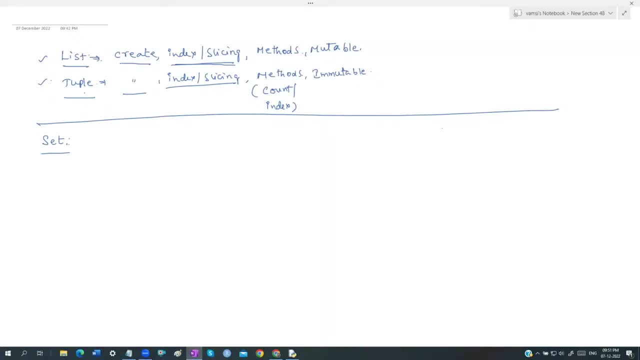 What, generally, that comes to your mind? actually, guys, which is going to be nothing, but We can say that something like an it is going to be in mathematics, You remember? no, guys, that is going to be nothing but sets and relations, set operations. 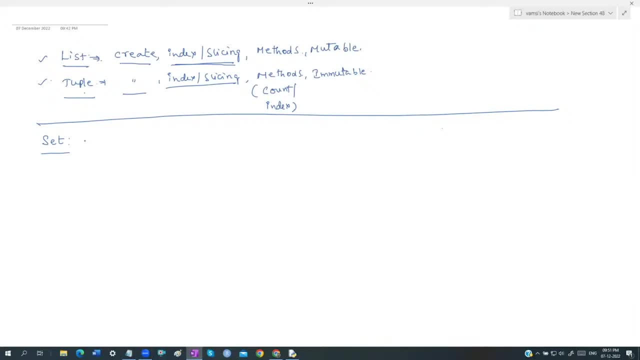 Okay, Which is going to be something like an intersect. Okay. Okay, We have union. We have something called as a minus. I hope you remember it, guys. We are working with something like an set operator subset. It is going to be super set. we are having 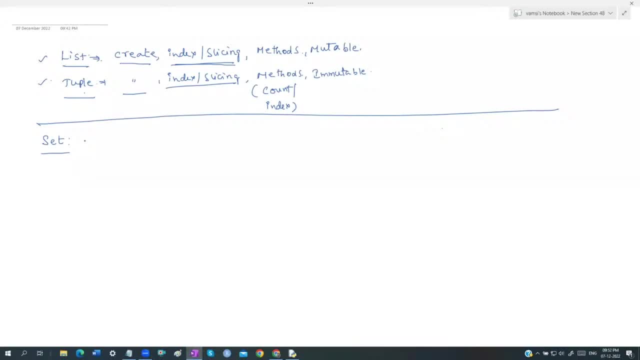 So same topic is going to be set concept: actually guys. So in mathematics also, you remember guys, how do you represent a set A? It is going to be like this: We are going to be representing, actually guys. 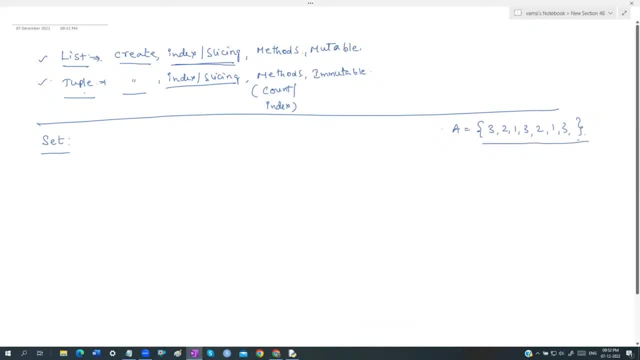 It is enclosed within curly brackets, actually like this, or curly braces, or curly brackets. What is a set actually, guys? Set is also. what is the difference between list and tuple? Both of them are going to be same And one more thing is going to be nothing. but one more thing is going to be nothing, but both of them are same. 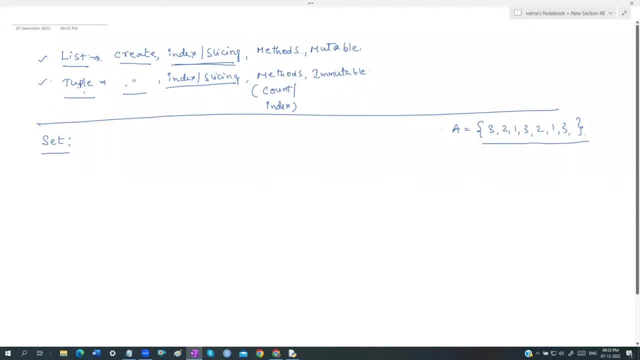 And one more thing is going to be nothing, but only just is: both of them are homogeneous or heterogeneous. One is a mutable, one is an immutable. What is a set object actually, guys? Set object is going to be nothing but what we are going to call it as, and, guys, it is nothing but an unordered list. 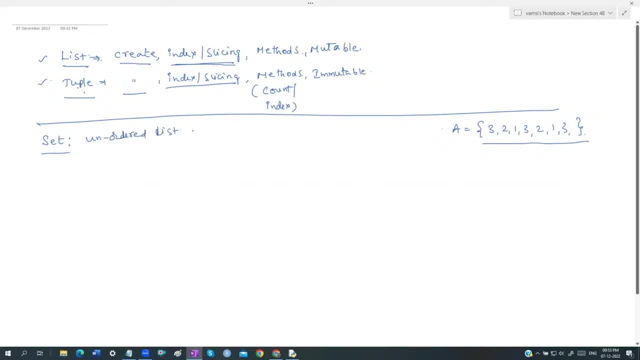 What is meaning of unordered list? actually, guys, Unordered list. I will tell you I did not complete it. actually, guys. What is meaning of an unordered list means, For example, in a list, when you are creating a list, if I give the values like 10, sorry, 20,, 10,, 30,, 40, if I give the values like this, guys, when I print the value of X, it will maintain the same order actually. 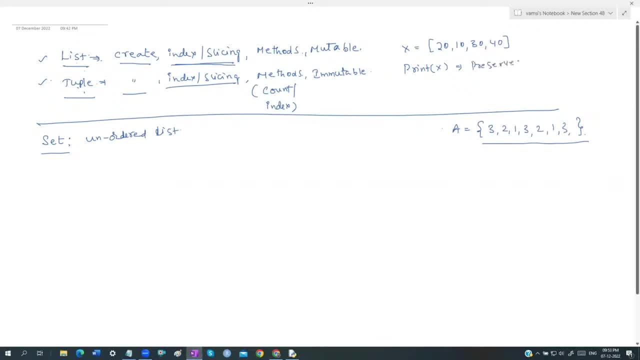 So it is going to preserve the order? actually We will say that it will preserve the order. actually, It will preserve the order Even whenever I work with the tuple also, the same order is maintained. Which order you give, same order it will maintain. 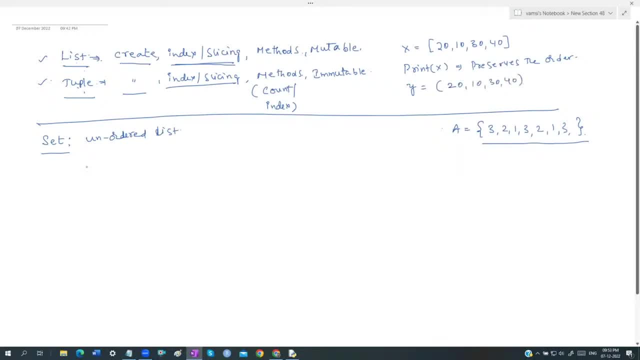 It does not change the order, actually, guys. But what is meaning of a set is unordered list. actually, What is meaning of an unordered list means You give one value, you give some order, we will get a different order, guys. 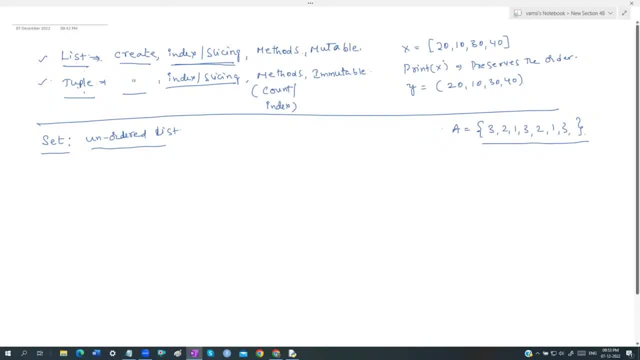 You give some order, we will get a different order. If I give this order, there is no guarantee that it will get the same. It does not preserve the order. actually, It does not preserve the order. It is an unordered list of one more thing, actually, guys. 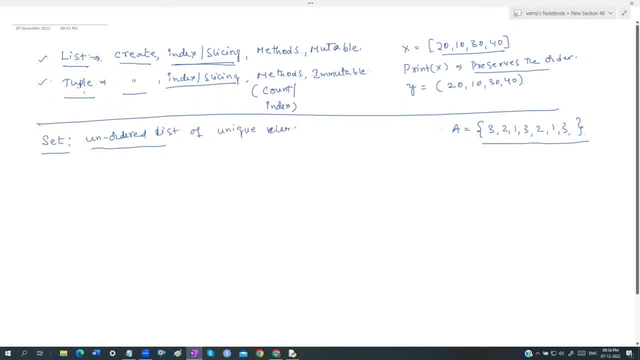 It is an unordered list of unique elements. You know what is meaning of unique elements, actually, guys, The values or the elements which cannot be repeated. But in list, we know this, actually, guys, We can have multiple times. I can have the same number as many times you can have it. 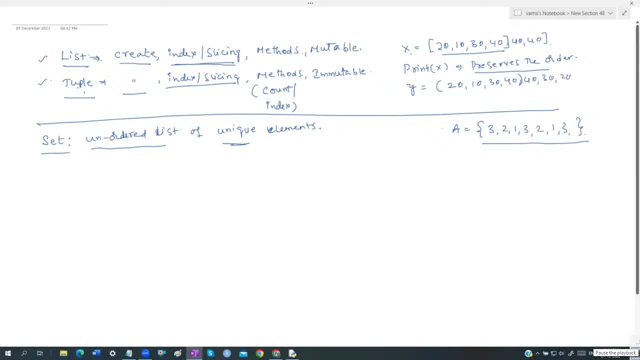 Even in the tuple also. you can have the same number as many times you can have it. Even in the tuple also. you can have the same element repeated number of times. But when it comes to the list, only two features are there, guys. 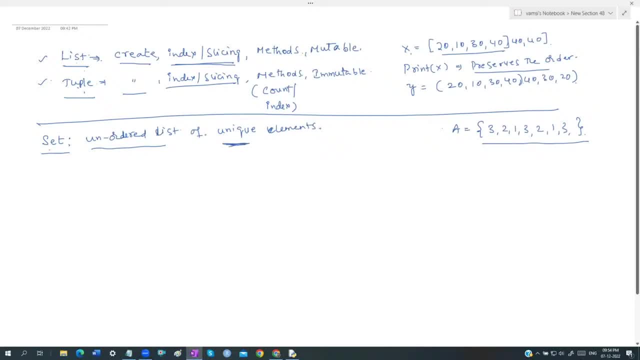 One is unique elements. That means the value should be. the element should be there only for one time. The element should be there only for one time only. It is going to be what we are going to be doing- this, actually, Okay. 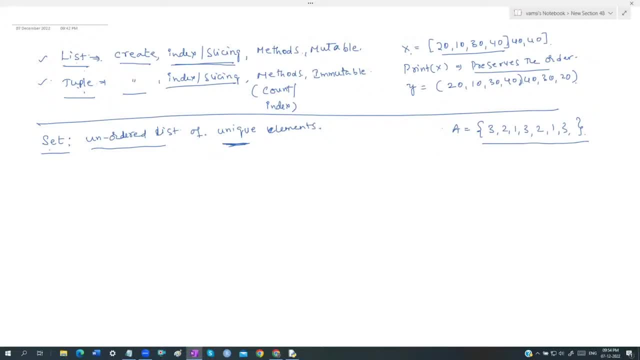 So this is going to be the one what we can say, that And one more thing is going to be nothing, but You can say. that, which is going to be what we can say is: It is going to be something like Like an unordered list of values, actually, guys. 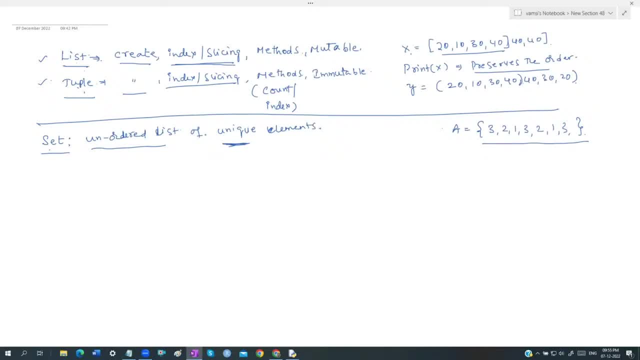 What we mean to say. an unordered list of values means, Whatever the order we give, it does not use the same order as it is. It gives something a different order. We are going to get it. actually, guys, We will get a different order. 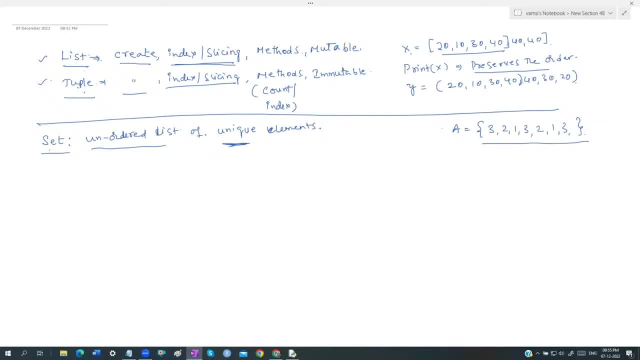 Your input is one order but your output is another order, So due to it does not maintain that order. Indexing and slicing is not allowed on the set object. guys, It is going to be indexing and slicing, So we cannot get from a set. if I want to get third element means we can't get it, actually, guys. 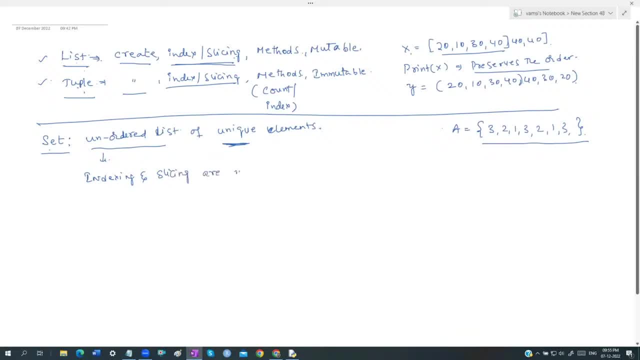 Indexing and slicing is are not allowed. actually, They are not allowed. on, the indexing and slicing are going to be not allowed. Why it is not allowed? actually, guys, Because whatever the order we give is different. Whatever the order that comes is going to be different actually. 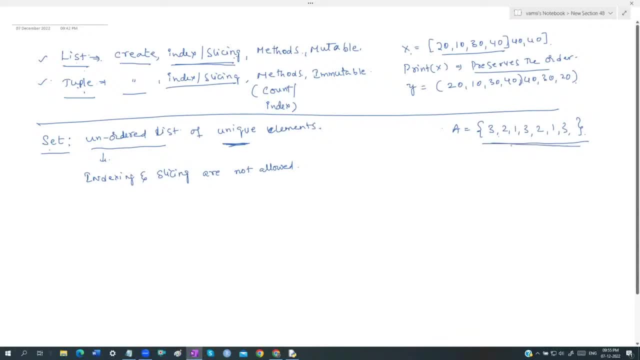 And that too, if I give the values, even if I give the values like this, guys, You give the values, repeated values, you give it, It does not throws any error, But it takes only unique values only will be selected. actually, guys. 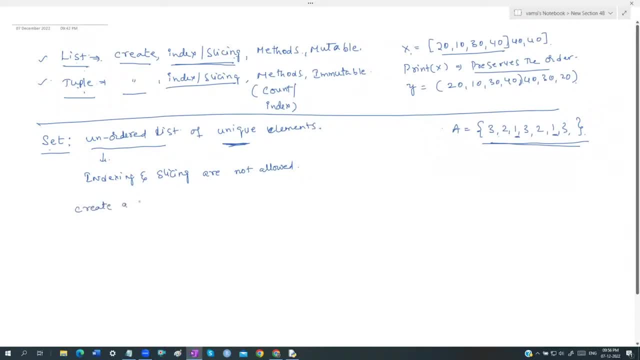 But how do you create a list, Sorry? how do you create a set? Create a set by enclosing in parenthesis, sorry, enclosing in the curly brackets. actually, guys, The curly braces or the curly brackets. Very simple, guys. So square brackets. if we enclose, it will become a list. 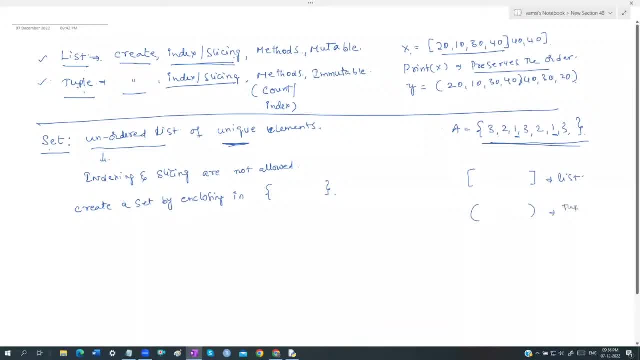 And if I use a parenthesis, and we are going to call it as an H-tuple, And whenever I use a curly brackets, which is going to be something, what we are going to call it as an S-set object, what we can call it as. 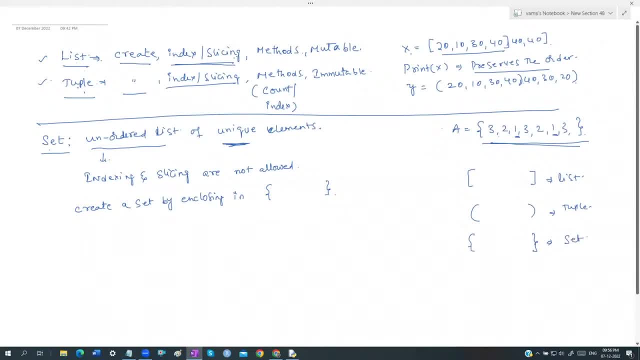 So for a normal, if I show the same example to a C-programmer, tell me, if I said X equals to this much, what is the type of the object it is? He cannot say about that In C language because C programming, Java programming, 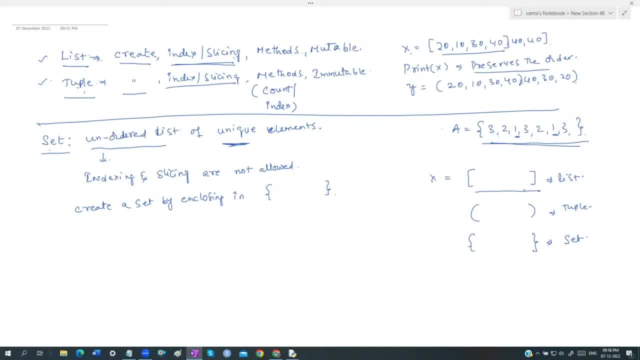 we are having an habit of writing list tuple set something. we have to use the keywords actually, But in Python you do not use any keywords actually, guys, X equals to square brackets, Y is equals to some parenthesis. 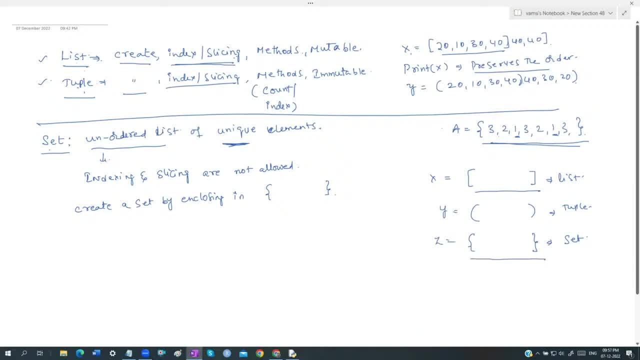 Z is equals to curly braces. It will automatically become a set, But it does not preserve the order, actually, guys. And it is going to accept only unique values, only Being. the order is not preserved, so indexing and slicing is going to be not allowed on this particular set object. actually, guys. 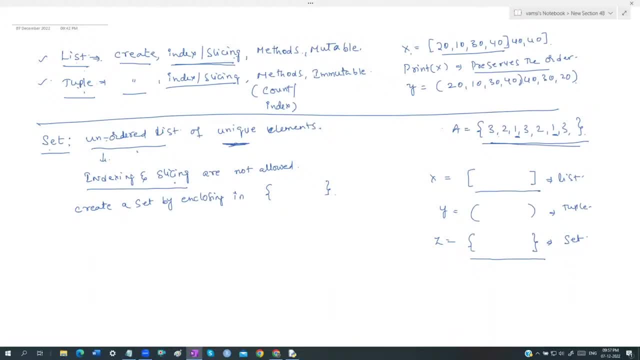 Indexing and slicing is going to be not allowed on this particular object. what we are going to be getting, this actually guys. Okay, So that is going to be The concept of how we are going to be gets working with the set object. 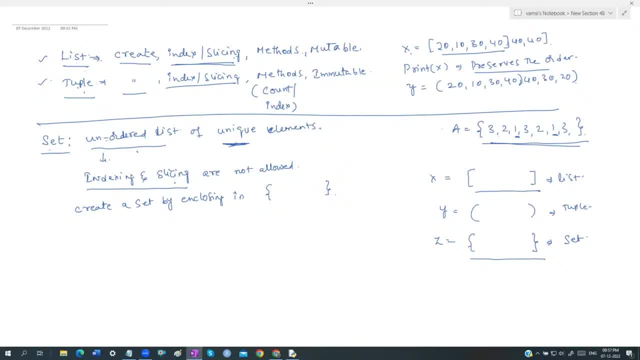 But we have a number of methods are there guys? But nothing is there. Only thing is: I have to just do some practice on that. It will take some time, But otherwise it is going to be a very simple. techniques only, guys. 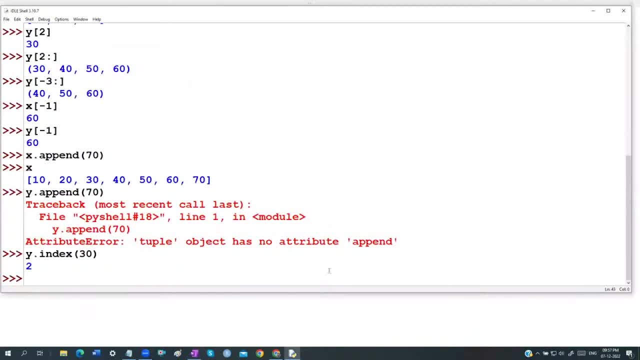 Let me create the set objects. How do you create the set objects? actually, guys. Let us say: S1 equals to, for example, guys, Just, we have to use the curly brackets. Just use the curly brackets, actually, guys. 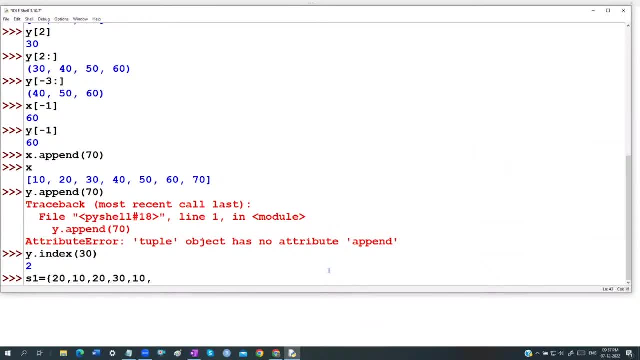 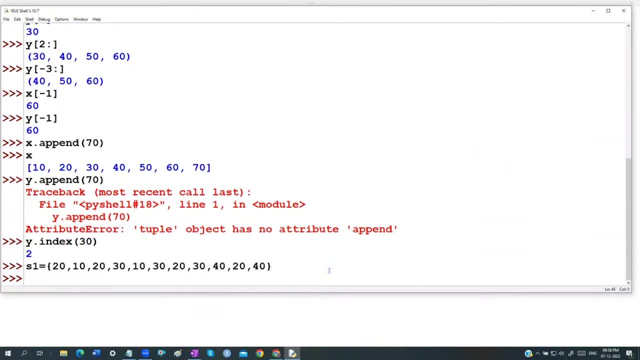 20, 10.. Again a 20.. 30, 10.. Let us say 30, again 20, 40.. Whatever the data you give, you can give it actually guys. Just I am giving some few values, actually guys. 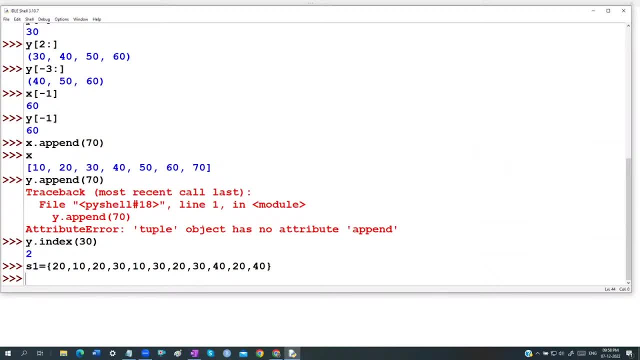 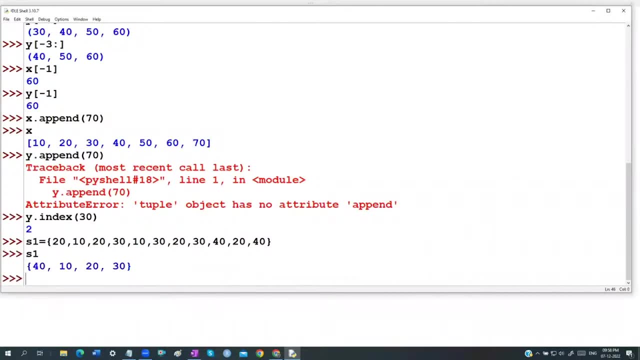 So do not think that I have given some 1,, 2,, 3,, 4,, 5,, 6,, 7,, 8,, 9,, 10, 11 values. If I print the value of S1, see whatever the output we are going to get, it actually guys. 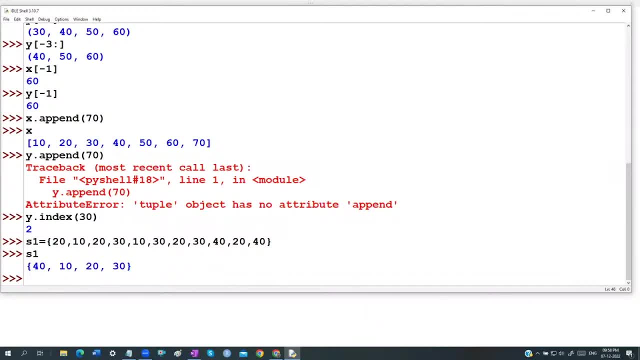 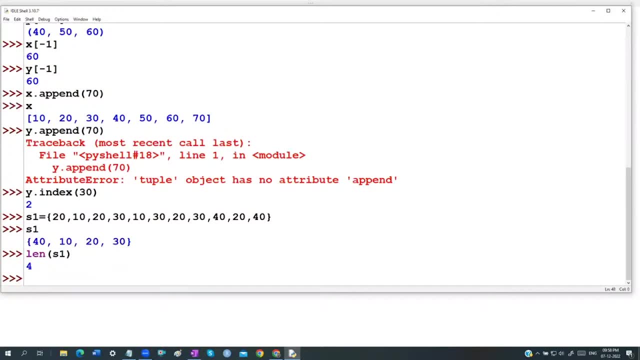 See the S1, actually guys 40,, 10,, 20, and 30. Even if I said length of S1, actually guys, Length of S1 is not going to be 11.. I have given 11 elements. 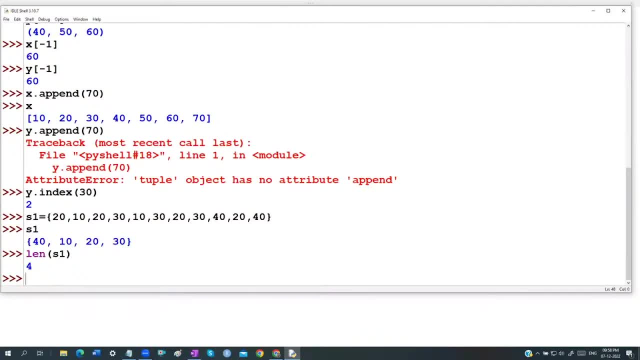 But when I said length of S1, you can see that there are going to be only 4 elements are there Because it will take only the unique values. only we can take it. If you have any doubt, I told you guys. 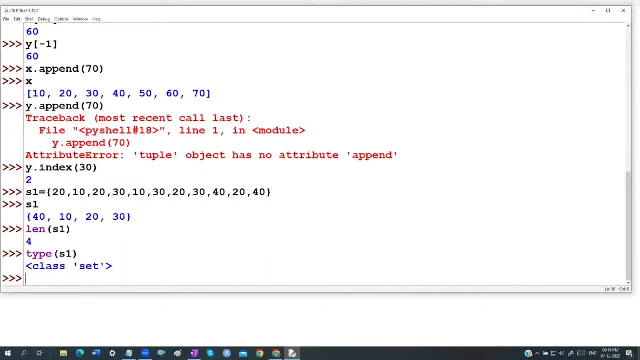 Use the function called as an type function. What is the type of the S1? It is clearly saying that it is a set object. That is it, guys. Just very simple. It is S1.. What is going to be the S1 here now? 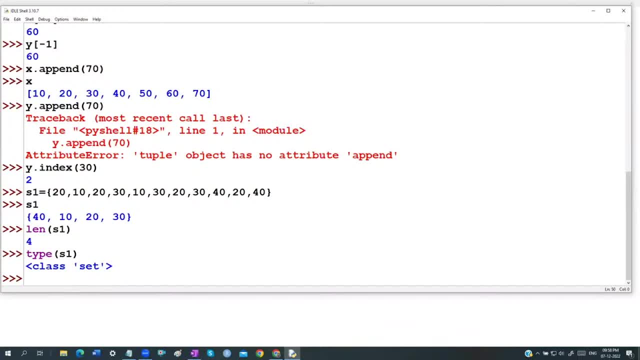 It is a list object. So what is the length of the S1?? Instead of giving 11, we are getting only 4 only. Why it is only 4?? Why? Because this we know that It is going to be a collection of only unique elements, only what we can see. 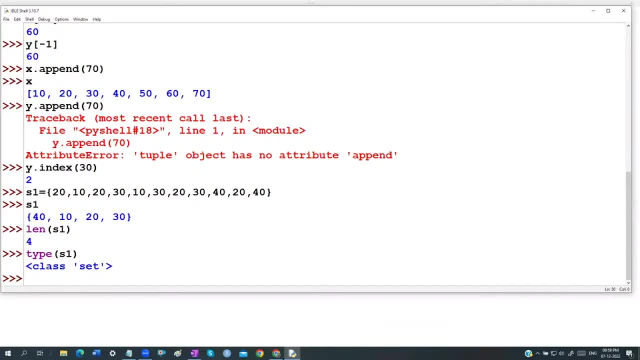 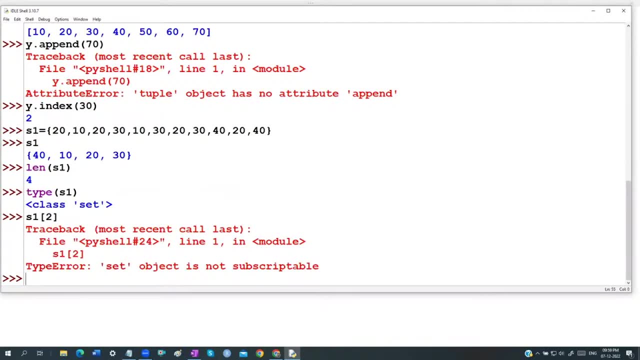 And what is the first point I told you, guys? Indexing and slicing is not allowed, So S1 of which is going to be 2.. This is not allowed, actually, guys. Set object is not subscriptable. We cannot subscript it, actually, guys. 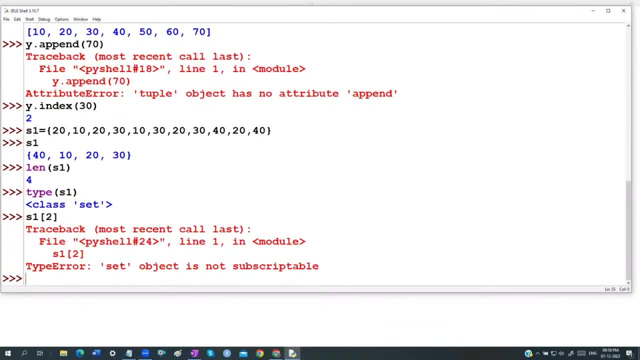 We cannot. Subscripting is also nothing, but we are getting. You know what is meaning of subscripting, actually guys. So getting some part of them, which is not possible. Even slicing is also not allowed, actually guys. 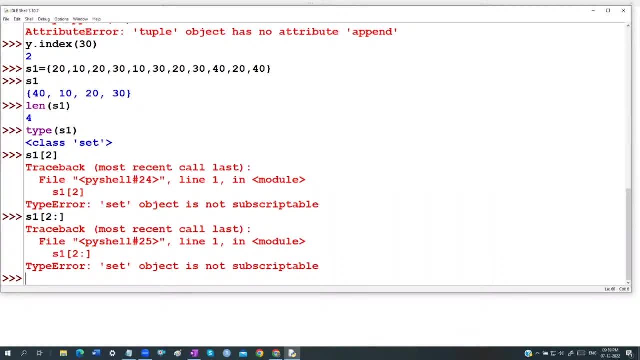 Slicing indexing is not allowed as of the set object Because the main reason is they are not following any particular order In a list. if I give some values, I know that I have given 10 at second index. If you ask second index, starting from second index, we can get it actually. 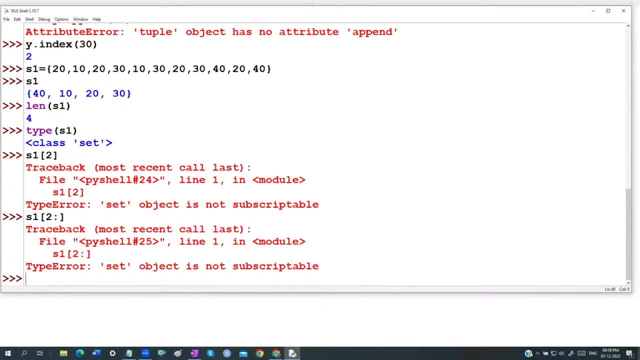 But here it is not. It is not maintaining any indexes at all and it does not maintain any order at all. So slicing, indexing is not allowed, actually, guys. Okay, Then what is the use of sets? there is no indexing or slicing. 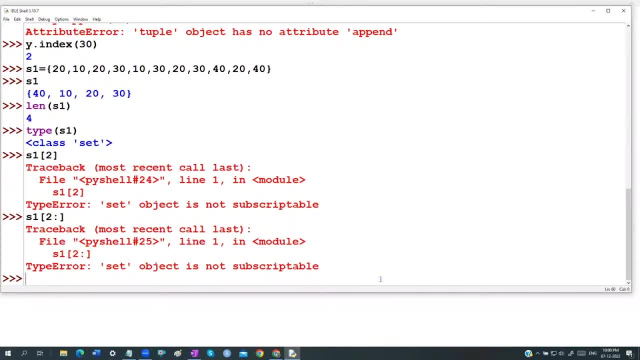 There is no indexing with C. No, no, no, No, no, no. It is not like that actually. Why do you require a set object, is I told you. I said also, I told you one point. These are going to be some of the. what we can say is: these are the basic things which we have to learn as part of the list. 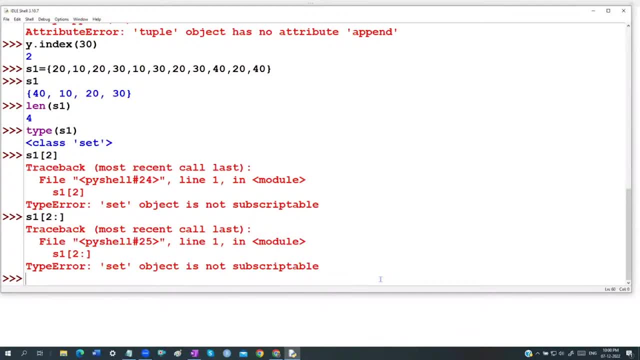 I am not saying that they are not used. I will tell you Like why, Why we are not going to use this and etc. Why do you use it? But just for the timing. let me explain that. So, as I told you that in Python the list tuple sets dictionaries. these are the basic data structures. 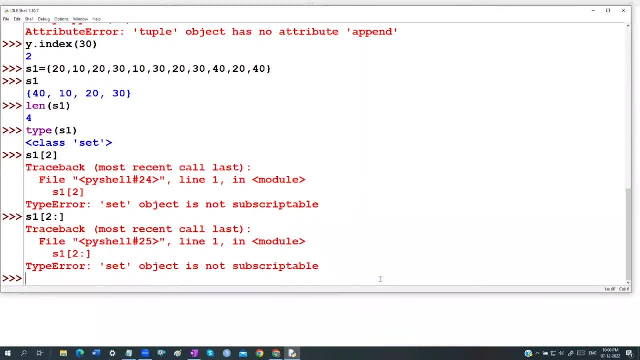 So that is the reason why you have to. if you are learning Python means at least some basics, we have to learn it actually. Why do you use it actually? Why do you use it means? I can explain that. 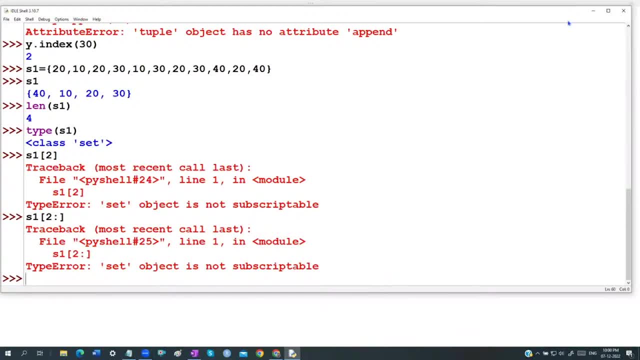 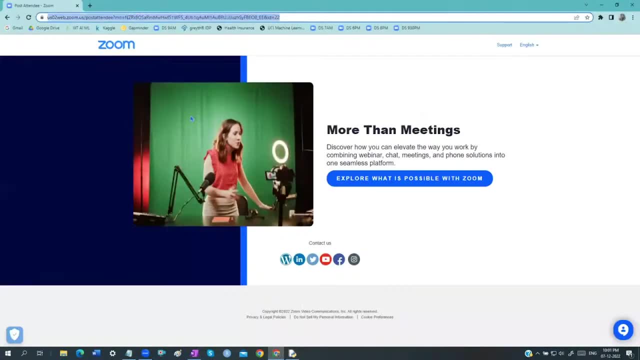 Like I can explain it, But the The things are like you may not understand the things actually, Just let me show you that application. actually Don't worry, Because being you have been asking for like why we are going to be using that. 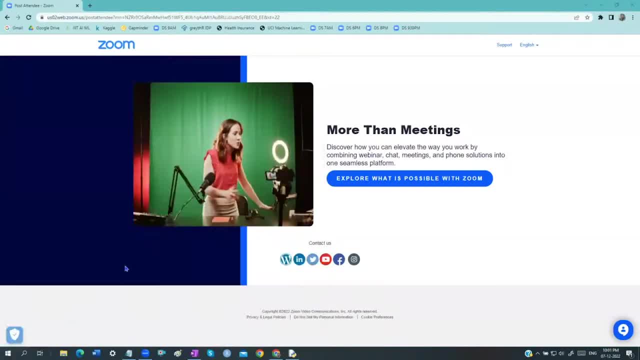 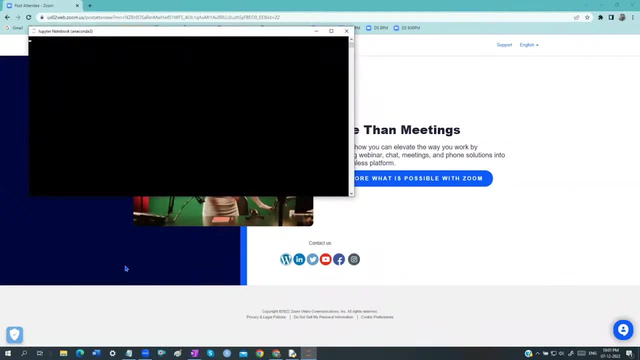 I will show you some practical application for that. I cannot explain the concept because you really don't know what is. I really don't know what I am explaining that. But I can just explain the things. Like, try to understand it a little bit carefully. 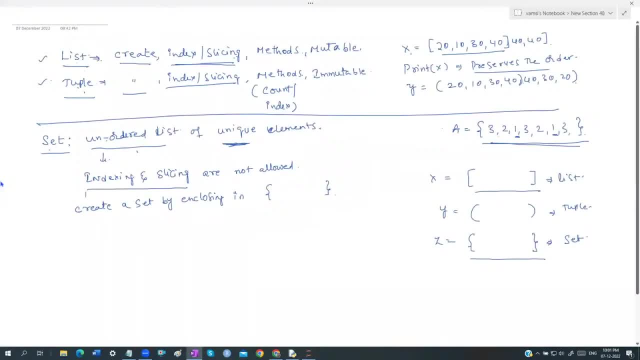 So let us say that basically, why do you require hearing? You know the set operations. no like we have the concept of intersection concept. we know that actually. So intersection can be applied only whenever it is a set object. 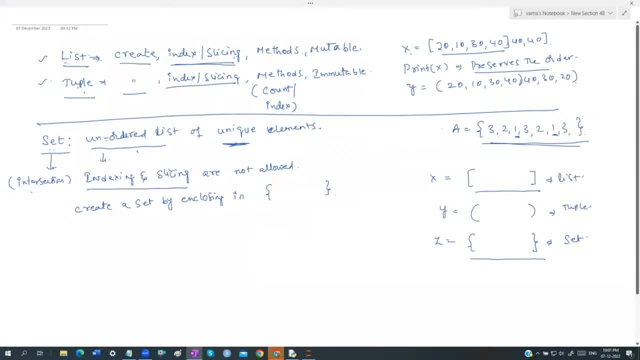 On list. we cannot say: I cannot find intersection between two lists, We cannot find the intersection between two tuples actually. Now just an example. I have some kind of an, I have some set of some values. are there some random numbers? are there actually? 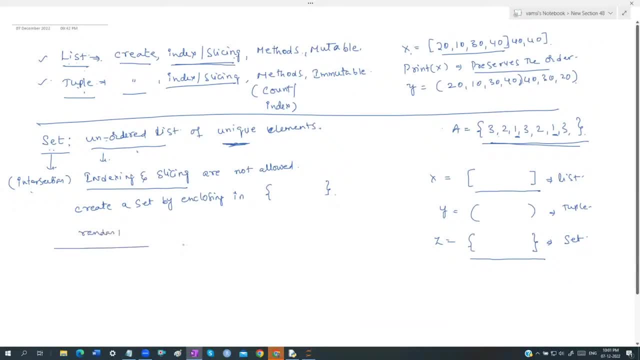 Just an example: Some- I'll take some random numbers, one actually, Some, it is having some values, like like some 20, let us say we have a 15,, we have a 25,, we have 11,, 16,, 18,, 17,, 43.. 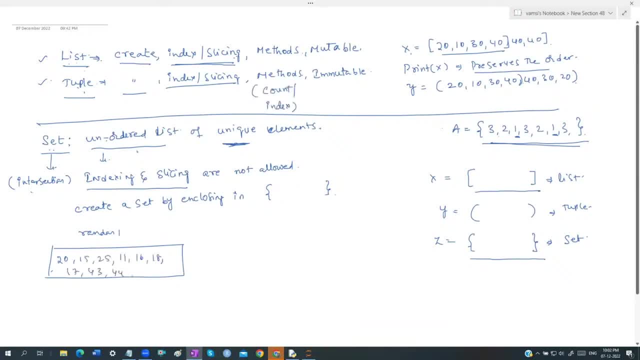 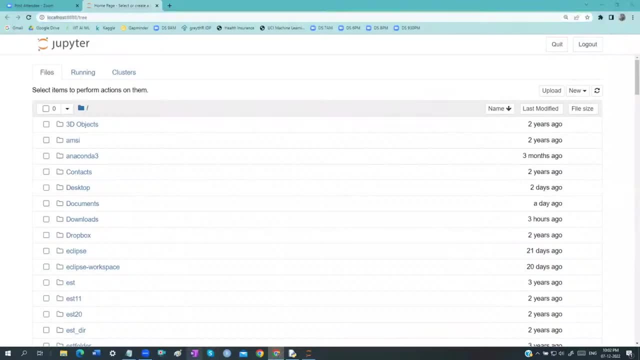 Some you may have also repeated numbers also does not matter. Let us say 44,. just a second, guys, Actually white is blinking. Let me just give a second. See, whenever the values are very small in numbers, we can easily identify that. 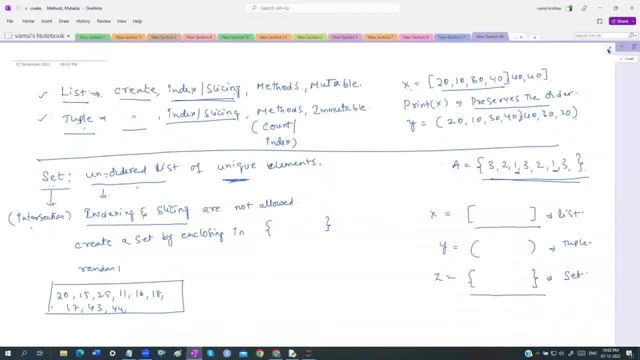 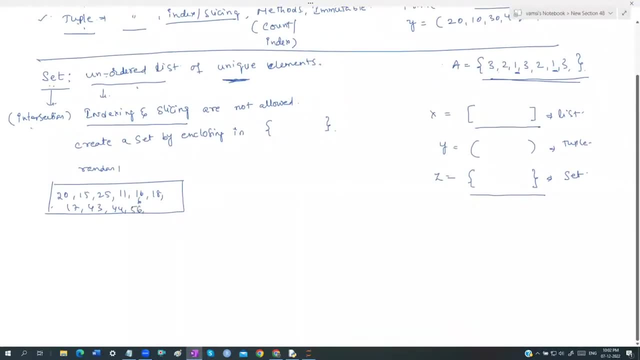 We can easily identify that, But whenever the numbers are very large in numbers we cannot do it. actually, guys Like something like 44 and some 56, and something like we have some 34,, 32,, something is the data. 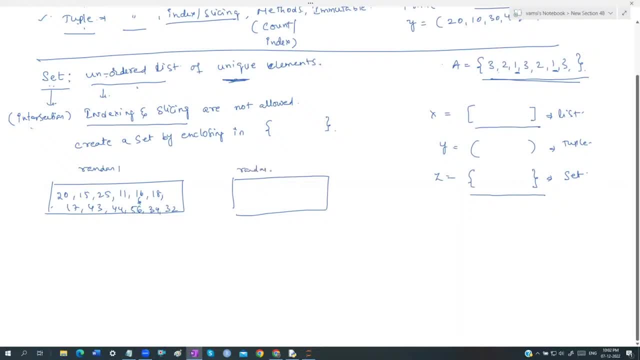 I have an another set of random numbers are there. I have an another set of random numbers are there, Like, for example, 17,, something like it, something like 20,, let us say 44,, let us say 57, and 35,. we have a 34.. 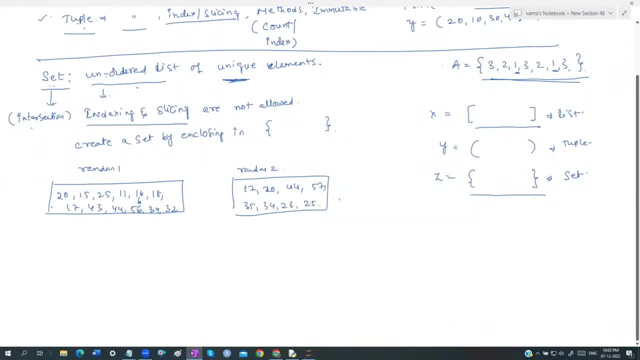 And we have 23,. we have a 25.. Some numbers are there actually Now. sometimes it may be required. That means, why do you use it Means? later I will tell you We do not have that many simple values actually. 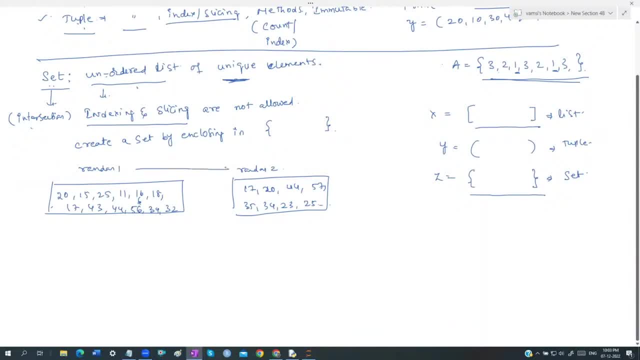 But I want to find out how many common values are there between these two random numbers. actually, Manually it is a little bit confusion. actually It is a time-taking process: 20 is there And maybe something like 34, I think. 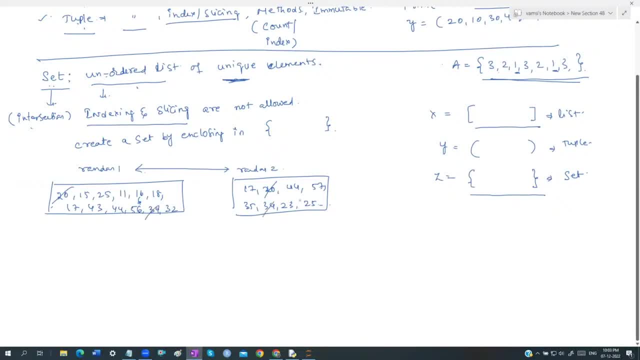 I have written 34.. 34 is going to be there, And even there may be 44 also, it is going to be there, Something like that. I want to find out some common values between them. So in that cases, we are going to convert these random numbers to one set object. 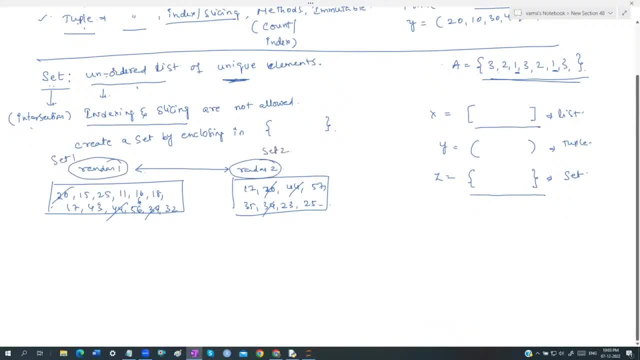 And I will convert this random 2 to another set object And then I will find out the intersection between them. But why do you use it? It means, when you go for machine learning applications, I will tell you that actually In machine learning concepts we will discuss it actually. 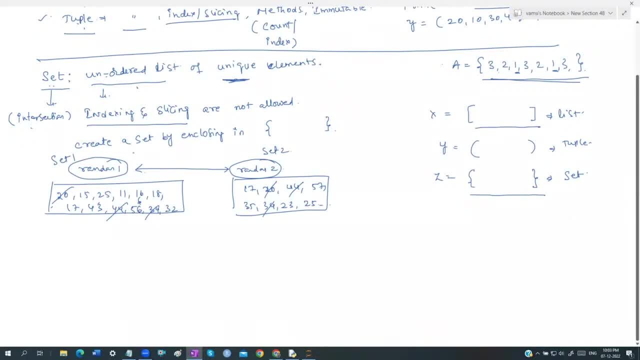 Because in machine learning, what we will do is we are going to do some kind of testing. We are going to do it actually. So this is going to be my test sample 1.. And this is going to be my test sample 2.. 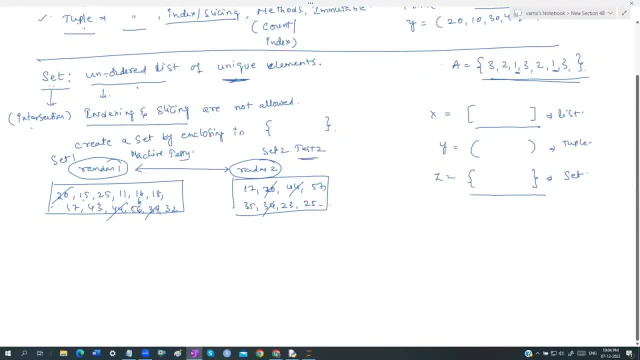 So in test sample 1, test sample 2, at least how many samples are getting repeated? 3 samples are getting repeated actually. Maybe out of 10 samples, 3 samples are repeated. That means 30 samples. 30% of the samples are getting repeated actually. 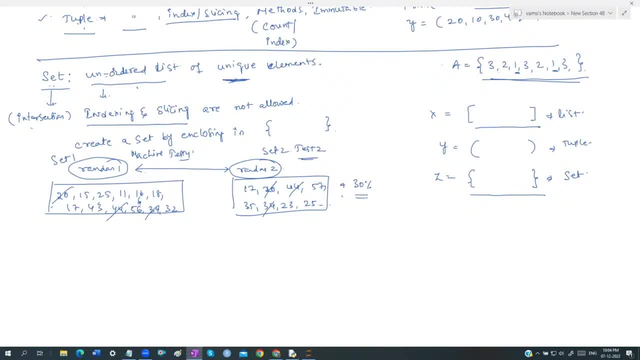 So to make you understand that I will use this set of objects, We are going to use it, But one or two times only Throughout your machine learning. one or two times only. we have to use it. But if you want to use it, you can. 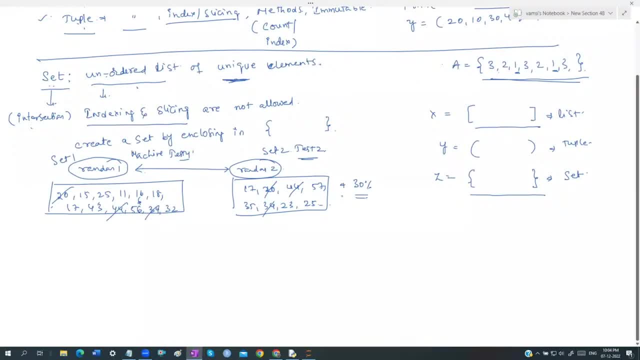 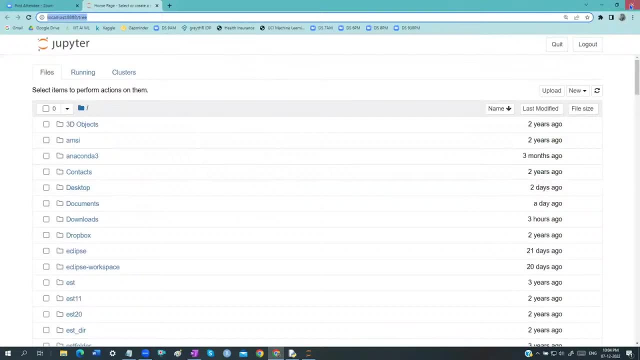 But if you want to use it for one time also, we have to know the concept. So that is the reason why we are discussing it. Right, Okay, Right guys, Okay. So later we will see them One or two times. we are going to use them. 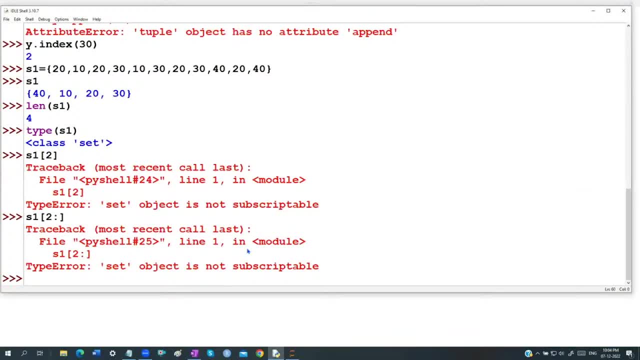 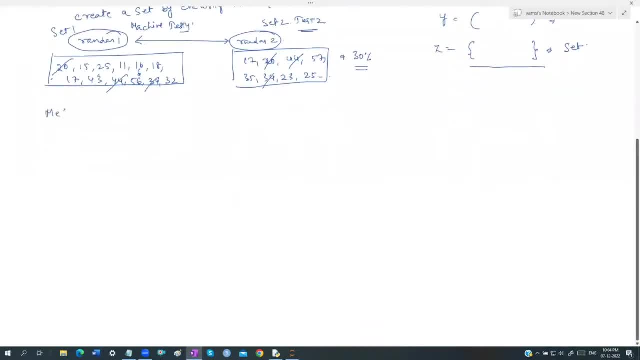 I will explain that, like where to use a set object actually. Okay, Now let us come to the methods actually. guys, Let us come to the methods First. I will tell you some methods which you can understand it easily. 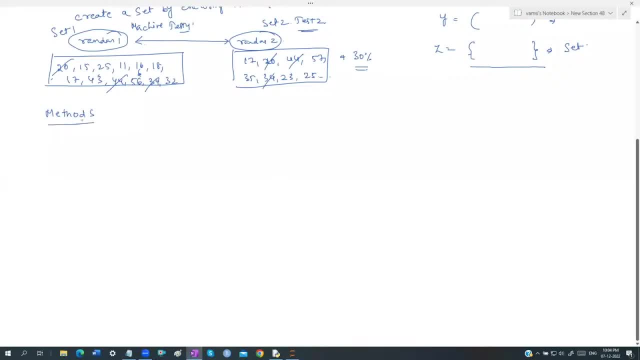 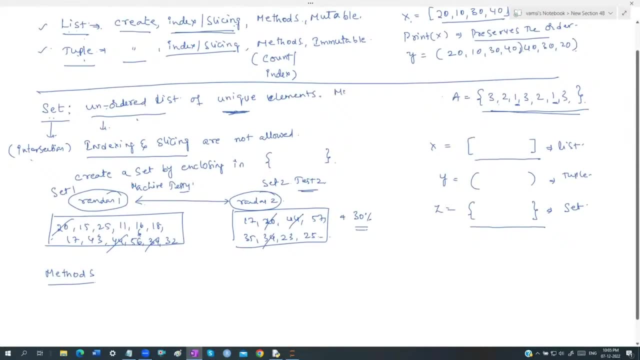 After that I will tell you some other methods which are different From the list. and the tuples, actually, guys. So one more thing: actually, guys, It is a mutable object. only Set is a mutable object. guys Means you can modify them. 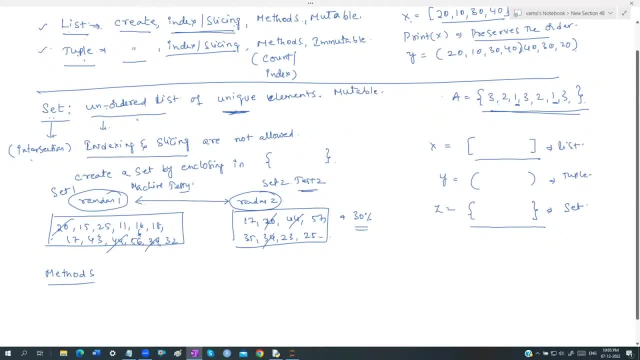 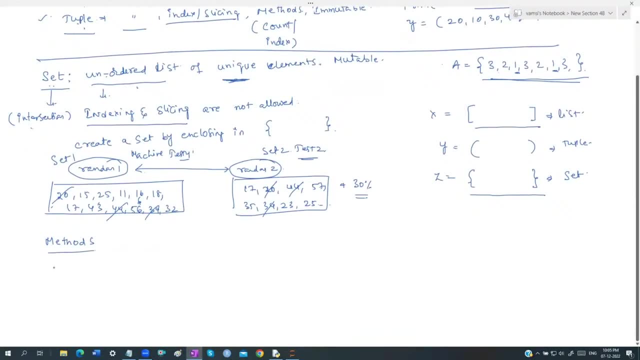 Modify them means you can add some elements, You can remove the elements, Whatever you want. we can do it actually, guys. First one, which is going to be nothing, but The method is going to be: how do you add the elements, actually, guys? 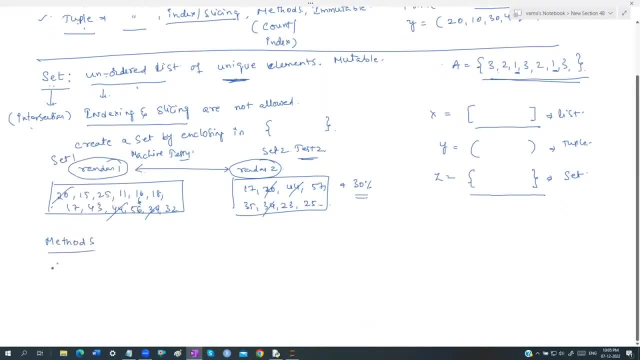 Normally in list we have append, we have an extend and we have something called as an increase. So in the list- we are sorry- in the sets we are having a method called as an add object. actually, guys. 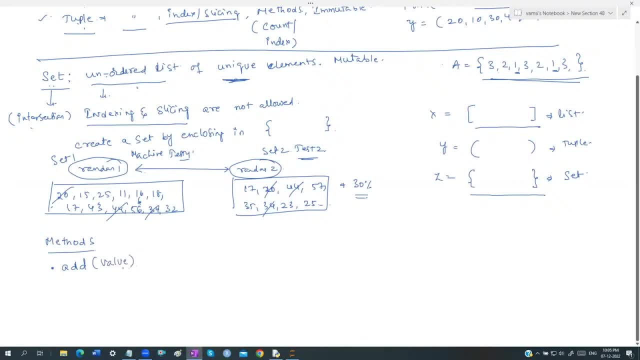 Add is a method And just give the value actually, guys. But where it will be generally, why it is not append, you may get a doubt. So why it is not append then? Why it is not append means generally, appending means it is at the end. 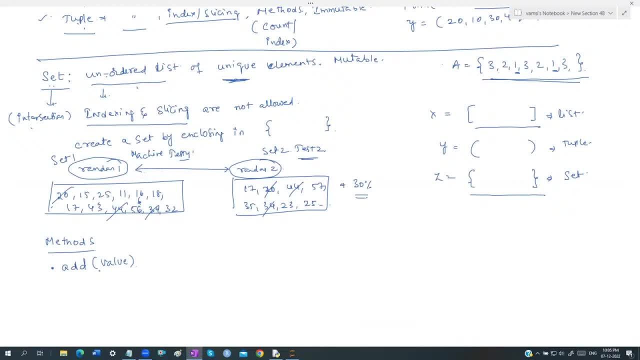 But here in set object, we can't say that it will be appended at the end. actually, guys, We can't say that it will be appended at the end. Actually, that's the reason we don't say that append and extend. 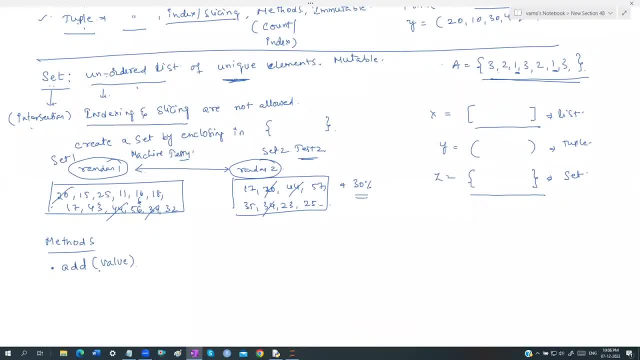 Even in insert. also, insert is based on the index concept. I want to insert before the second index, I want to insert before the sixth index, But here indexing does not work, actually, guys. So it is going to be add. 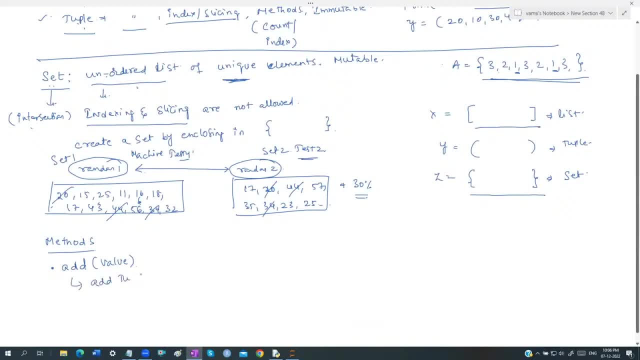 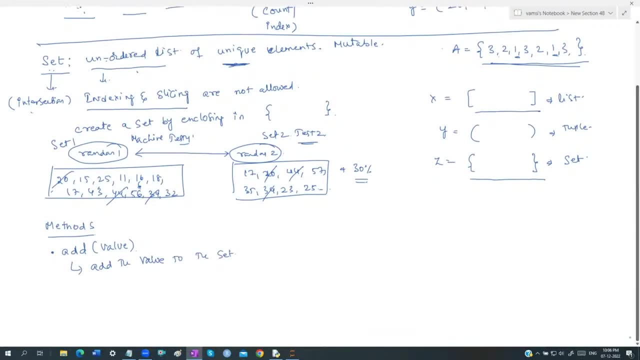 So what is add is going to do, actually, guys, It is going to add the value to the set, actually. But one small problem, actually, guys. If the value is already existing, simply it does not do. It does not do anything. 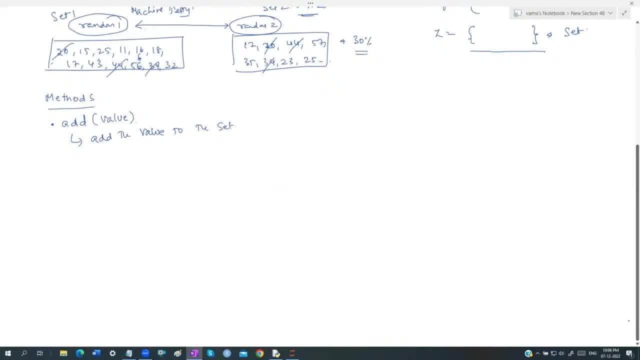 It does not raise any error. also, actually, guys, Because we know that the elements must be unique. If already 10 was there, if we try to add one more time- 10,, it does not throw any error saying that 10 was already there. 10 was already not there. 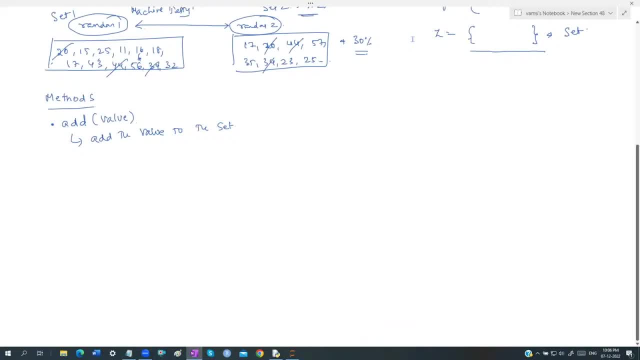 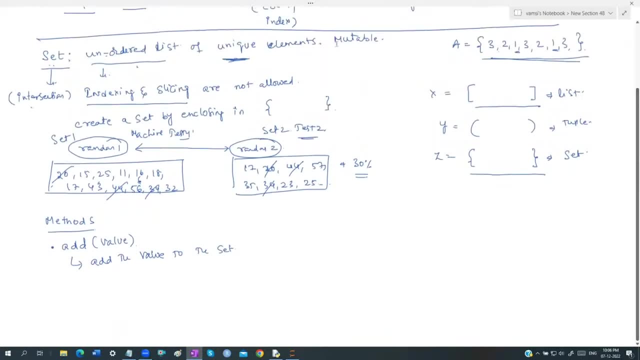 It does not raise any error. actually, guys, Sets are mutable. Yes, absolutely, Sets are mutable. Just now I told you the point. Just now I told you the point. actually, guys, They are going to be immutable objects. 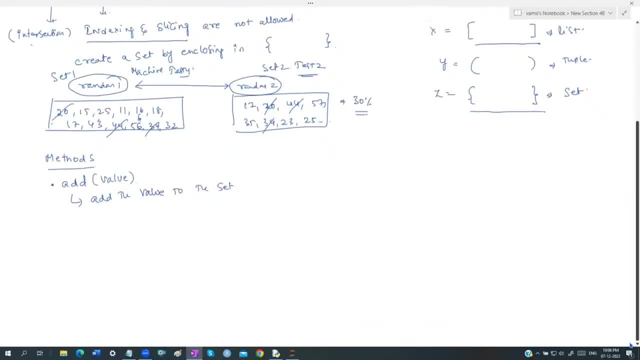 Sets are going to be mutable objects. actually, guys. Okay, Fine, Add the value to the set, But I cannot say that where it is going to be appended. actually, guys, And I think so. I need not to tell you about what is clear. actually, guys. 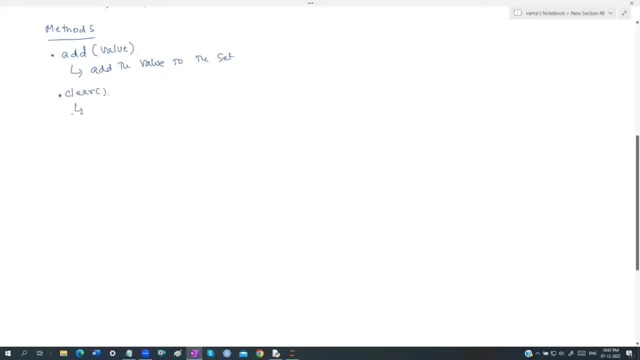 Same. Clear is going to be common, actually guys. Some methods are common, actually guys, But they will work with respect to that object only. It will work, actually Clear. You know what is a clear? actually guys. 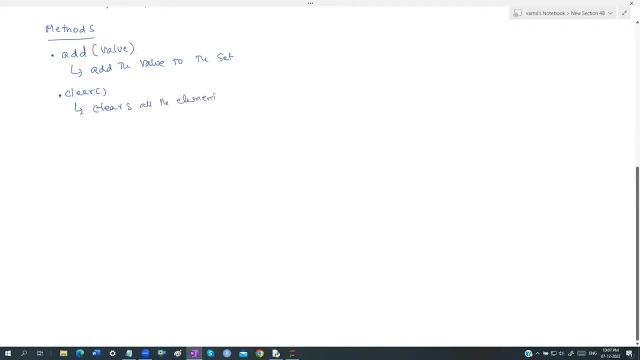 Clears all the elements from the set. All the elements from the set. it is going to remove actually guys, Same as it is. we are having some option called as a remove- actually guys. Think a little bit carefully, guys. 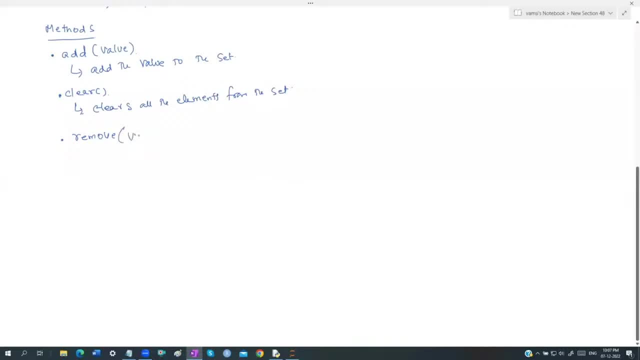 A remove is going to be based on value-based actually, guys, Right, It is going to be value-based actually. While I am discussing about the list, I told you what is a remove method is going to do, guys. In list object: same element may be there for multiple times. 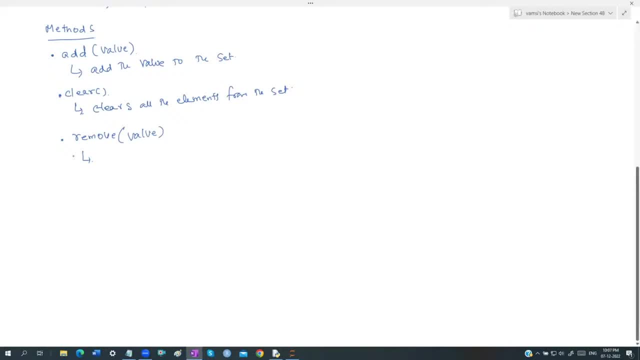 That's why it will remove only the first occurrence. But in set object it is only, It is only one time available. The value is not duplicated. It is going to be only unique values only. So I cannot say that first occurrence, second occurrence. 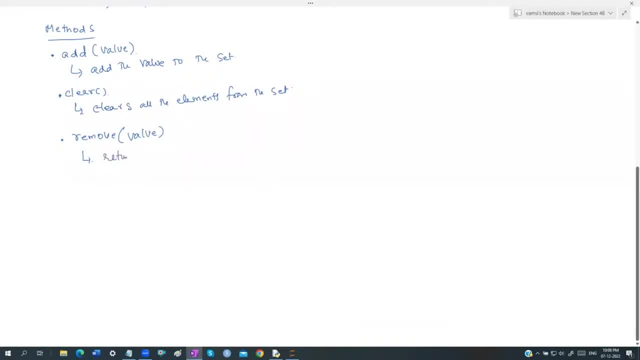 I cannot say this. actually, guys Remove- you know this. actually, guys Remove is going to. It does not return anything. guys Add won't return anything. Clear won't return anything. Remove also won't return anything, guys. 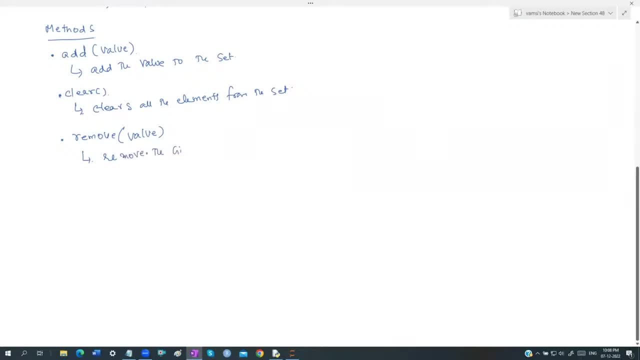 What it is going to do is remove the given values, or removes the given value from the list, Given value from the list, And we know this from the set, actually guys. But you know one point: This value must and should it must be there, actually guys. 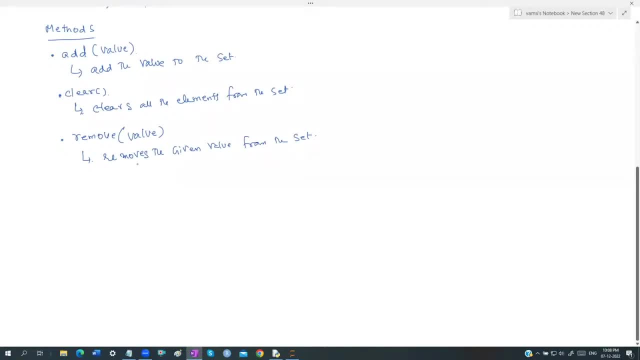 If the value is not there, it will raise as an error. actually, The value must and should it must be there If the value is not existing, If value does not exist Or if value is not in the list. If the value is not in the list, then it is going to be raised as an error, actually, guys. 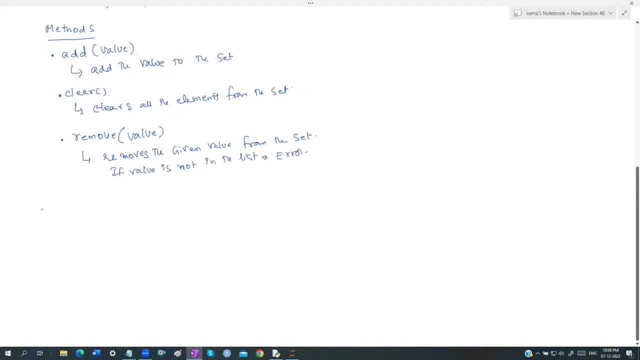 An error will be raised Here. there is one small method which is special. There is a speciality here, actually, guys. That is, we have a method, what we are going to call it as discard. It is going to be discard, actually, guys. 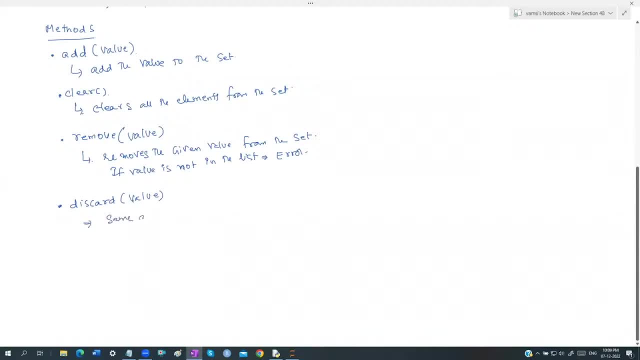 What is a discard is going to do is, guys, Discard is going to be nothing but same as a remove, actually, guys. But difference is if the value is not existing in the list. sorry, sorry, guys, Not in the list. 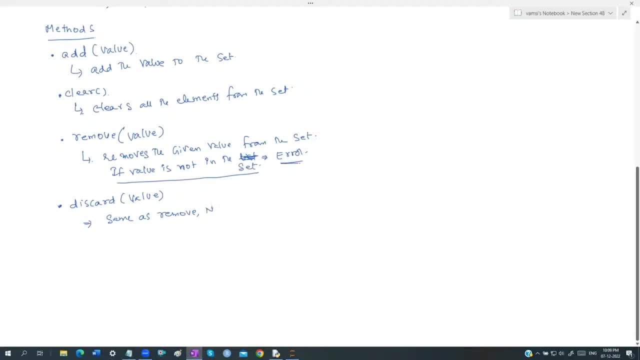 It is not in the set, It is going to be not an error. So it is going to be no error. If value is is not in the list or value is not present, that means it does not makes any noise at all. what is remove is going to do if remove value. if the value is there, it does not makes any noise. 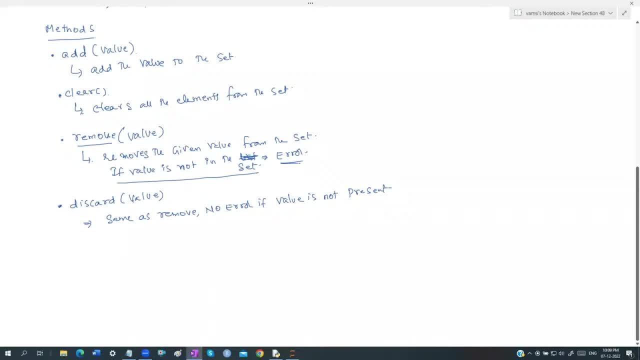 that means noise, mean generally i'm talking about that. it does not raise us any error, but whenever the value is not there, immediately it throws an error. actually, error is a noise in our normally. error is always a noise actually for us guys whenever we talk about a discard. discard says that. 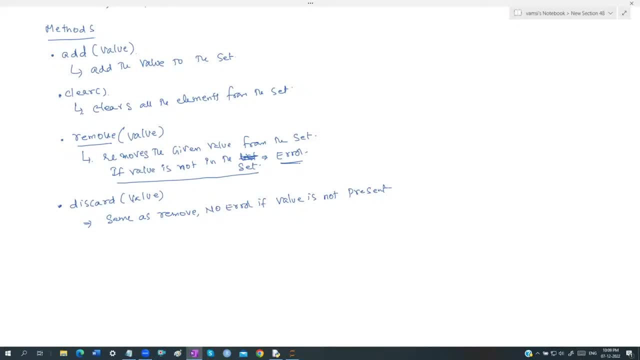 if the value is present, i will remove. if the value is not present, i don't do anything. actually, if the value is there, it will remove. if the value is not there, it does not lose anything. discard is not like this actually. so remove is not like that actually. if the value is present. 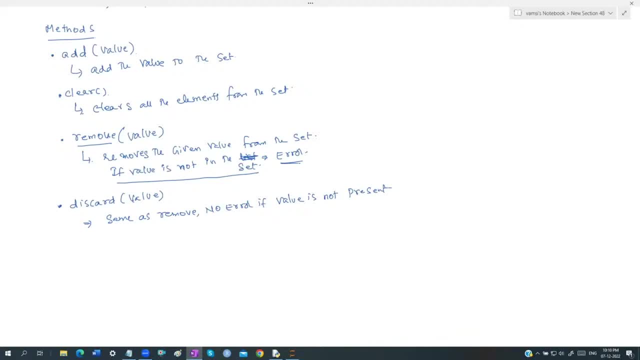 it will remove it. if the value is not present, it will raise us an exception. actually, yes, one error will come, actually yes. so similarly the same way, guys, but with the small, small changes. what we can do for adding only one add method, guys, but for removing, we have clear, we have remove, we have a discard, we have a pop also, actually, guys. 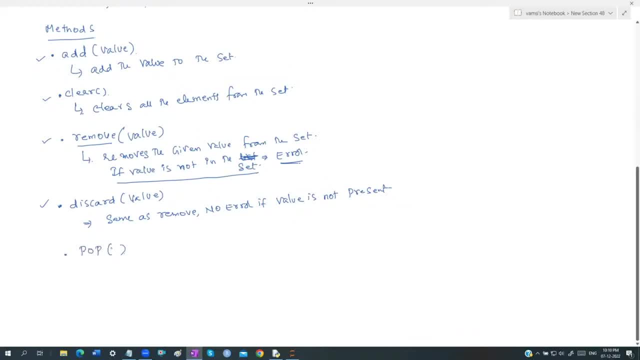 but pop does not takes any index, guys, pop does not takes any index because in set objects, we can't remove any based on the index. actually, because we cannot point to the index. actually, guys, what is pop is going to do is actually, guys, remove and return. you know this. actually, guys, it will remove as well as it will return. actually, guys, an arbitrary number. 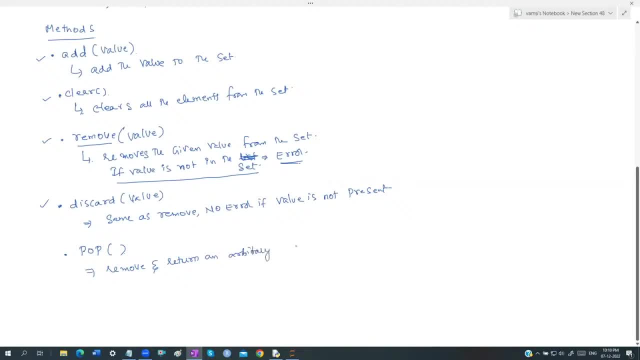 going to be arbitrary. actually, yes, it is going to be some arbitrary. so it is going to be something like: left to right, right to left, it is going to remove the values. so we don't say that that means it will all. normally, list will always remove only the last element minus one. but here it is not like. 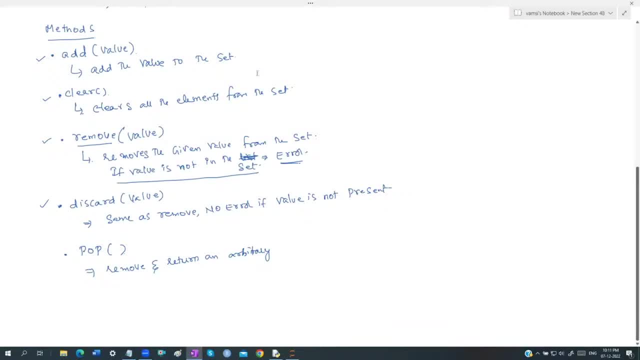 this actually, guys, from left to right. it will remove the elements, actually, so that that that kind of an exception, that kind of an application is what we are going to be using as of the pop method, actually, guys. so add, clear, remove, discard pop. these are the some of the common methods, guys. only pop is going to returns a value, actually, guys. 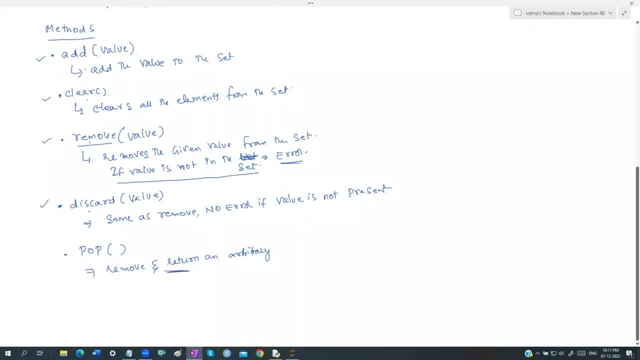 remaining. add won't return. clear won't return. remove note return discard won't return. even there is a copy method, is there actually, guys? but i'm not discussing about copy. i told you even in list also, i didn't discuss it- the copy in tuple, anyhow, we don't have a copy method, guys. 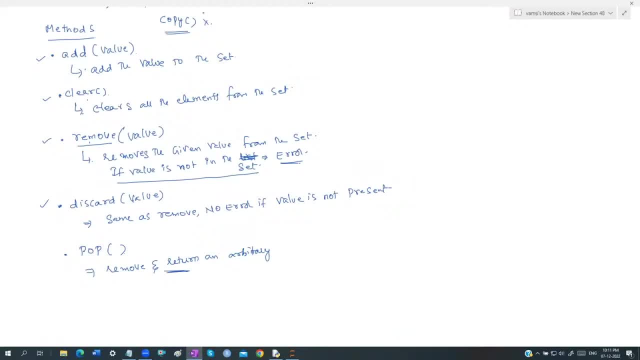 but in set objects also copy method. i'm not discussing almost all nothing. is there, guys, some concepts which you already studied? some concepts are? there are some architecture templates added. actually, these are going to be mathematical techniques. actually, guys, there are the mathematical techniques: add, clear, remove, discard, popness, these. 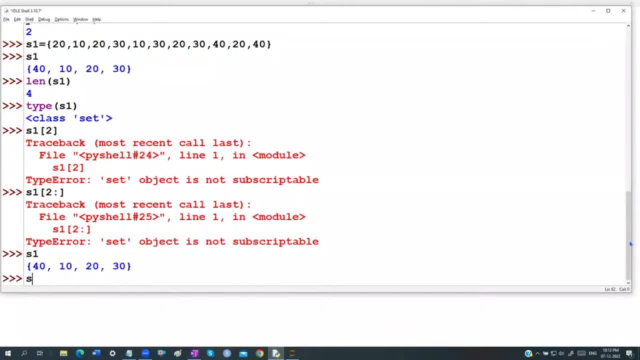 are the sum of the methods. first, let me finish off these guys and then we'll go to the next methods. actually, guys, these are your s1 action videos. i can say s1 dot, which is going to be the first method, itself is going to be nothing but guys, it is ad, actually, guys, it is ad actually. 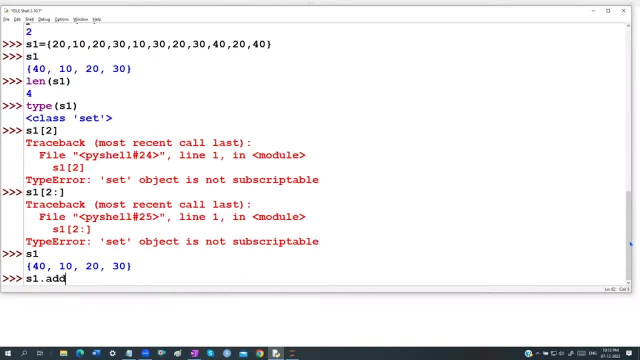 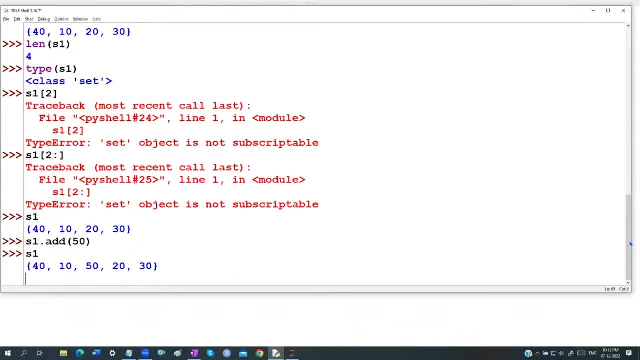 add of 15.. we cannot say that very clearly, guys. add an element to the list. see the document again. documentation: yes, add that. sorry, not. at least it is going to be set. actually, yes, generally in a flow we are getting it actually, but, sir, where it is added actually, yes, i can't say that 50 will be. 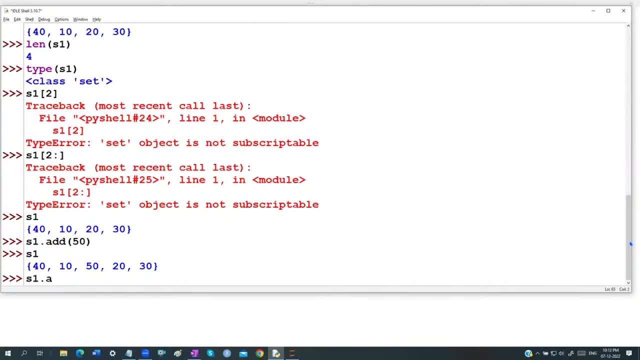 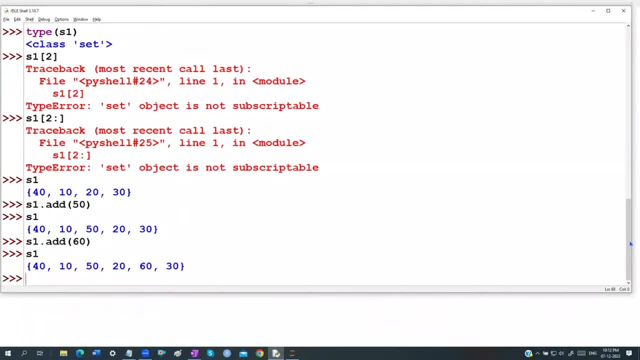 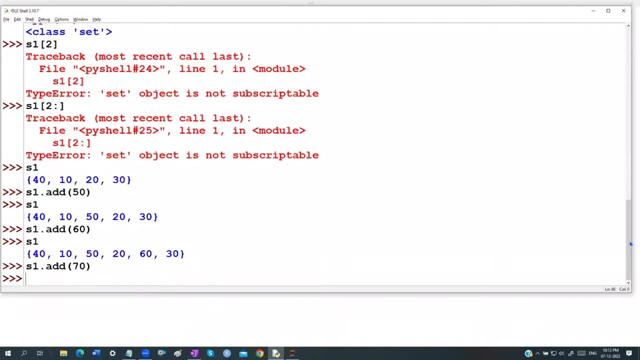 added only at the end. actually, yes, s1 dot, which is going to be add, of 60. yes, i cannot say that beside the 50, only the 60 is also going to be added. actually, yes, 60 is going to be added somewhere. actually, yes, s1 dot, it is again a add which is going to be nothing, but it's a 70 actually. 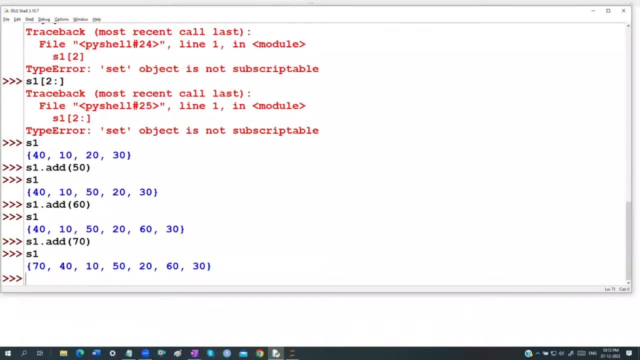 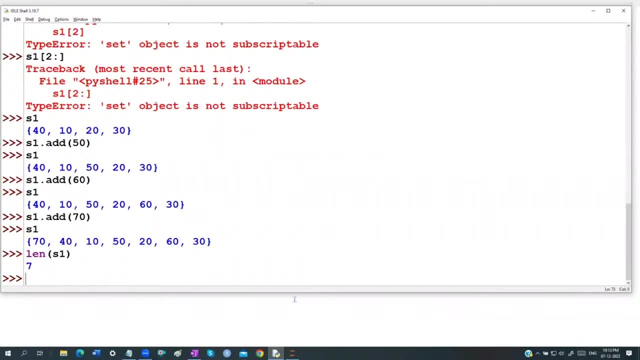 where it is going to be gets added. actually yes, 50 here, 60 here, 70 here. actually yes, what is the length of the s1? actually it is going to be. right now it is 7. that's it actually. yes, so we can add up the elements as you require if you want to clear. 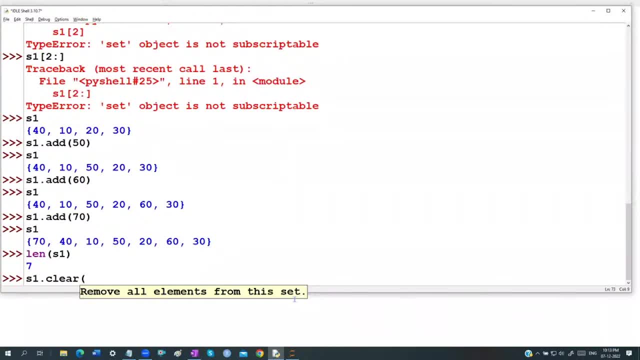 yes, you can, simply, you can, do the clear actually. you know what is clear actually. yes, remove all the elements from this set. i want to remove it actually. yes, i can say: remove actually, yes, what is going to be removed actually. yes, what is going to be removed actually. yes, i can say: remove actually, yes. 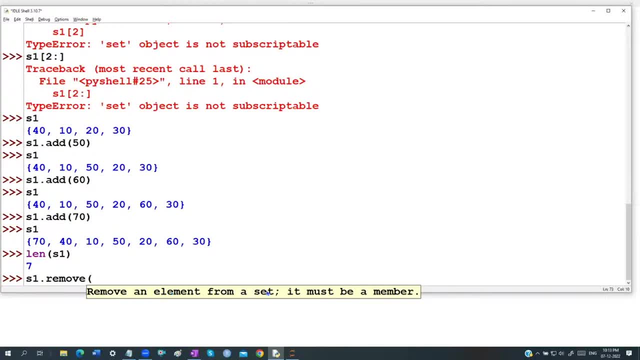 very clearly: remove an element from a set. it must be a member. it is clearly saying that it must be a member. you know what is meaning of it must be a member, must ensure it must be a member. actually, s1 dot. remove of 70. i can't say that. first occurrence, second occurrence. 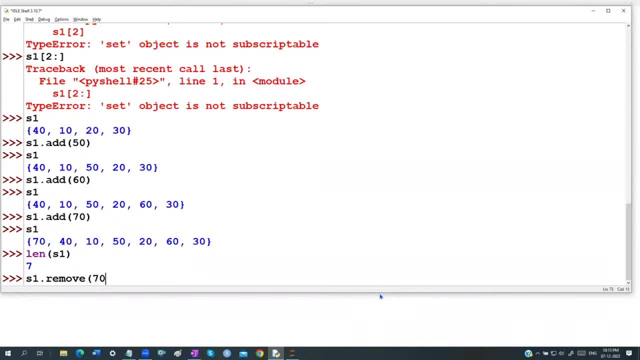 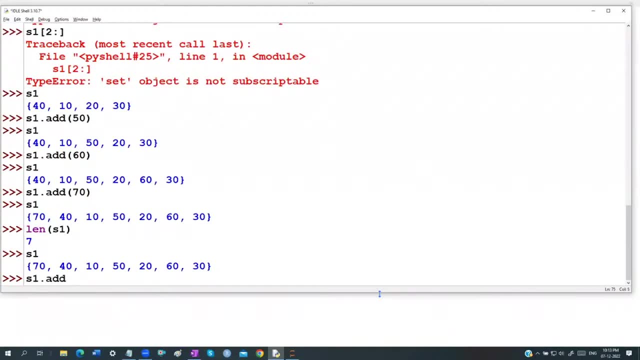 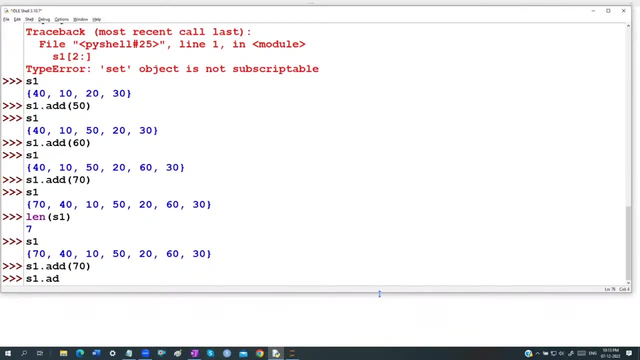 actually yes, why? because this 70 is available only for one time. okay, before going to that, i didn't execute it. 70 is already there. s1 dot which is going to be add of 70 one more time time. if i add up 70, nothing it will do, guys. it does not, so throws any error. also, how many? 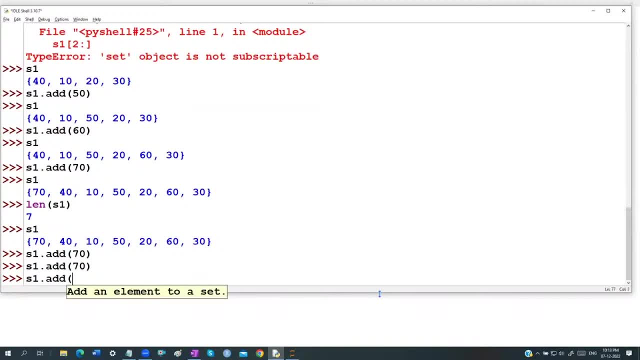 times you do it also. it does not throws any error at all. actually, yes, but don't think that it has been adding the 70 for multiple times. it is there only for one time only. it won't add it for multiple times. now i can say: s1 dot which is going to be remove off. 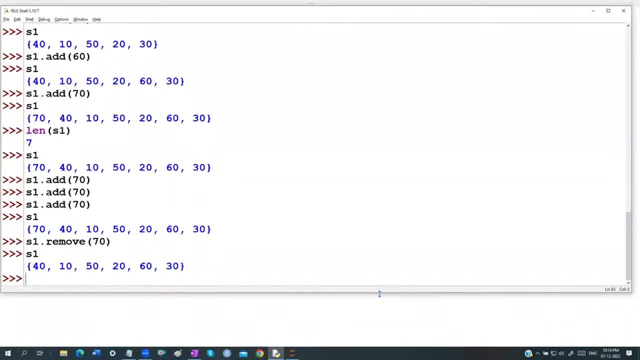 which is going to be 70. 70 was removed actually, guys, but it didn't return any value back whenever i set s1 dot, which is remove of again 70. this time 70 was not there, but removal makes a noise if the value is not there, it's a key error. so i can say that the key was not fought. 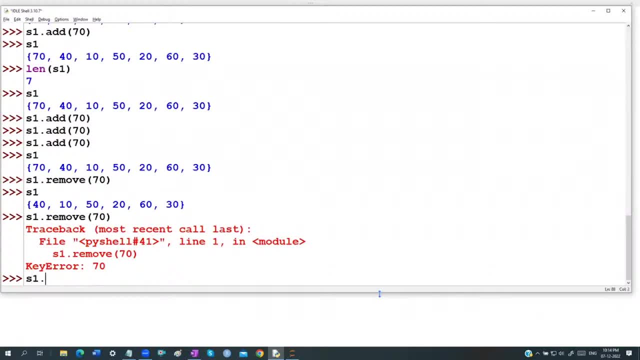 which is 70, actually guys. same example, if i said s1 dot, if i said discard, actually guys. see the different: actually guys. remove an element from a set if it is a member. it is not saying that it must be a member in the earlier case, when i said remove, it is saying: 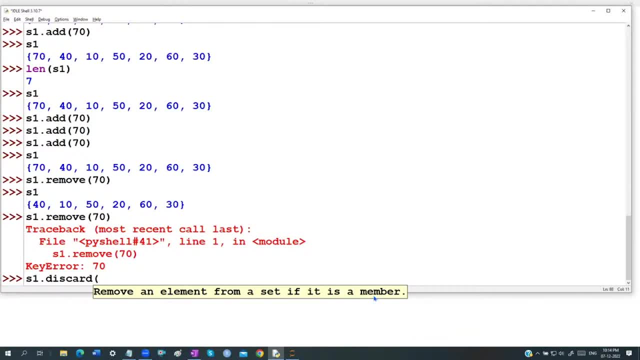 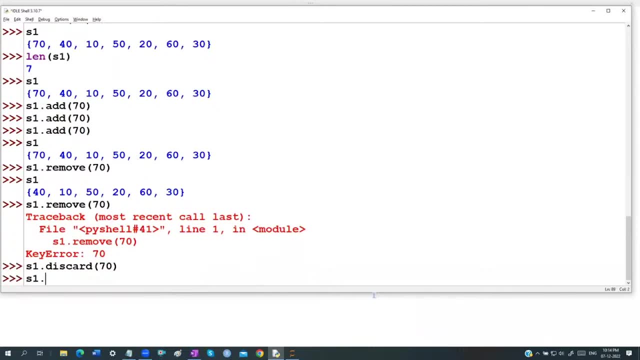 a member. but it is saying that if it is a member i will remove, if it is not a member, i don't do anything. actually, try to say 70 once again. guys, don't think that it has been got removed. it may be removed, it may not be removed. i said 40 actually, guys. 40 was removed again if i said: 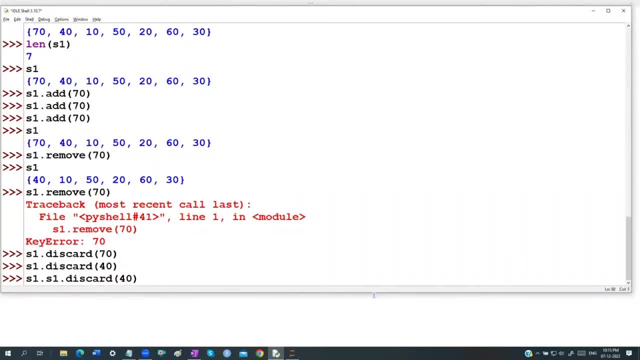 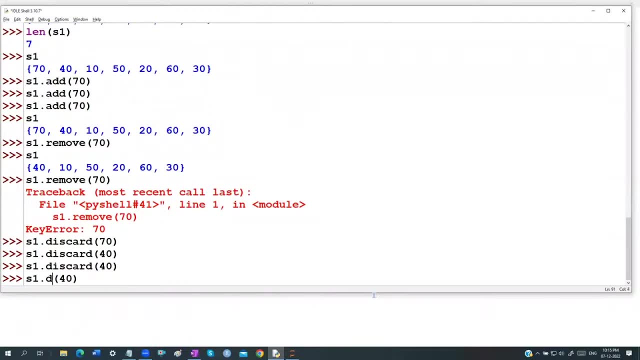 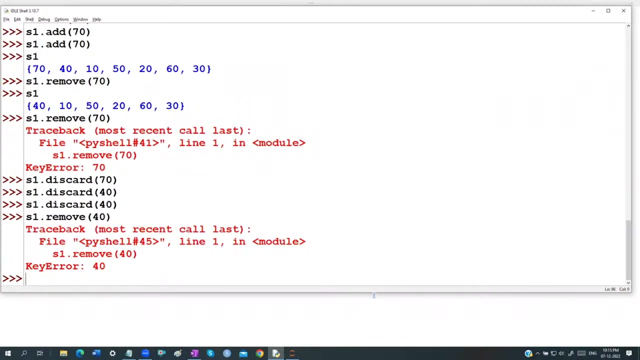 s1 dot, again discard of 40. it does not throws any error, actually it does not throws any error. but if you say, if i say yes, sorry guys, if i said s1 dot, remove 40, actually guys, 40 was already removed. we are getting an error, actually guys. so it must be a member. it it may be a member. 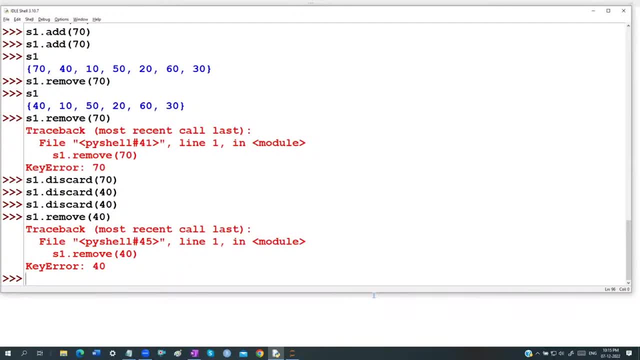 if it is there, i will remove. if it is not there, i am not going to do anything. actually, guys, this is going to be nothing, but this one, actually, and you know what is pop? actually, guys can observe carefully. guys removes and reduces, returns. an arbitrary set element raises a key error. if the set is empty, don't give any input. 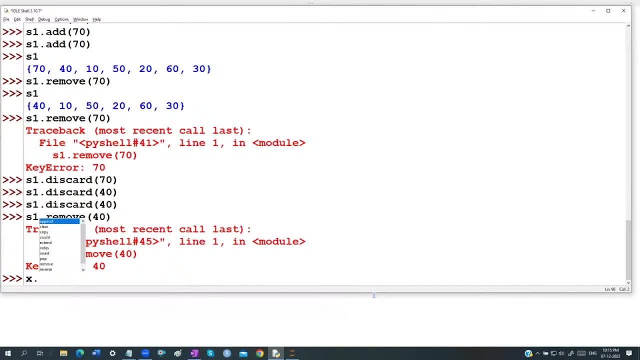 actually guys. we remembered when i said x dot, x is the list. actually, guys. if i said x dot, x is the list, actually, guys. if i said x dot, remove, you are getting a value. actually, even whenever i said which is going to be x dot, uh, what i'm talking about pop. actually, guys. if i don't give any value, 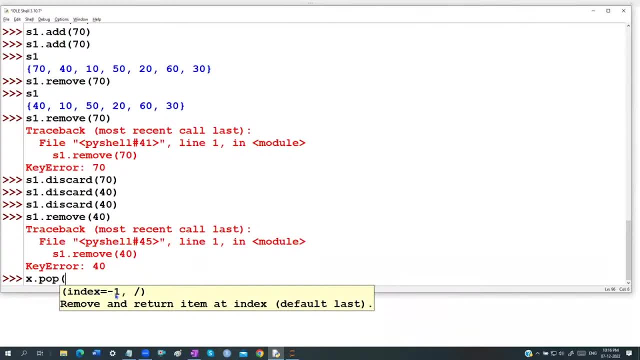 default value is going to be minus one, actually. yes, index will be minus one. that means if i don't give it, default is last element actually, guys. but here it is not like that. if i said s1 dot pop, it is not taking any arguments. guys, don't give any minus one, you will get an error. 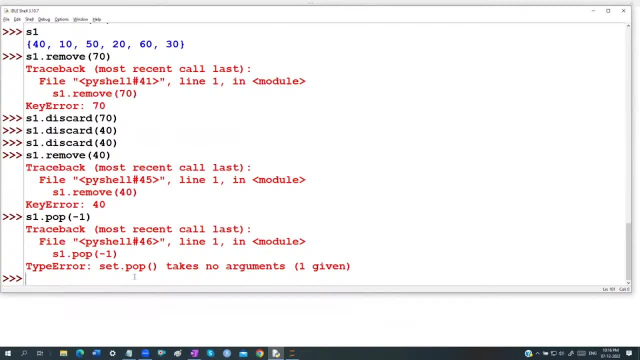 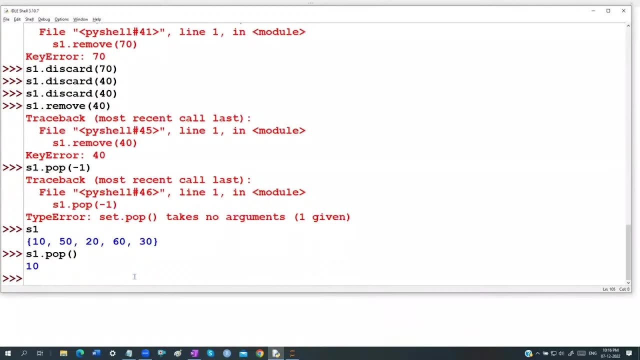 pop takes no arguments, one, but you have been given one. so it is an error, actually, guys, if i said x dot pop, actually guys. now you can see once, let me show you s1 here. now you say s1 dot pop, actually guys. so it is going to be removed basically from first element. that means from as 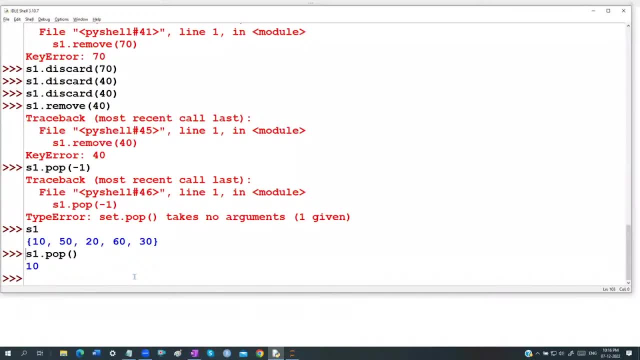 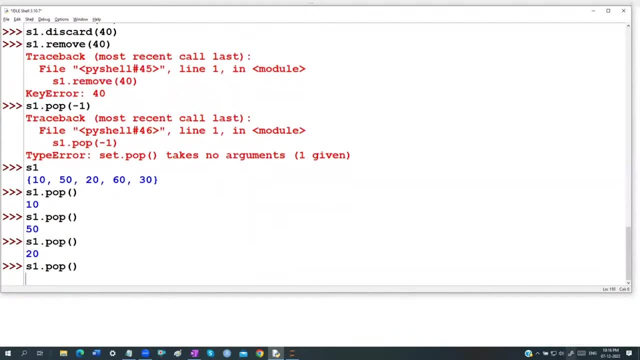 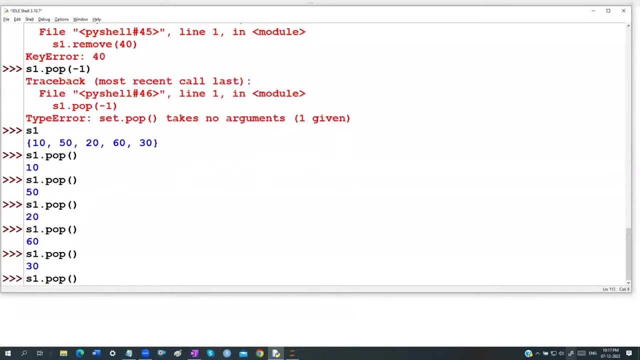 of now let's left to right again. s1 dot pop. you know pop will return some output. actually guys, 50 was removed and then 20 was removed, then 60 was removed and then it is going to be 30 was removed. actually, guys. now again, if we said s1 dot pop, it will throw an error because there are no. 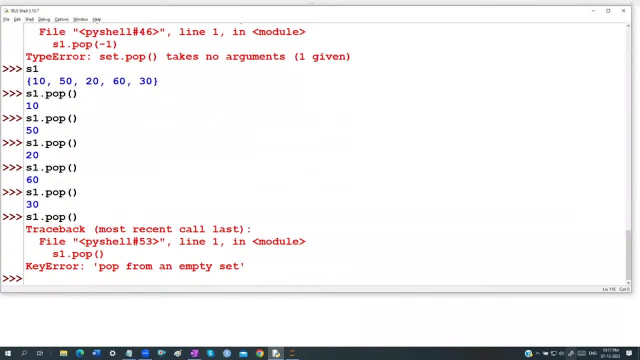 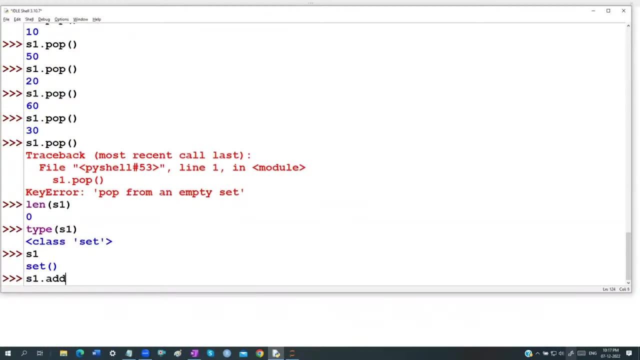 more elements from the list actually. so it is saying that pop from an empty list, actually s1. so what? you is the length of the s1 actually right now it is zero. actually, what is type of s1? there is no change, it is still, still a set. only this is your s1 actually. yes, again, if you want s1 dot, add at. 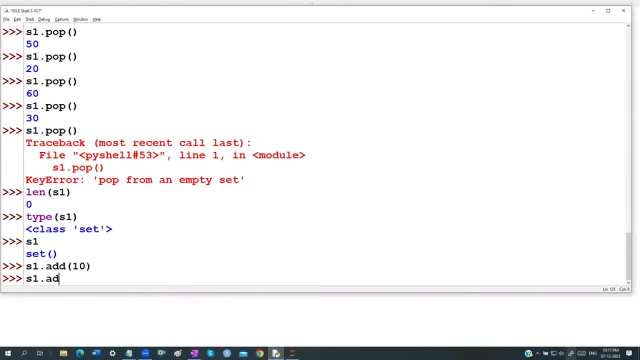 a time. you cannot add multiple elements guys. 10 s1 dot, which is add of 20, for list we can add up them, guys, but for set we can't add it actually s1 dot. 30 s1 dot, which is add off, which is going. 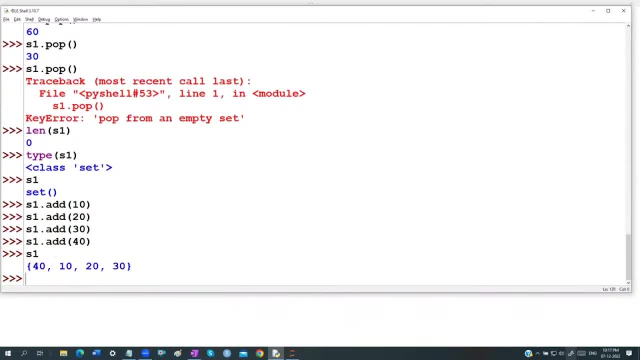 to be nothing, but it's a 40 actually. yes, so this is the data, what we can see with the data, guys. so these are the some of the methods which are basically, you know, sectional again, so remaining are different methods. it's very easy, very simple actually, guys. there are veryp. 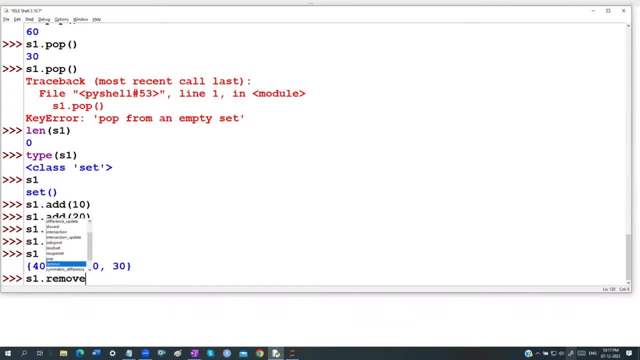 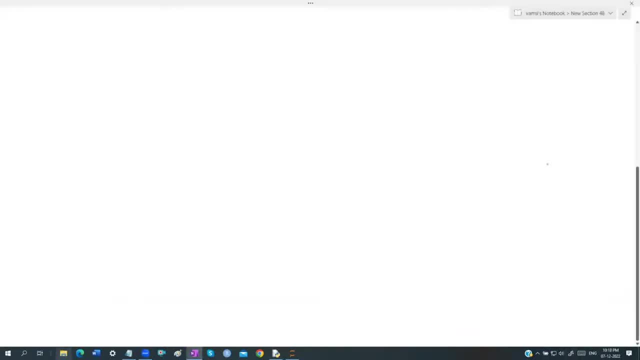 easy and very simple methods. actually, yes, okay. so once again i have been got discussed about half, i don't know insanely, as of now, discard. i told you, yes, discard, discard is. i told you, apart from that, pop. i told you remove. i told you actually, yes, remaining are different methods. it's very easy. 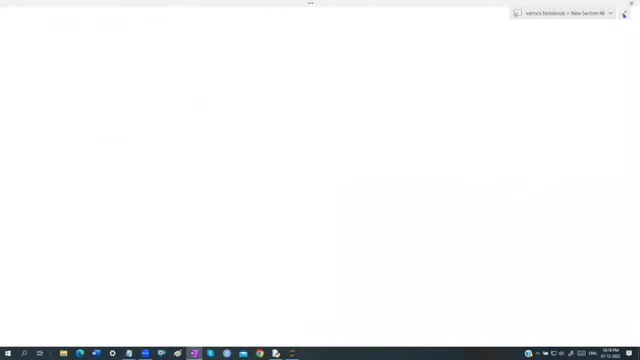 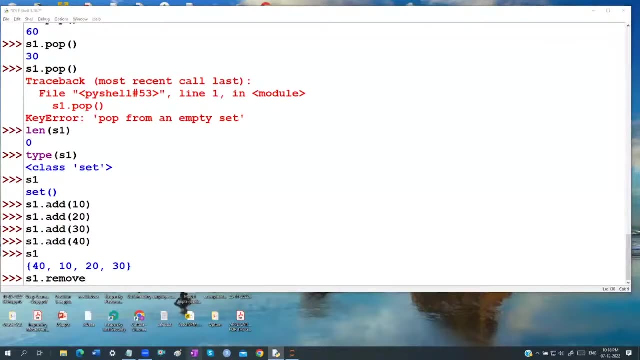 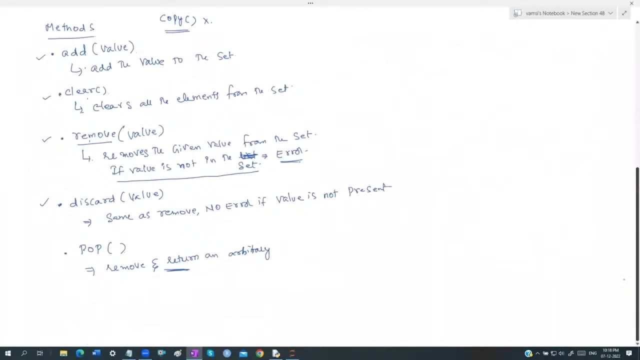 very simple actually, yes, there are very easy and very simple methods. actually, there's okay. so, once associated with the list- sorry, the methods associated with the set objects- i have been got discussed about that just a second. yeah, so these are the methods, what we have it actually. yes, these are common things. 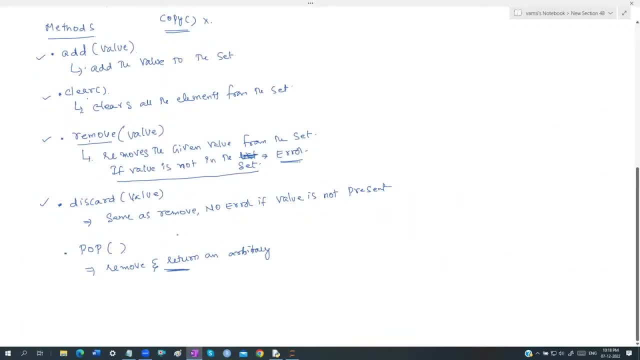 add, clear, remove, discard, pop. these are common methods, actually, guys. now the methods which are special, which are going to be speciality, in the list set actually, yes, you can't see the methods in any other. that means you don't find it in any other objects. we cannot find it, actually, guys. 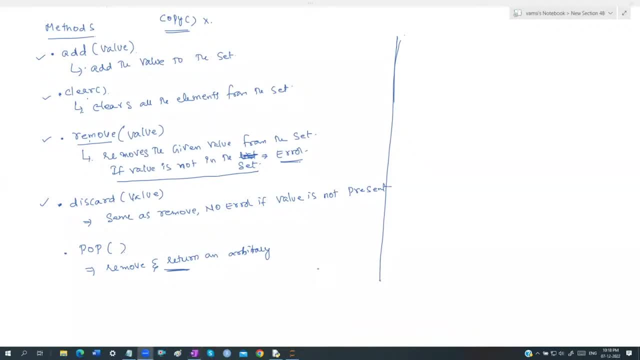 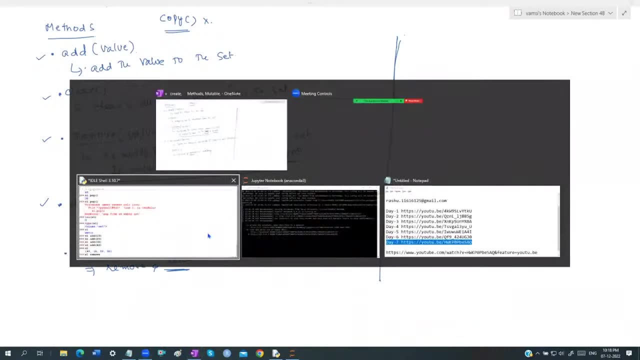 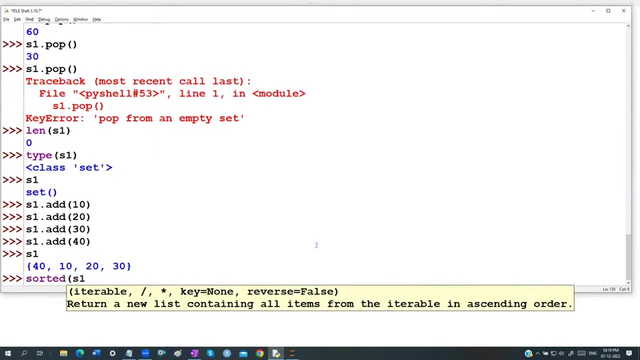 what are those? what are going to be those objects actually? yes, um, here, ascending, okay, actually, ascending, descending orders generally. we have a method, is there actually? yes, that means we have a function, is there not ascending, descending? it is going to be nothing, but it is going to be. 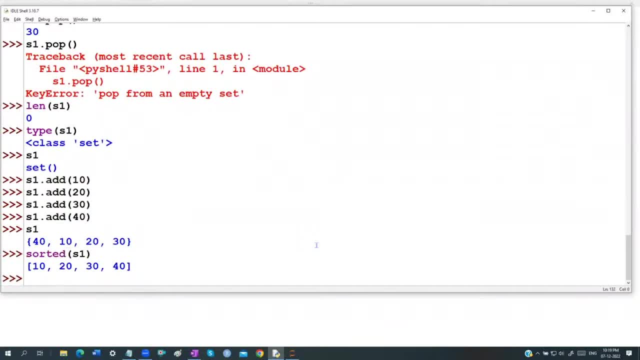 the, the, the S1, what we can see with the data, there is a method is there is a function, is there actually sorted of S1, you can see sorted can be used on list to pull sets anywhere you can use it. actually it is working. but see the output, what we can observe carefully guys. 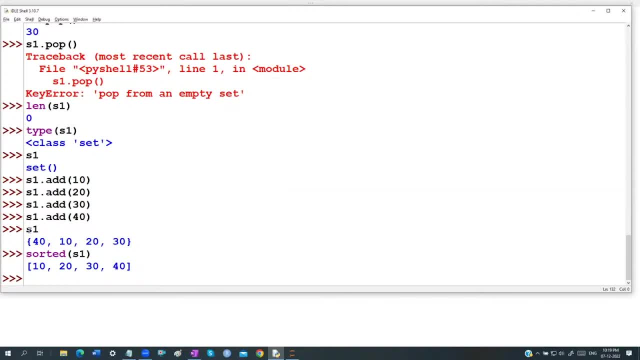 you see the output, what we can see, it actually guess S1 i have given as an input, as a set. but sorry, as i said, but outcome is coming like n, which is going to be nothing, but it's a list object. it is coming actually. so this is going to be sorted actually. yes, 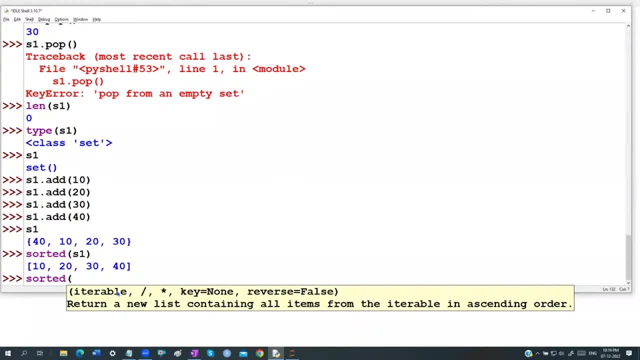 um, one point. i didn't discuss any guys what is iterable? i have been not a discuss, but see the output actually. yes, returns a new list. that means the set is getting converted into list containing all the element from the interval in an ascending object it is going to be returning. 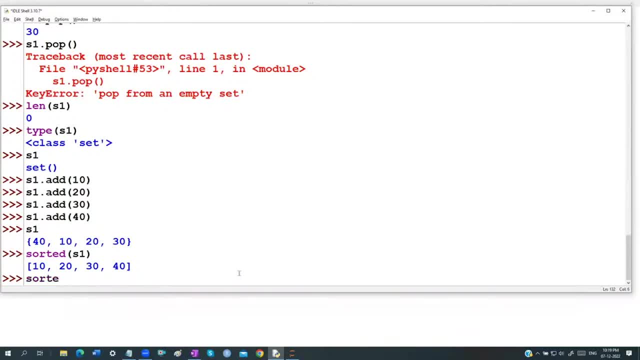 actually, we can do it, but it is no more a set. it is going to be converting into it, converting into list. sir, can i convert again into set? absolutely, you can convert it actually. yes, okay, we'll see. we'll see the application how to do that. we'll see that. we'll see that application. how to do that. 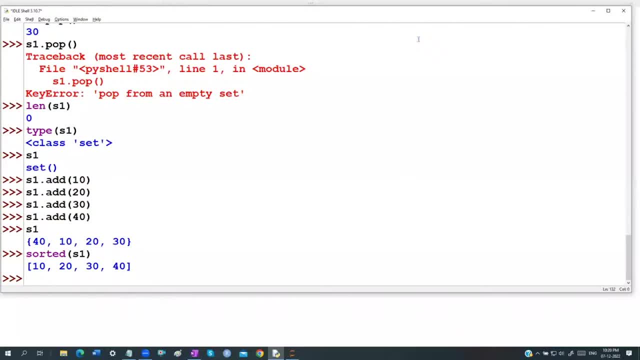 how to convert a set into text, uh, set into list, list into set. how to convert them, we'll see the applications. okay, fine, guys. okay, and i forgot to share set the option, actually guess, to everyone. so, guys, if you have any doubts, please, uh, when you're posting, when you're testing anything, 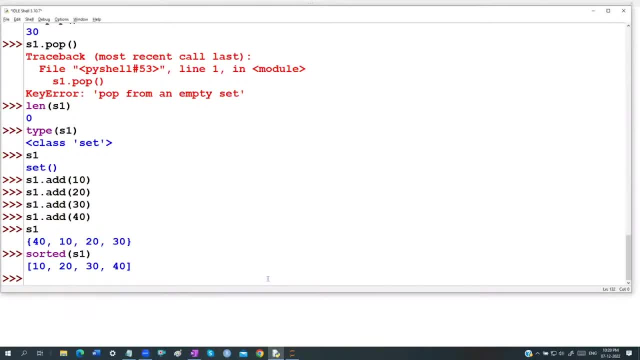 please send it to everyone, guys, so that everybody can see what, what i'm discussing about. that, right, guys? so this is going to be about, uh, this is going to be about the basic methods. actually, guys, now, the methods i am going to be discussing, they are going to be completely, they are going to be. 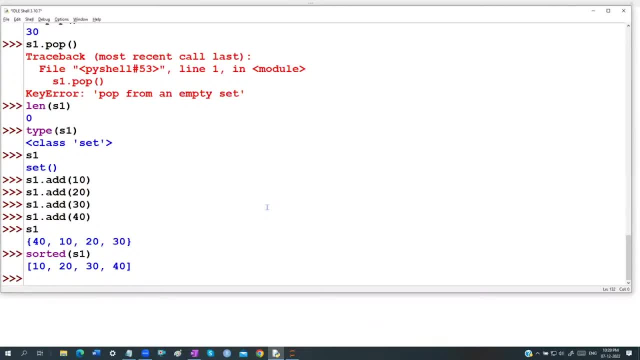 completely. which is going to be special for the set objects? actually, yes, it is going to be nothing, but a kind of an, a speciality, a special functionalities for your set objects. actually, yes, which is nothing, but we do it in our mathematics. no, guess it is going to be nothing. 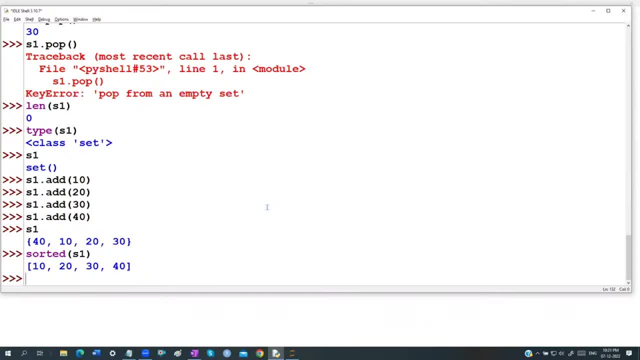 but in mathematics we know that actually set objects, uh, sets, we are going to be gets talking about that. so what our going to be that kind of an options? actually guess one of the common methods? common methods are going to be nothing. but let us imagine that there are two sets. are there actually guess s1 and 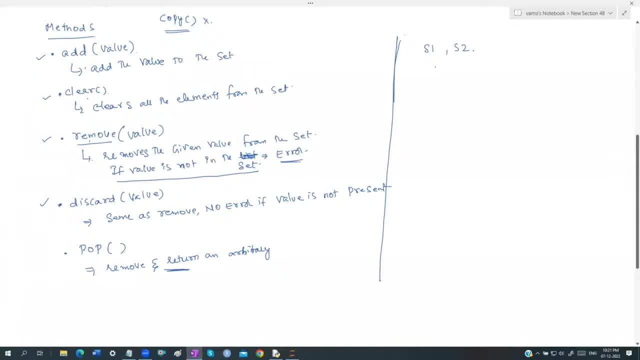 s2. i want to find the intersection. you know what is going to be intersection between the two values? actually guess it is s1. how do you do it? actually guess s1 dot. it is intersection of s2. so we know what is meaning of intersection between two elements. actually guess s1 dot. intersection with. 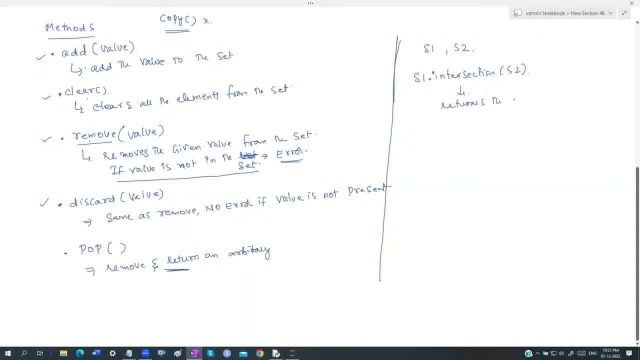 it is going to returns. we know this actually. yes, it is going to returns the common elements. actually. what are the elements which are commonly available in s1, dot, s2, s1 and sqt is going to returns and hope you remembered. it is union actually. yes, union of s2. actually. same technique. 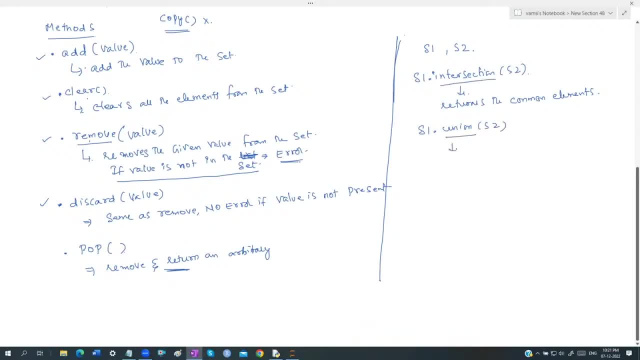 says intersection and it is union class. you know what is going to be. union is going to return section. i guess it is going to be returns the elements of both, elements from both s1 and the s2. actually it is not common values, actually, guess. i'll show you some examples what i can show. 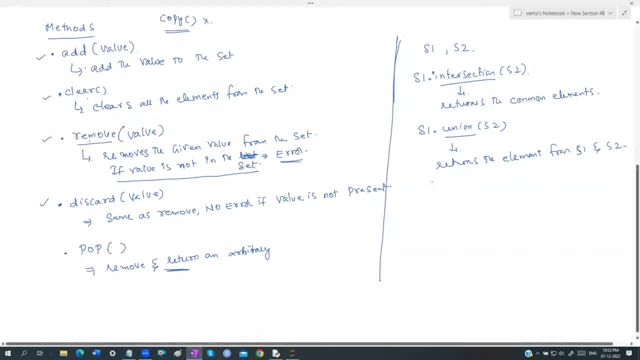 you actually and what exactly we are having. if you remember, minus, actually, guess we will call it as minus. in mathematics, you call it as minus. here, we are going to call it as an a difference. actually, yes, it's what we are going to call it as a difference, actually, guess you know what is. 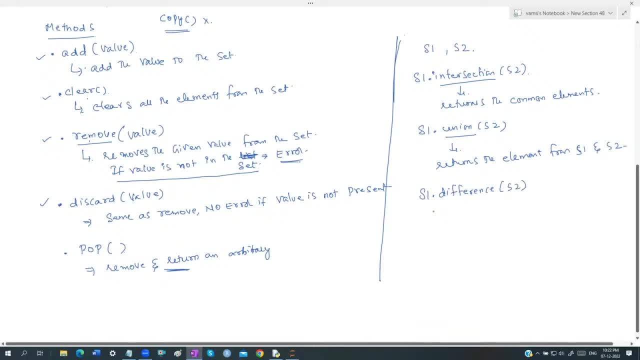 a difference. after removing the s2 element from s1, whatever that is left over those values are going to be gets coming. i'll show you once. have a look at this one, for example. s1 is having some elements like: let us say this: guys, i'm writing in a sequential order, but internally, what order it? 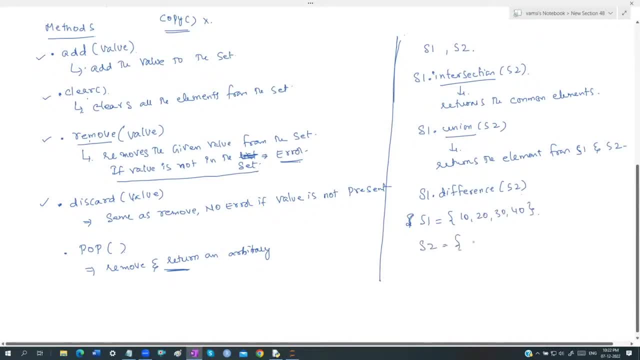 will take, it does not matter. with that, s2 is equals to nothing. but we have some values like 10, 20, 30, 50 actually. yes, just an example, s1 is having 10, 20, 30, 40, whereas s2 is going to be having 10, 20, 30, 50. we have it actually, guys. 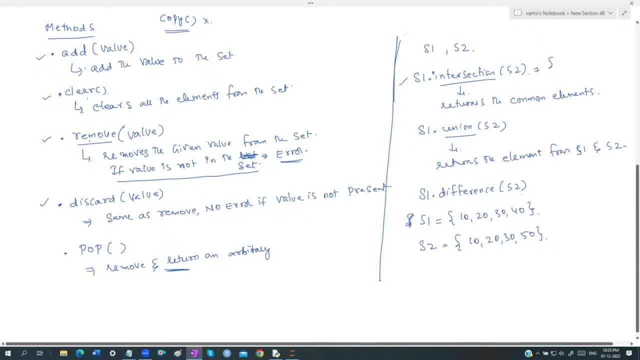 if i do s1, intersection s2, the result is going to be nothing but the common elements. actually guess, order may not be the same. actually, guys, i can't say that same order will come, union, we know it. actually, guys, it is going to be 10, 20, 30, 40, 50 will come actually. 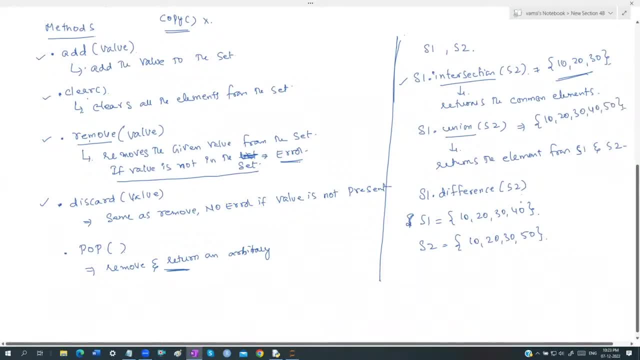 but we know this, guys: what is s1 difference, s2, s2 difference, s1? if i, if i say s1 minus s2, it is 20, 20, 30, sorry, 10, 20, 30 is eliminated. if i said s1 difference, s2. 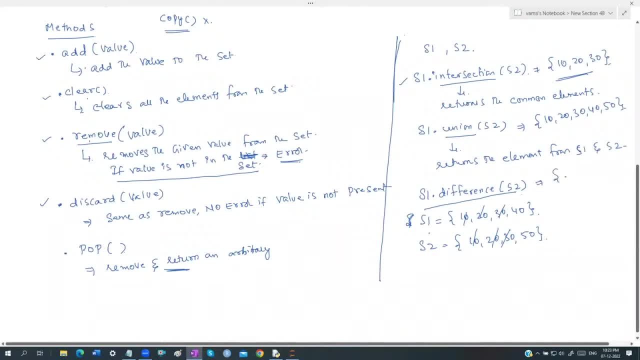 the result is going to be nothing but what is left over in s1, which is going to be nothing but 40, actually, guys. but whenever i said s2, difference of which is going to be s1, then the result is going to be nothing but what is left over in s2 after removing the element from the s1, then the 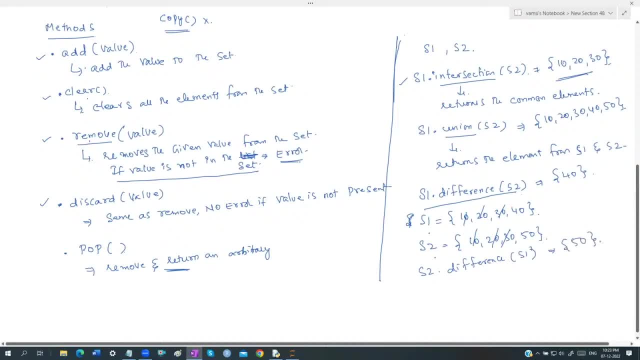 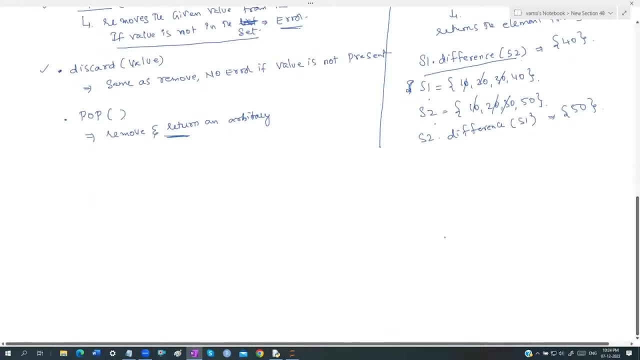 result. we know that it is 50, actually guys, what the point is. so it is going to be nothing but the intersection union and it is going to be different section of this, and if you remember the concept of um like, which is going to be something like, can i hope you remember actually guys, subset. 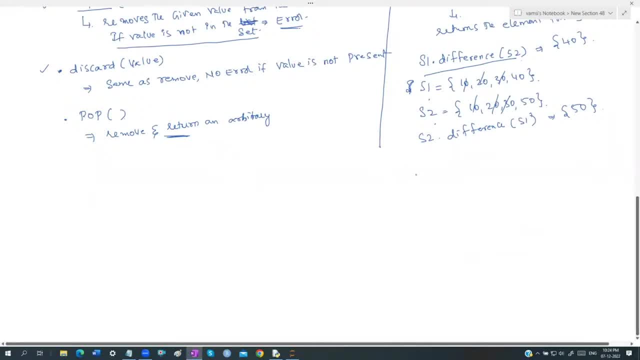 and supersets. actually, you know what is meaning of subset and supersets. actually, guys, if one set is also a part of another set, like, for example, we know that s1 is having some elements like 10, 20, 30- let us say that we have a 40 is there? s2 is having some elements like: we have 10, 20, we have a 30, 40. 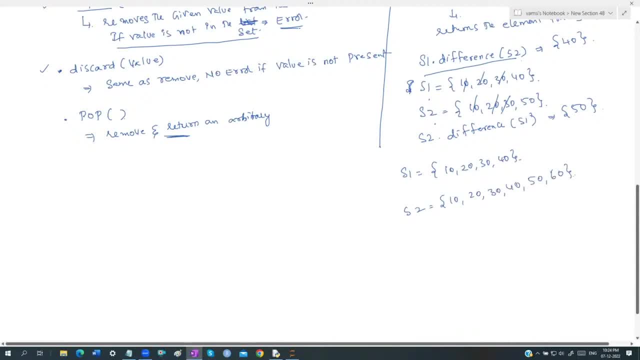 and 50 is there or 60 is there. now, if we can see, s2 is containing the s1. so s1 is nothing but a subset of s2 and s2 is going to be nothing but a superset of s1. what is s2? s2 is a superset of s1- s2. 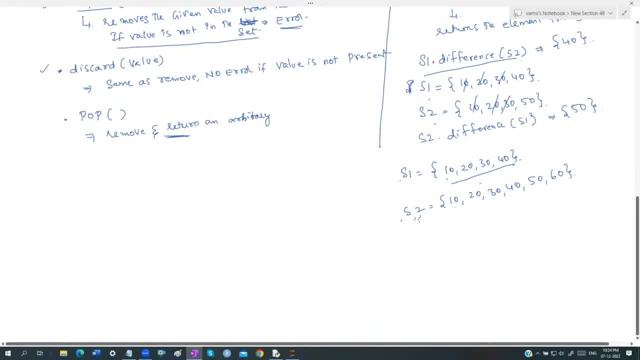 contains all the elements of s1. so if we want to check whether s1 is a subset, s2 is a subset, we have a method. is there actually guys s1 dot? we have a method called as an e subset of s2. is we are asking s1? 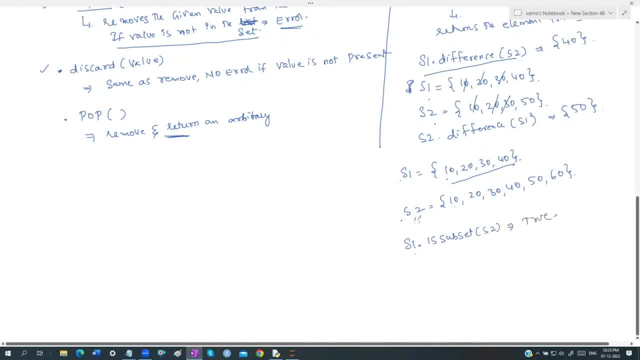 one is a subset of s2. it is going to returns true or a false, actually, guys. so you know that is subset and is superset. you are asking, you are checking whether this sub, whether this set, is a subset of s2, whether the s2 is a subset of s1. it is returning something like a true or false in. 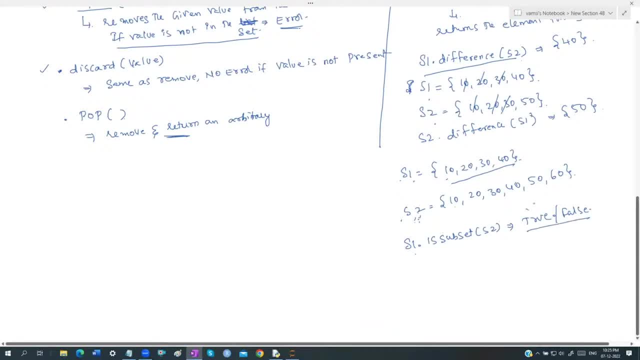 this case, s s1 is a subset of s2 now. so returns true, actually guys. now reverse order. i want to check whether s2 is a superset- actually guys. so it is a superset of s1. then also it is going to returns true or a false case. s1 is not a superset of s2 and s2 is not the subset of s1- actually guys. 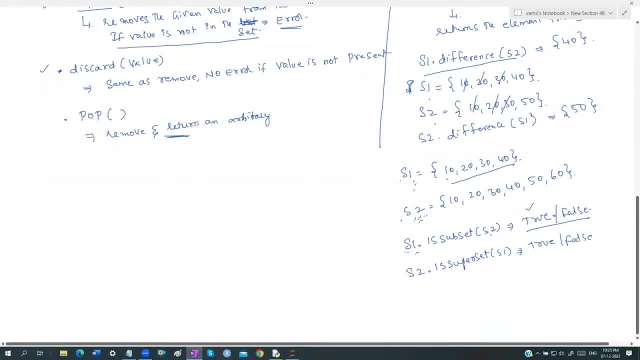 because s2 does not. s2 contains all the elements of s1, but s1 does not contains all the elements of s2. actually. so a little bit mathematics, guys. don't think that, sir? we learned a long back ago. it's a just like a refreshment class. 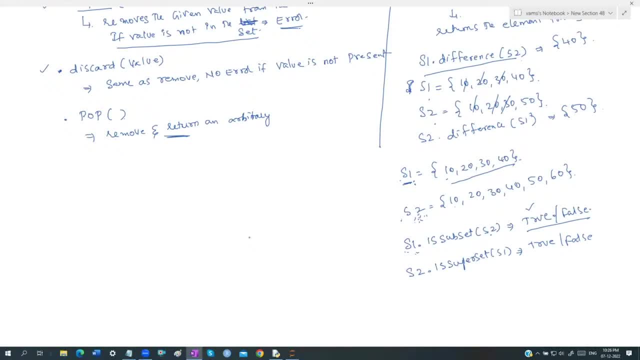 you maybe learn a long back. echo intersection union. it's a difference actually, guys, in mathematics we call it as a minus, here we are going to call it as an. a difference, is there? do you remember, guys, anybody, what is meaning of a disjoint? anybody guess? do you remember, guys, what is? 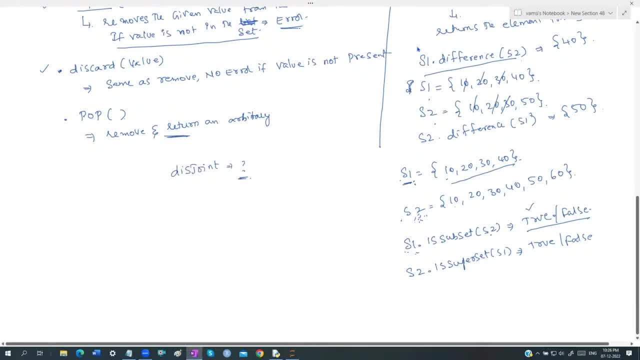 meaning of a disjoint actually, guys? no, this joint is nothing. but whenever two subs, two sets don't have any common values, then the two sets are nothing but what we call it as a disjoint. sets actually like, for example, a is having some elements like 10, 20, 30, 40, and whenever we are having b is having an elements like which: 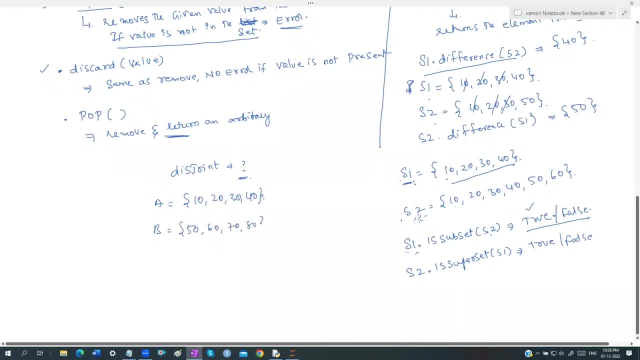 is going to be 50, 60, 70, 70, 80. now, what about the a intersection b? actually, guys, in mathematics i'm writing it actually: a intersection b is going to be nothing, but it's an empty. actually, guys, that means there is no common values, are there? so, if you want, then the a and b is nothing, but. 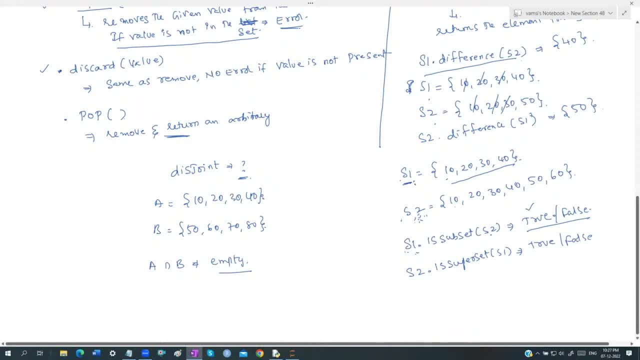 what we call it as a disjoint sets. actually, this joints joint set section. okay, so if you want to test, we can test it. actually, guys, it is a, dot is disjoint of, which is going to be nothing, but it's a, b actually, so it is going to tells you whether it is true or whether it is false actually. so see, 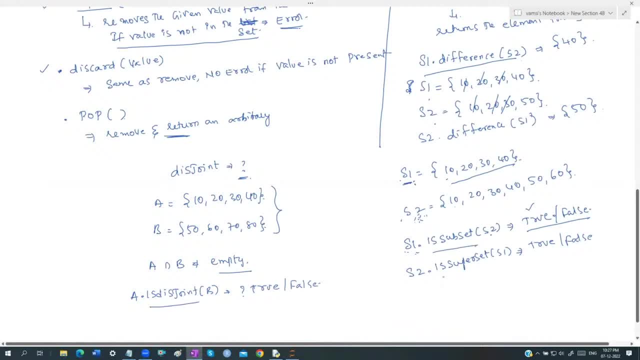 guys is disjoint, is subset, is superset. they will only checks out whether it is a subset and superset or whether it is going to be a kind of a joint. actually, it's a negation, actually, yes, it's an okay opposite. it's a negation, it's a negation. 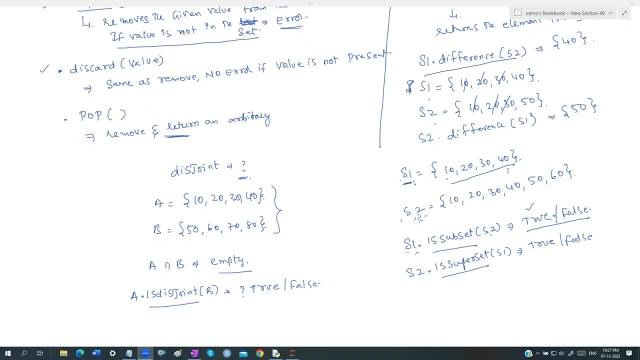 actually intersection is nothing but which is a common values will be there. this joint means nothing but which do not have any common values, which have common values which do not have the common values. that's it actually. yes, okay, so just we can play with the things. we can just play with. 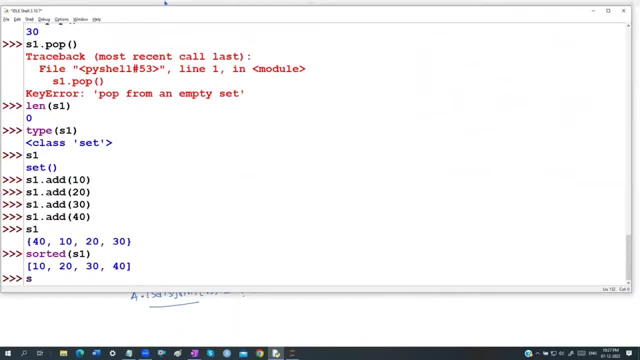 the things actually just you can also do by yourself actually. yes, i think one or two days back, maybe you may be having a little bit confusion to understand them actually, but now you got a little bit, uh, control on this. all these topics, actually it is going to be 10, 20, which is. 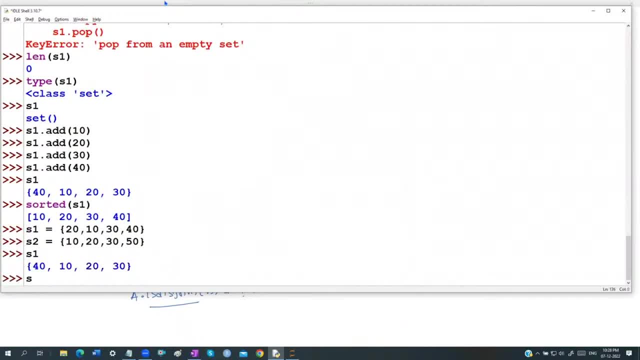 going to be 30 and 50? actually, yes, if you want, i can show you once again: s1, s2. actually yes, s1 is having 10, 20, 30, 40, s2 is having 10, 20, 30, 50. so how do you do it? actually, yes, s1, union, s2. 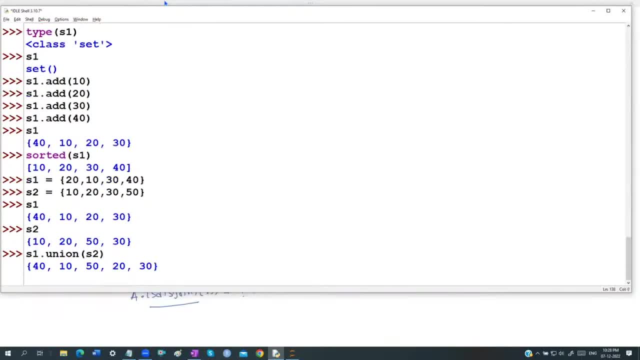 very simple: guys returns the union of the sets you as a new set. so 10, 20, 30, 40, 50, and you know that s1 union s2, s2 union, s1, both of them are going to be same, only guys. there is no change in the output, same as it is. what is intersection actually, guys? 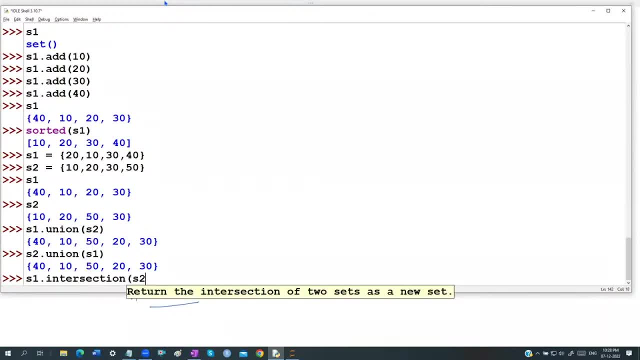 intersection of s2 returns the intersection of two sets as a new set. actually s1 intersection s2 is going to be 10, 20, 30, even s2 intersection s1 is also going to be same result only no change in the output. but what? 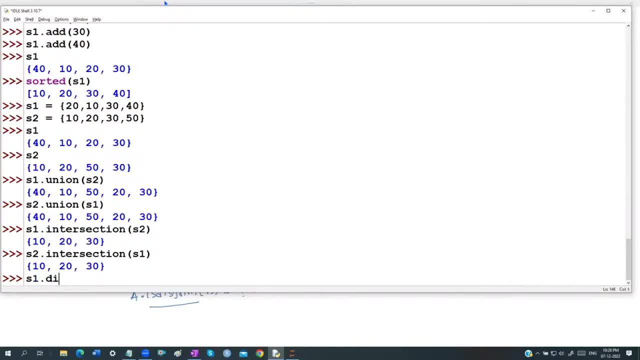 about the difference. actually, guys difference is nothing but minus. we have a function. is there method? is there actually guys? difference of s2. you can see very clearly: guys, what is difference will return. return the difference of two or more sets. as a new set, it is going to be s2 actually. yes, 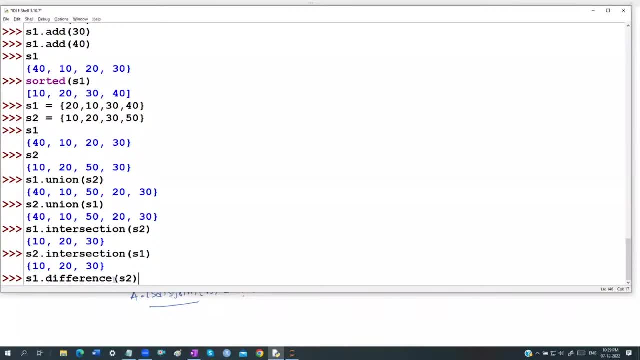 that means what we have to do, guys: s1 minus s2. so s2 should be eliminated from s1. what is there in the s1 after removing the s2 from s1? what is left over, and what is left over when we remove the s2. 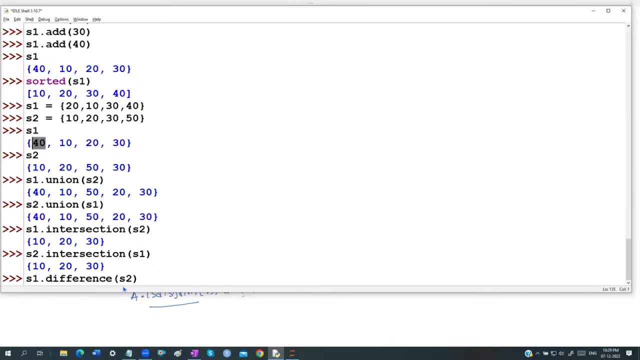 in s1 less. don't think that s1 difference s2 means it is s1 is removed from s2. no, it's s2 removed from s1. so what is left over in s1, which is going to be 40, is the result actually. 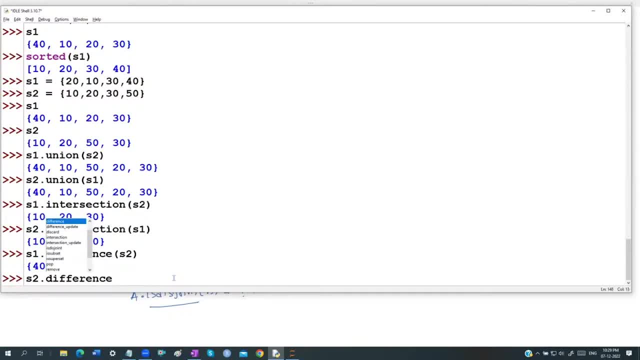 but when you do s2 difference, s1, then the reference is going to be nothing but difference output. less so we know that a union, b and b union is the same associative property. a intersection, b and b intersection is the same, but a minus b, b minus a is not the same case actually. 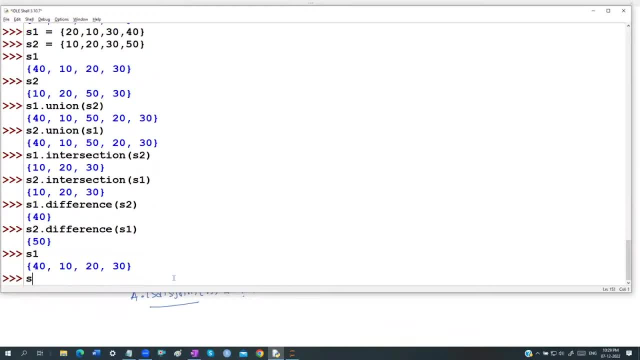 same as it is. we have s1 and s2. actually, guys, here s1 is not a subset of s2, s1 is not the subset of s2. guess what is meaning of subset? all elements must be there. so all elements of s1 is not there in s2. all the elements of s2 is not there in the s1 actually. so 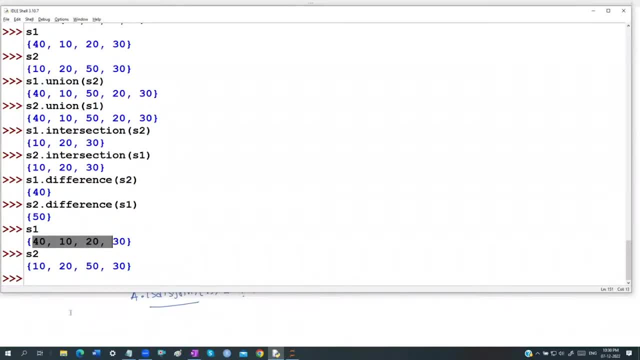 s1 is not a subset. s2 is not a subset. none of them is a superset. actually, guys, s1 dot, which is going to be. i'm asking guys, is you can see there guys, if um is is disjoint, is subset, is superset. is s1 is a superset of s2. returns whether this set contains. 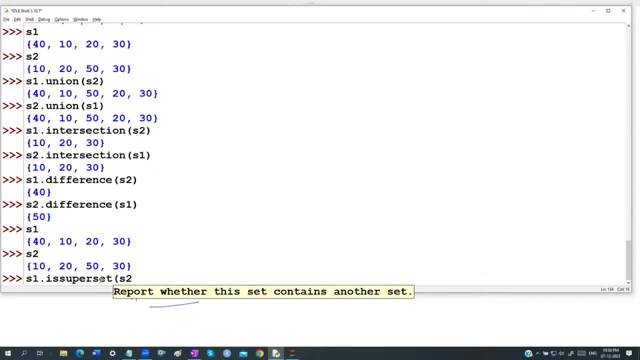 another set. you know superset means it contains another set. it is subset means this set is part of another set actually. so s1 is a subset of superset of s2. it's a false is s1 is a subset of which is s2 returns whether other set contains this set. actually, yes, it is going to be none of. 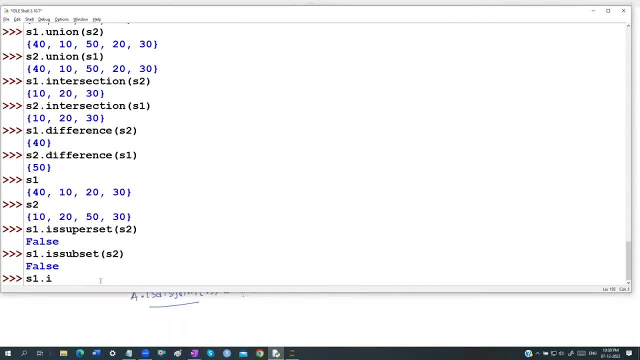 them is going to be true, guys. even s1, intersection, s2 is, it is a easy to say- disjoint actually, yes, they are not disjoints actually, because there are some intersection common values, are there, guys? all of them are returning false. actually, yes, but if you want to return true, you know what? 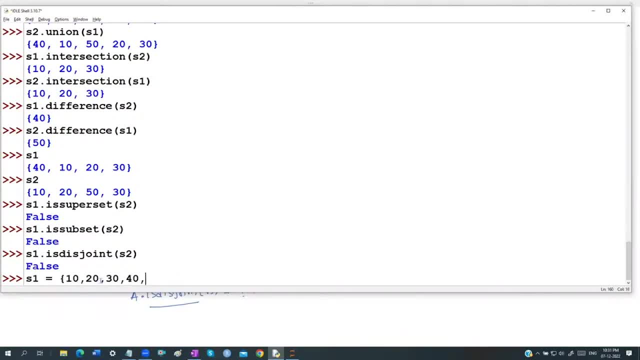 we have to do it actually guess. s1 equals to 10, 20, 30, 40 is already there. s2 is equal to nothing, but otherwise i'll do one thing is: s2 is equivalent to- um, let us say it is sorry. s2 is equal to 10, 20, 30, which is a 40, 50, 60, 70, actually, guys. 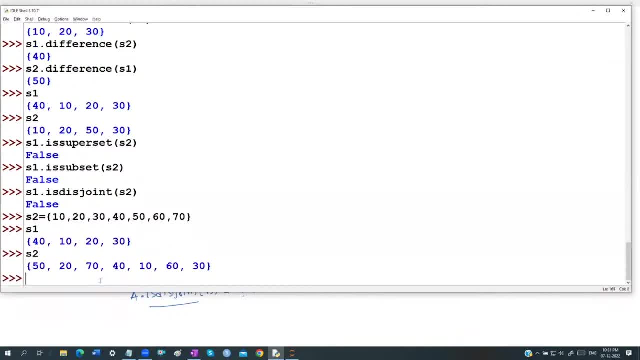 just an idea about that. s1 is this one, guys. s2 is this one. now, whatever the elements of s1 is there, all elements are there here, guys. that is 10, it is 20, it is 30 and it is 40.. so here s1. 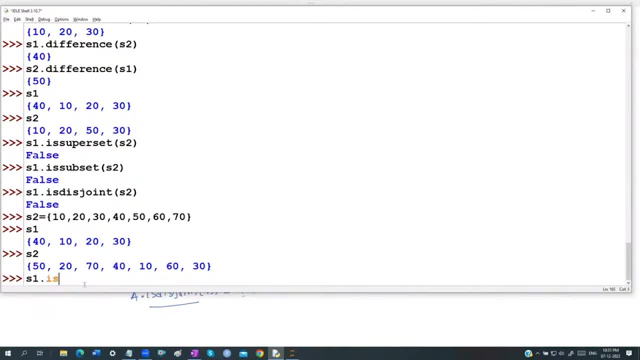 is called as an subset of s2. now you can ask: is s1 is a subset of? is it is a subset of s2? yes, it is a subset of s2. is s1 is a superset? no, it is not a superset, actually. yes, 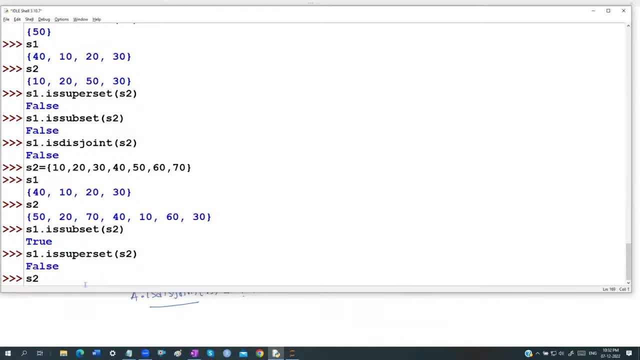 it is not a superset of s2 actually, but s2 is a superset of which is going to be nothing, but it's a superset of s1 actually. yes, that is the idea of how we are working with and how to how to say that it's a disjoint actually. yes, s1 is equals to, i said, 10, 20, 30, 40. 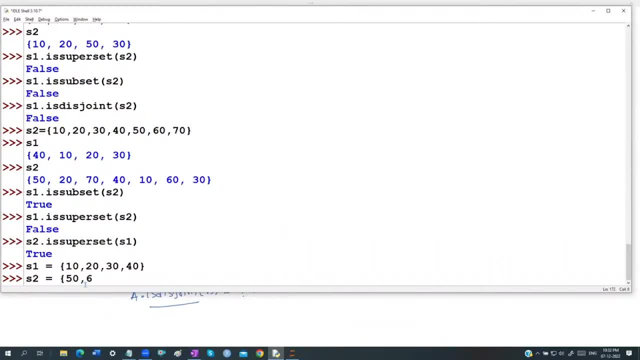 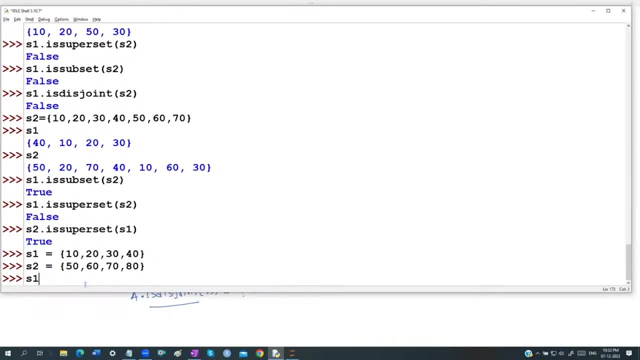 whereas s2 is equals to, let us say, 50, 60, 70 and 80. actually, guys, if we can observe carefully, there is no common values. yes, s1 intersection with s2 is going to be nothing, but there are empty list actually. yes, you can see. 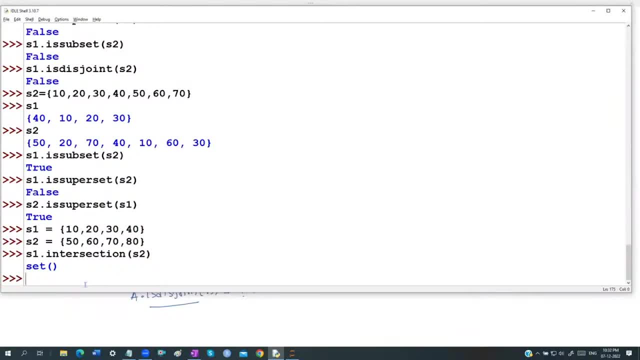 empty list is coming, then whenever there is no common values between s1 and s2, there is no intersection values. guys, union i can do guys, but intersection i can't. intersection is empty. so whenever there is no common values, then s1 and s2 are basically what we are going to call it as an. a disjoint functions what the disjoint sets what. 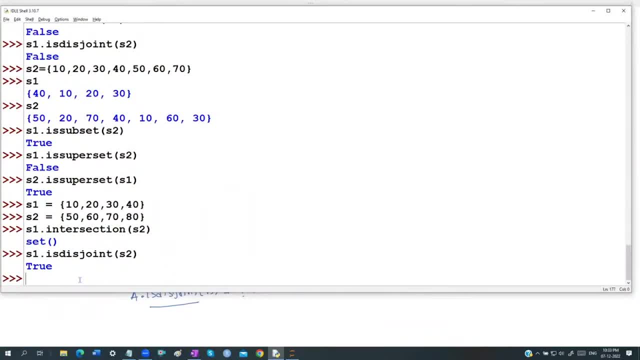 we are going to call it as actually. yes, we have a number of methods actually, guys, if you remember, in list concepts: first today, i taught you three methods. second day, i taught you another three methods. after that i have discussed about the remaining one or two methods. i have been 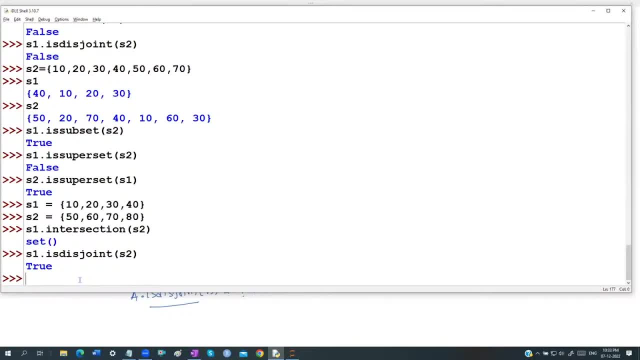 discussed about the three or four. i think. first class it is four, second class it is three and next class it is three. i have been more discussed, but today how many methods you'll discuss, i will discuss it actually. guys add: uh, we have been seen about a clear. these are common methods actually. 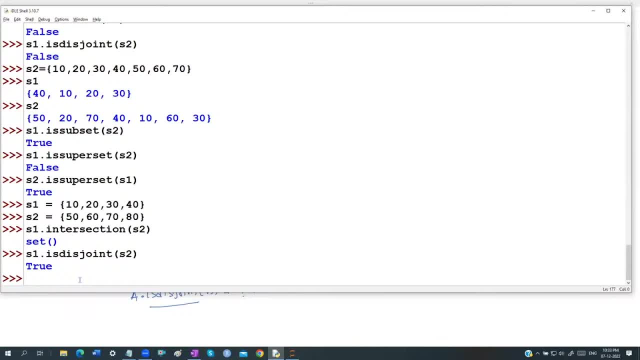 guys, remove discard, pop now intersection union at this, uh, minus, which is going to be the difference? actually, guys, each subset is superset is disjoint, so almost all we are having somewhere around 11 or 12 methods we have been got discussed. guys like that, we are going to be the same methods, only, guys. 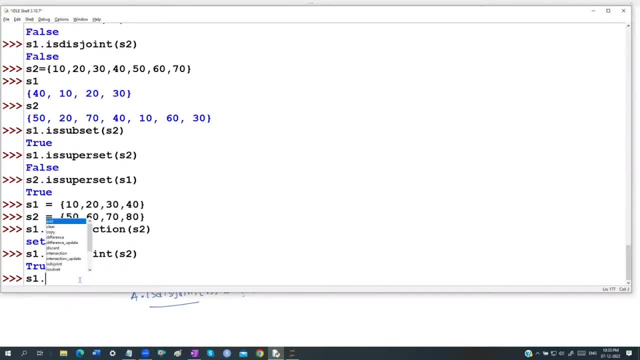 if you see them. i totally know i don't have anything to hide from you. add clear copy. i told you guys i don't discuss about that difference. i already explained guys: difference underscore update. i'll explain it. difference: difference underscore update slightly difference is there guys? discard intersection, intersection underscore. 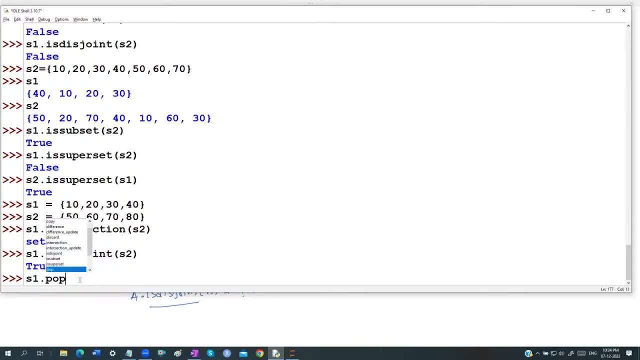 update. is there, guys, is disjoint, is subset, is superset, pop, remove. we have something called as an symmetric difference. actually, guys, i'll tell you guys what is meaning of a symmetric different. nothing is there. symmetric difference is going to be nothing, but it is a minus b, union, b minus a. 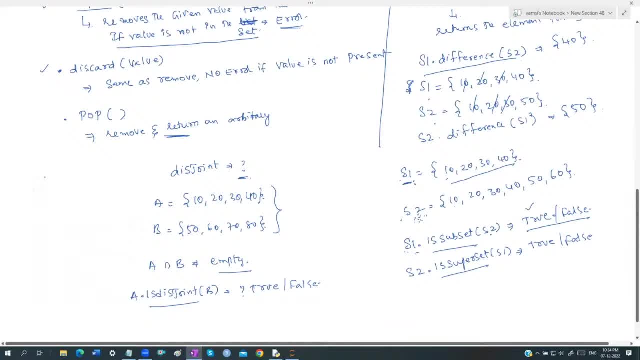 that is what we call it as symmetric difference. actually, you know what is the difference? actually, guess difference. you already know about that. difference means which is going to be a minus b or b minus a. what do you mean to say? symmetric difference? actually, symmetric difference, what we are going to call it, as it is going to be nothing but the union between a minus b. 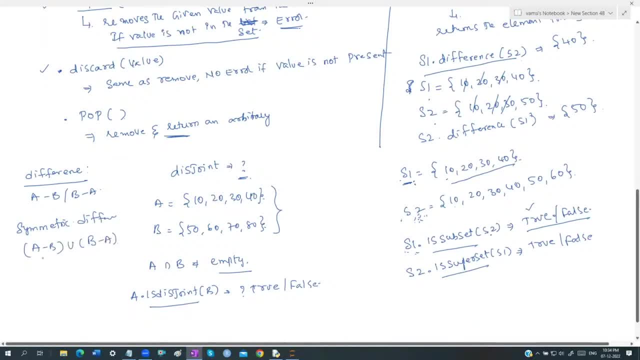 union. it's a, b minus a. so what is output? actually, guys? the elements which are there in a but not in b, the elements which are b but not in a. that is going to be nothing but what we call it as a symmetric difference, actually, guys. okay, mathematically it is what we call it a. 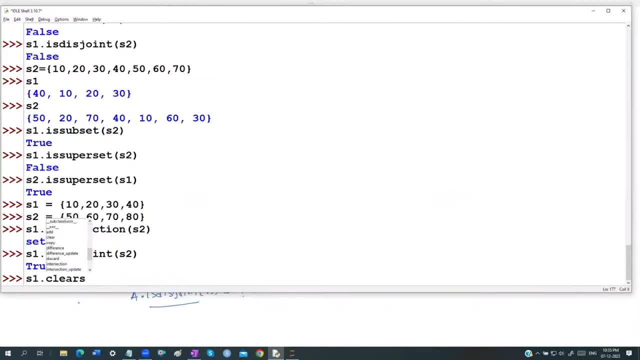 symmetric difference, semantic difference, underscore update will be also there. it is semantic difference. underscore update is also there actually, guys, s1 dot. if i say s1 dot, you can see it actually. symmetric underscore difference. uh, underscore update will be there actually. yes, okay, i'll tell you. if you know symmetric difference, understanding symmetric. 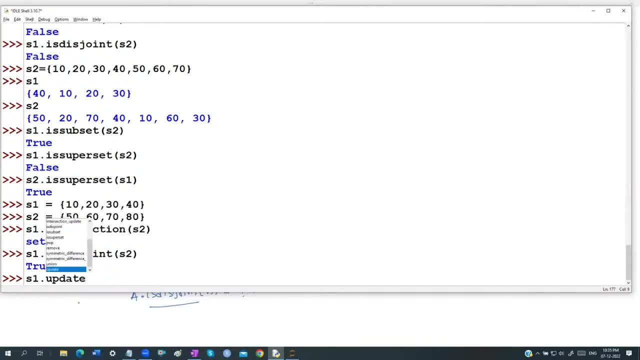 difference: update is also same, actually union and we have an update, is there nothing difference? is there guys? just, there are going to be just a small extension. you know intersection, intersection underscore update. you know difference, difference, underscore update, union. it is actually union underscore update. actually, guys. this, actually the dashboard, also the actual for the union factor is: acceptor, but i've laứngedently learned this. first there stopped, but now it is released. it is there. yes, so this also. it is added right now for r1 to r2. right now it is actually connected r someone else in the right now. that's because showing the vector and r1 moved away. it was not stopping this, for r1 converted way to r2, giving an. 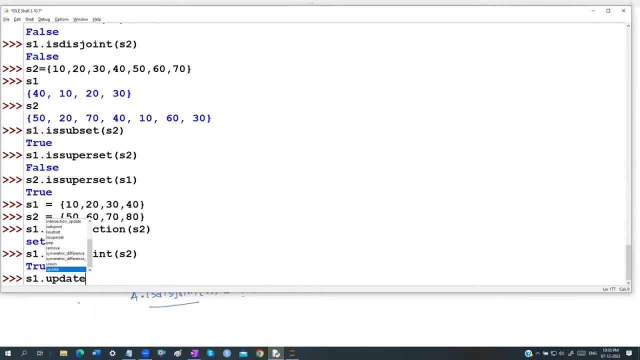 important function just remaining. there was some error that you cannot control on that as one over division n 10: update is actually the given as a name as update actually, guys, but is indirectly. it is union underscore update actually and we have a discard and we have a discuss. sorry, we have a symmetric. 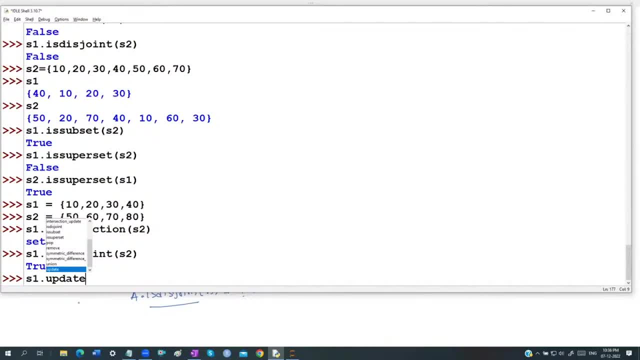 difference. we have a symmetric difference. underscore update. is there just five minutes? it will take it actually, guys, tomorrow. i'll just explain the concept because already 1035, so i'll take up in the tomorrow's class and tomorrow i'll finish off this one as well as. 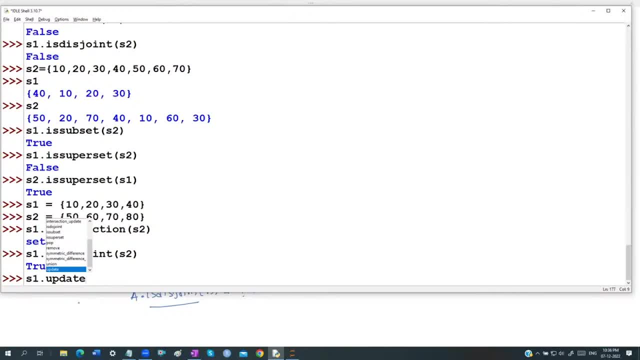 there is a one more concept called dictionary objects. actually, guys, will complete of that particular dictionary objects, and then we'll think about, like that will complete of your basic data structures, guys. then what is the next level, what is the next concept? we have to discuss it, actually, guys, okay, so that's it. um, i'm ending the session for today, guys, we'll end up the session. 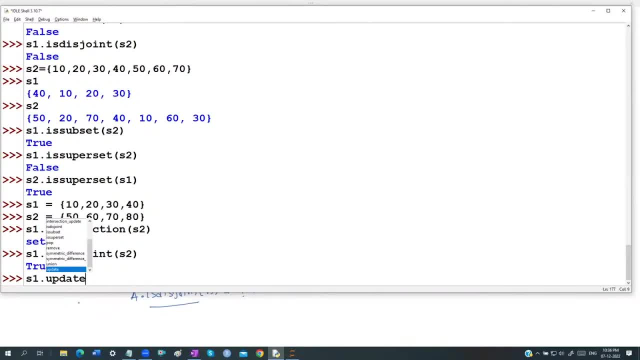 for today. uh, if you have any questions, we can discuss it. guys. anyone guys? do you have any questions like: why don't we have these options for list? also, you once, if we have it for the list, because list is going to be accept multiple values- it will take it. 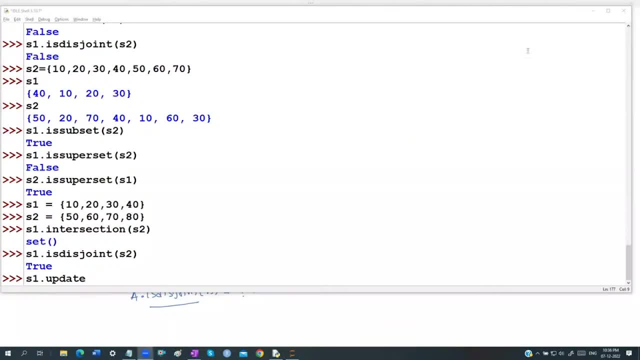 so it's an all predefined classes. actually, guys, it's going to be all about the predefined classes only, so they given the functionality we have to use as it is. so if the same functionality is given by all the single object, then we don't really require them actually. so set is going to be one. 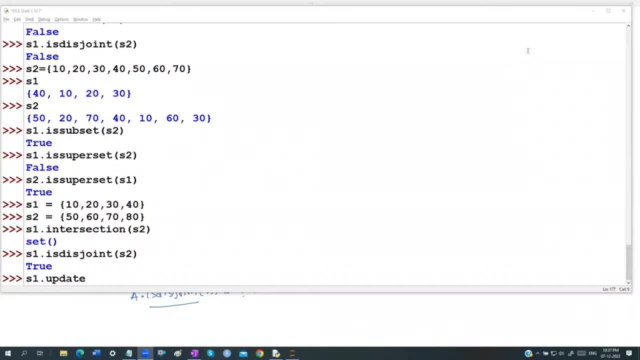 kind of like mathematical operations. you want to do that, so why don't you have it as a set object? means, for example, if i put it for the list, it will take it as a set object, and then it will take it as a select object. but um, we don't need the set object as it is, so so it is good instead of where it. 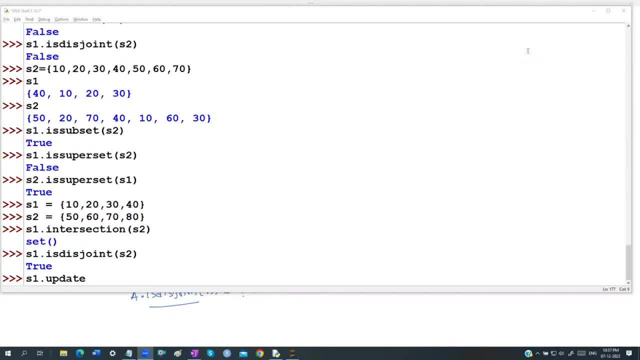 comes in there. we just write a set object for violator. there are the importa dead or even therires or whatever, weiter and so on, and these will take from a base object also. so list is going to be. gets contained multiple values: duplicate values will be there. so their slicing and indexing. 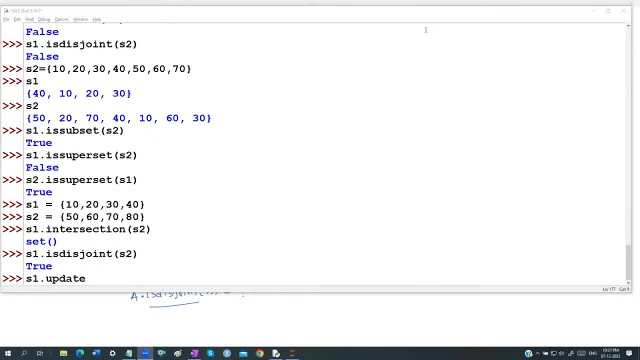 is all停 and indexing is not hello, so it's going to be functional distribution. they have been results. okay, fine mission. yeah, i like your, machine machine learning will still takes a long time. okay, core python should be completed. numpy pandas, data visualizations: these are the prerequisite to start. 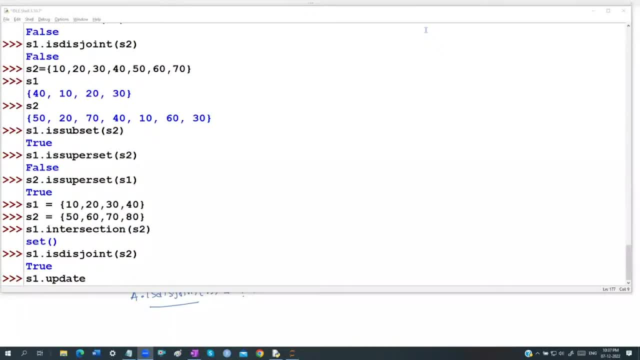 with the machine learning. so all these topics will take around 40- 45 days. after that, machine learning will start. okay, fine, these are all prerequisites. whatever you're learning is a prerequisites. fine, right guys? um, what will be the next topic? next topic is going to be: 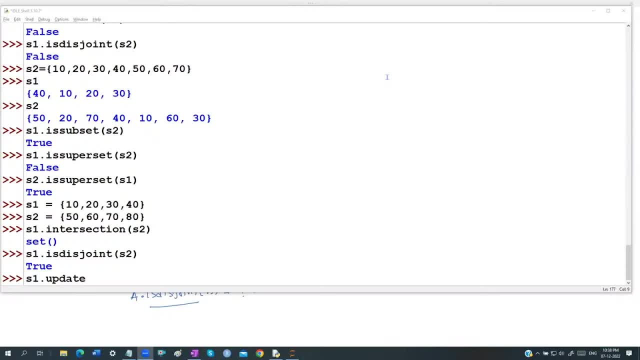 before going for the next topic, we'll see what are the other ids. are there? like we don't work with this idle anymore because it becomes more complicated in the coming classes, so we have a different ids. are there? so how to install them, which id we prefer and even we are going to be? 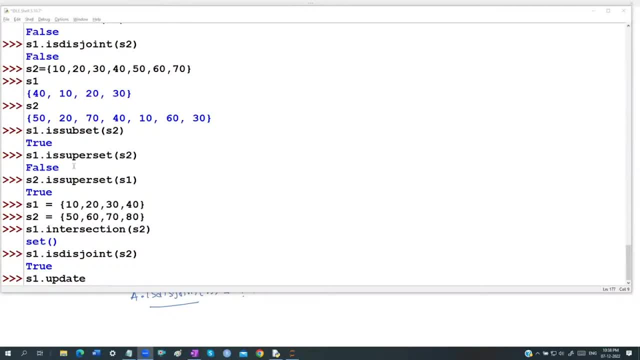 using something called as a jupiter notebooks. i use a jupiter notebooks actually. so how to set up the jupiter environment, that will be almost all. one day it will take it and then normally we will be using the jupiter notebooks and then we will be using the jupiter notebooks. 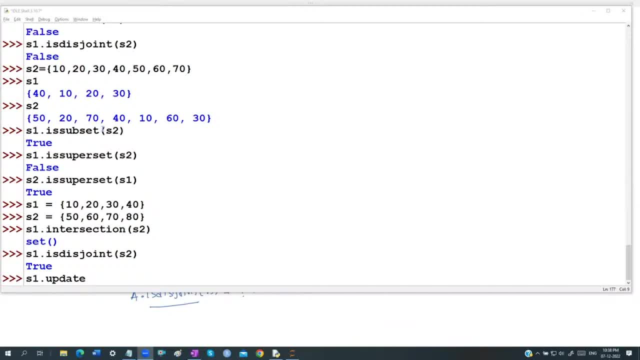 and then normally we will be using the jupiter notebooks and then normally we will be using the like a common programming language, uh, conditional statement, control statements, uh, if and for, statements that common things will be there, and after that we have some classes like string classes, uh, we have something called as an comprehensions functions topic. those are the. 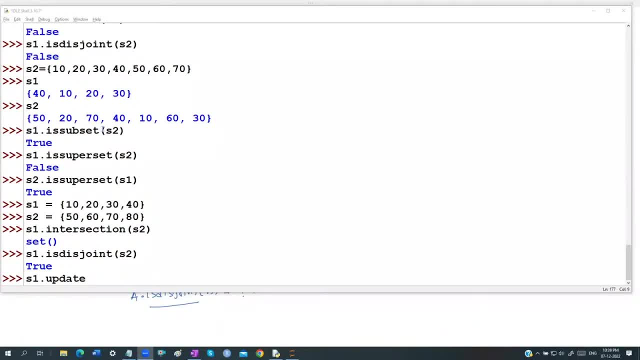 some of the core concepts of python, what we have to discuss. it may be another one more week. it will complete off, guys, okay, fine, guys, um, just uh. we'll end up the session for today, guys, and please attend the, i think who has been joined lately? and one more thing, guys, please, um, if you want to take up the course, some people has been joined. 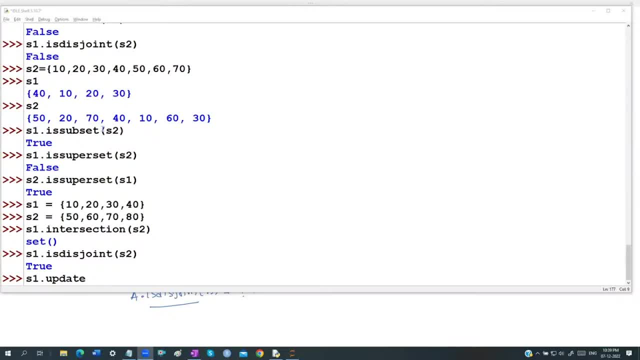 uh, lately, so please get registered. um, i think you can have all the following: the payment procedures and all these things, so that you can get all the access to the drives. all the backup sessions- links, videos will be coming. you need not to wait for the backup sessions also, so you can go through. 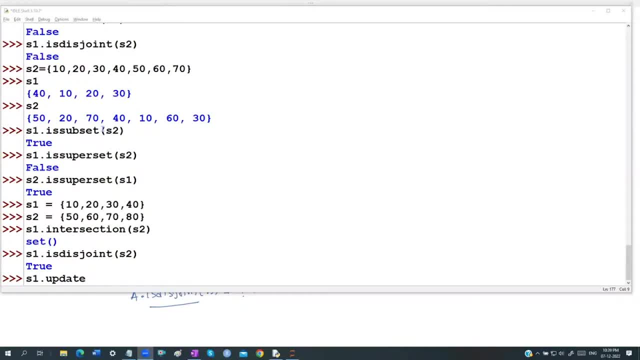 the videos and you can take up the particular classes also. so please complete off all your payment procedures and all these things. we are, we are just closing the batch process by end of this week. guys, we are just closing up. we are not going to add up no more, if anybody. 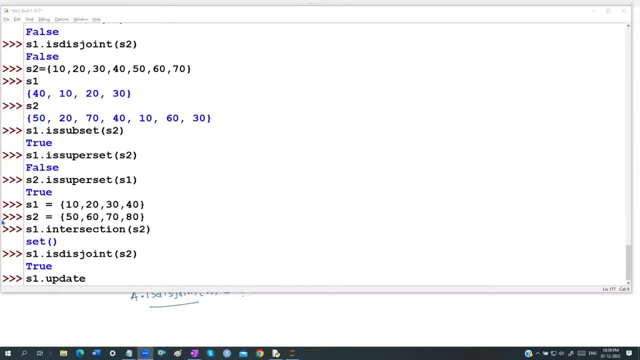 add ups also. they will there. it's only their interest only. we don't take any backups and all these things from the next coming week actually. so that's it guys. uh, we'll arrange a backup session. uh, based on your discussion base. i'll discuss with the participants one. 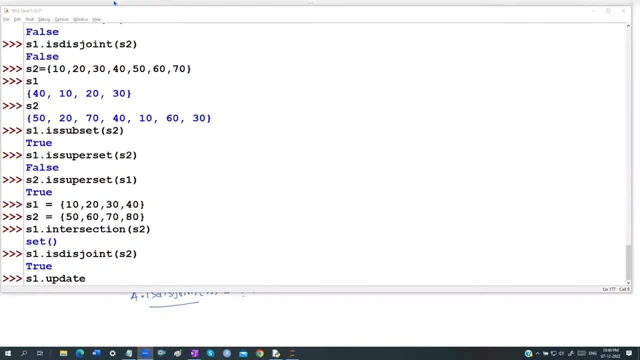 which i'll discuss with all of you and i'll arrange it actually, right? anyone, guys, any? any more questions we have, sir, i have a question of yesterday's, an index question. yes, yes, sir, actually we in sir we have taken some element: x is equal to 20, 30, 40, 50, and then we find the 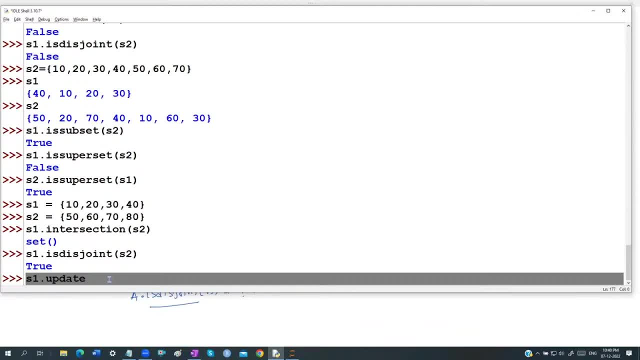 least value, we'll find the least value, okay, okay, okay, minimum is a function. what we have it actually. yes, sir, okay, minimum is a function. directly, you can find out what is the minimal value. do you want to know what is a minimal value, or do you want to know where is a minimal value, sir, actually it. 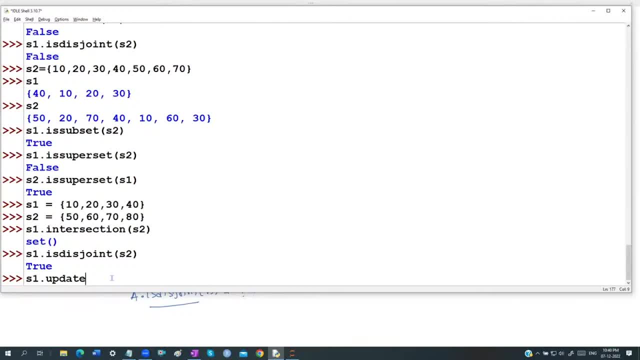 is going to be of the least value. but, sir, here, not least values, not least values. actually it is going to be wherever it finds the first occurrence it is going to returns. that, okay, your point is correct. it's saying that wherever it is going to be the minimal value, that means wherever it finds the 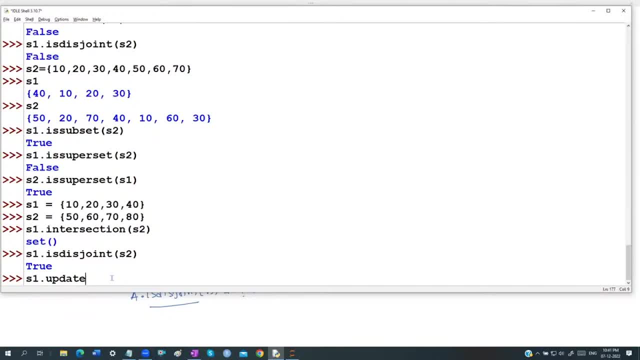 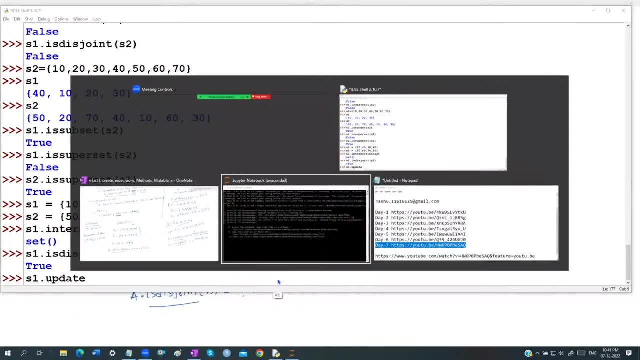 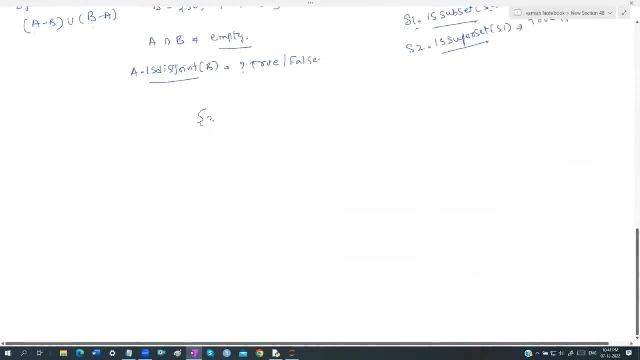 first, first occurrence. it is going to tell you that particular index. it is going to tell you about that. so what is your elements? you have, if you, just if you give an idea, what are the elements you want to take? so 20, 34, okay, okay, okay, okay, 20, 34, your example. i didn't remember yesterday's values, no, 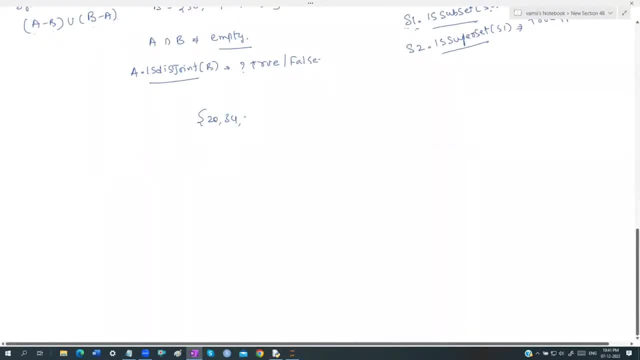 okay, 20, 34, any, just just tell me some ideas about that. okay, 40, 12, 16, 18, okay, some 12 again one more time. uh, let us say 6, 8, 16. okay, let us say 42 and something like an 8 for example. okay, shall i take. 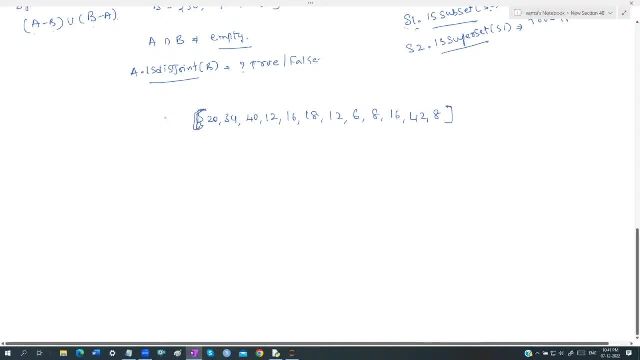 these values, for example. okay, now tell me, what is your requirement now? index is going to tell you. index is going to tell you like, for example, i'm asking 16. where is the particular 16 index is there. this is 0, 1, 2, 3, 4, it's a 5, 6, 7, it is an 8, 9, 10 and 11. so where is the? it will. 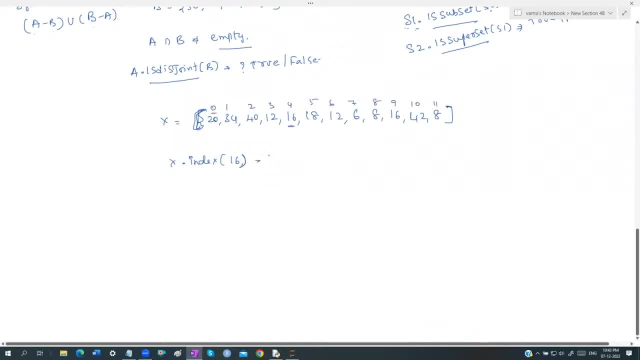 start from the 0 index. actually, where is the first 16? was there actually? it is there at the 4. it will return the 4 as a value. did you got it? yes, sir, okay now. what is your question now, sir, if? if we find sir x dot index, okay, two and eight, two. 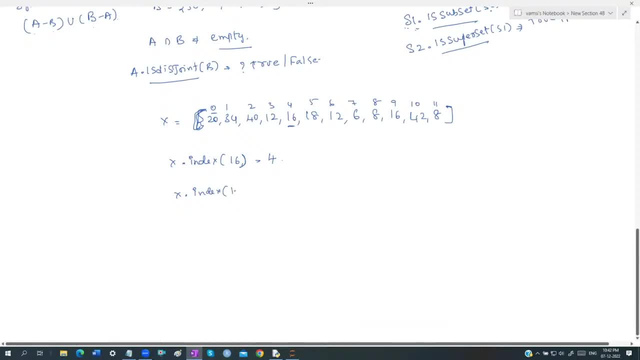 first value is going to be 16. yes, sir. okay. next value is nothing. but where to start your search? by default it will start searching from the zero here only. for example, if i start searching from seven now, can you tell me it is going to start from the seven here? now it will start searching. 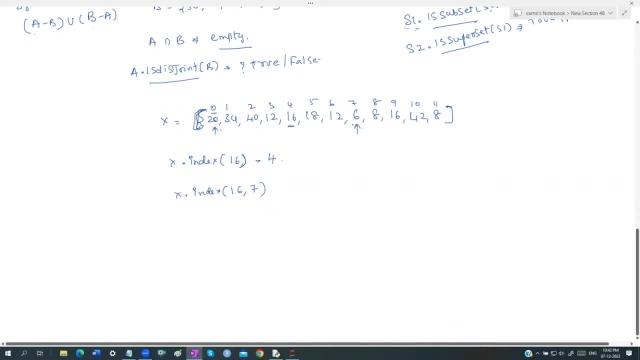 from here now. now tell me, where is the? where is the first occurrence of 16? is there now? actually, it is there here now, right? so what is an index? it is going to be there now. yes, are you there? yes, sir, yeah. what is output now? where is? 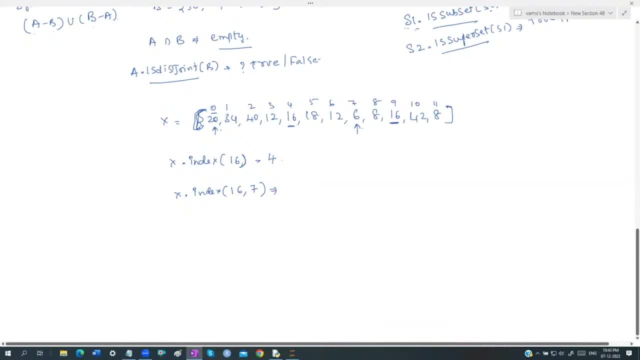 the 16 is there. whenever i start searching from seven here now, where is index? is there nine, nine? it's going to return the nine as an output action. so where you want to start searching, that is going to be the searching criteria here now. if i don't specify anything, it starts from searching from here itself. 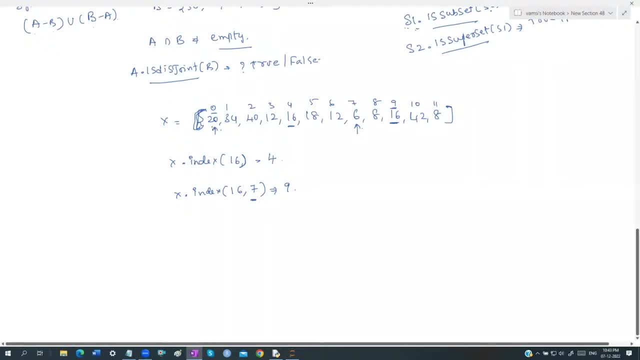 okay, okay. for example, if i said x, dot, for example, if i said index of, if i said 16 comma, for example, 5 comma 8, if i say just an example i'm talking about, then can you tell me what is meaning of 5 comma 8? now search for 16. where to start your searching? now start from the fifth index, right? 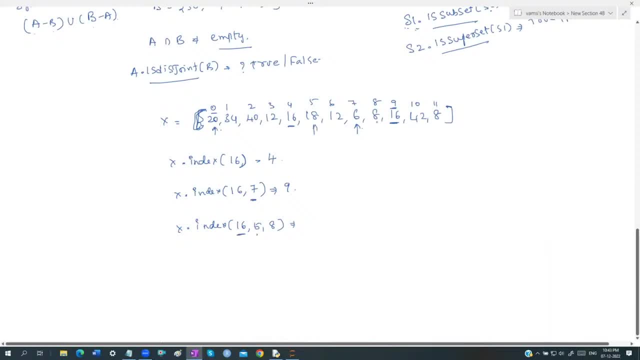 from here and where you have to go up to there, up to 8. it's not up to 8, it is before the 8. only. that means only. it is going to search for 16 only in these three elements only. so do you have the 16. 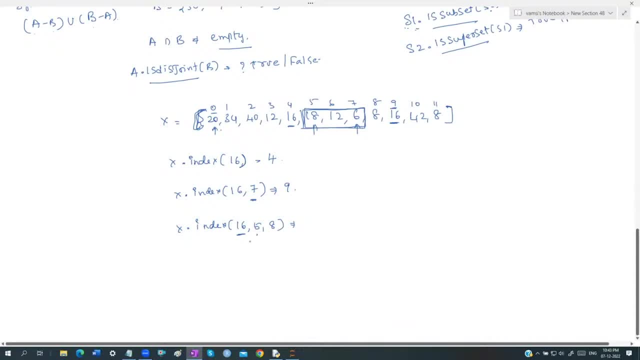 in this particular three elements. no, okay, so, no, sir. no, then we are going to get an error, okay, okay, okay. so where to where you want to search? if i don't specify anything, it will start from beginning. it goes up to the last. if i specify the starting index, only from the starting index. 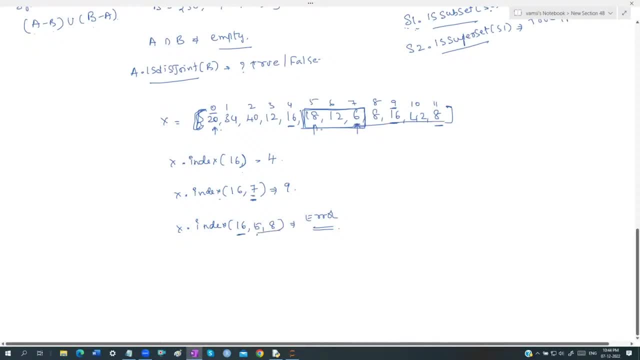 up to the last here if i specify both of them, starting as less ending. but five is the same, so included. it is going to be excluded. so it will search only for three indexes: five, six and seven. in these three indexes it will. in these three elements it finds a 60, it returns maybe five. 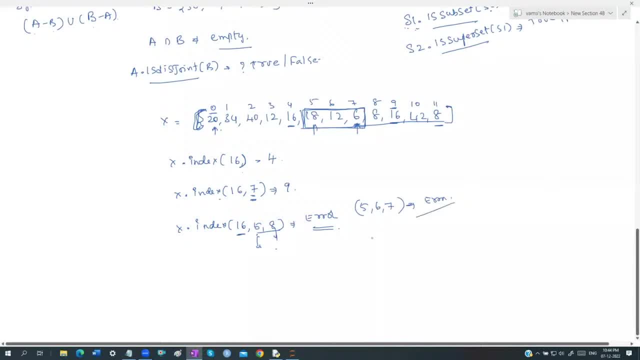 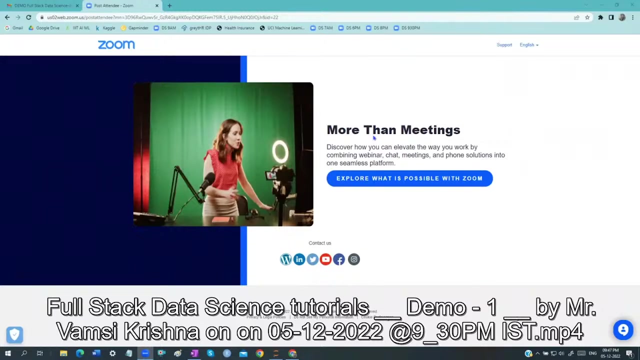 maybe six, maybe seven, otherwise we'll get an error, actually. okay, thank you. fine. so thanks for thanks for today, guys, and we'll meet up in the tomorrow's class. thank you, guys. uh, sorry guys. um, i was a little bit late actually just now. the previous class has been got completed. 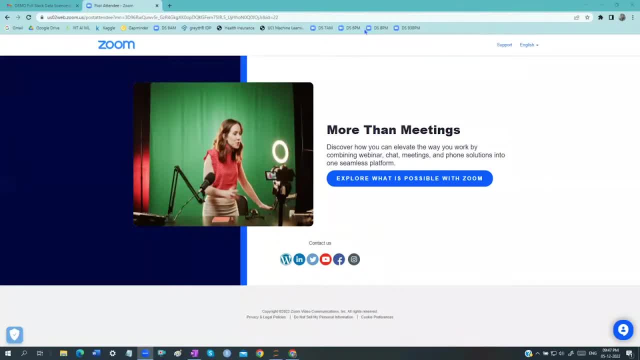 um, i can see some more people has been joined, guys, actually. so just let me tell you guys, uh, let me just give me two minutes of time let me check, like, who has been the new participants. um, like, i think so many people are there actually, guys, mano, her, yeah. 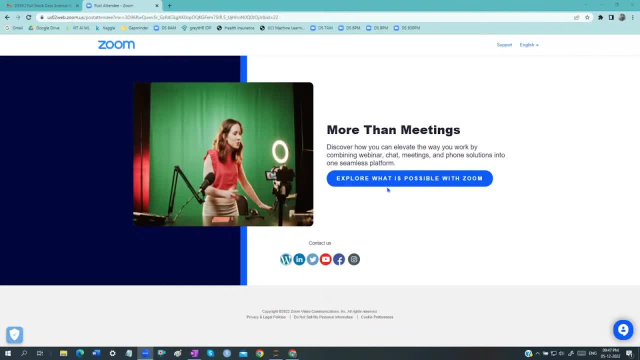 just give me a minute sonam. yeah, right, okay, guys. so, guys, i can see some, um, i can see some more people has been joined as a today's class. uh, today i think you have been joined as a demo class, actually, guys, but, um, let me tell you what has been happening, guys. so in the last week only. 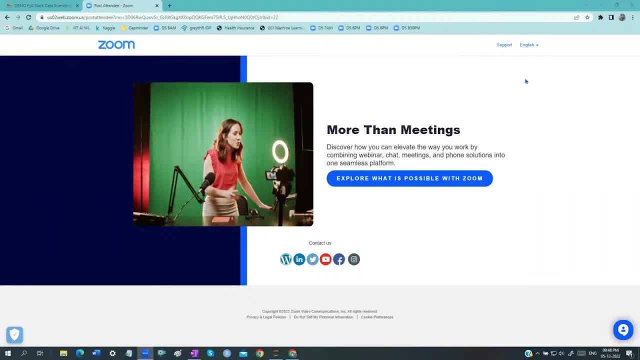 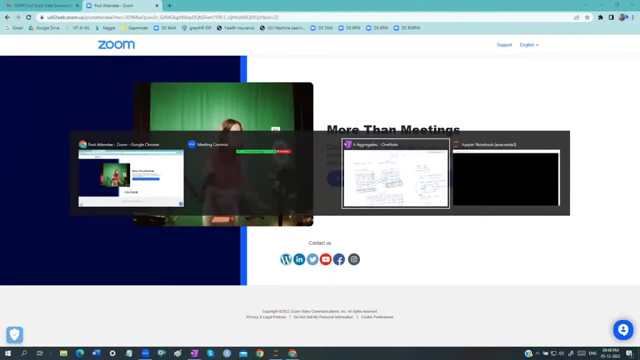 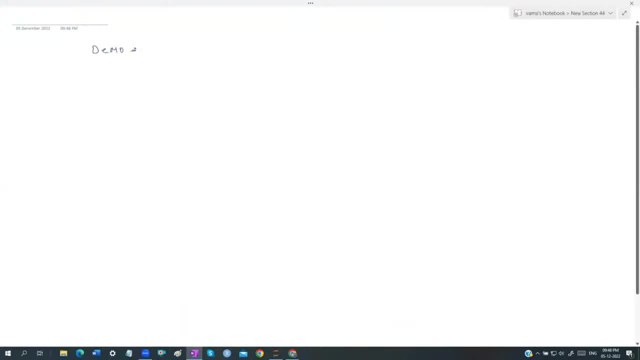 we have been started this session. um, last week means it is all mostly two weeks, actually guys. one week is a just a demo sessions, actually guys. so it is hardly two, two weeks it has been what happened. just we have been started with some. first week we have been taking a demo session. actually demo means like what is data science? 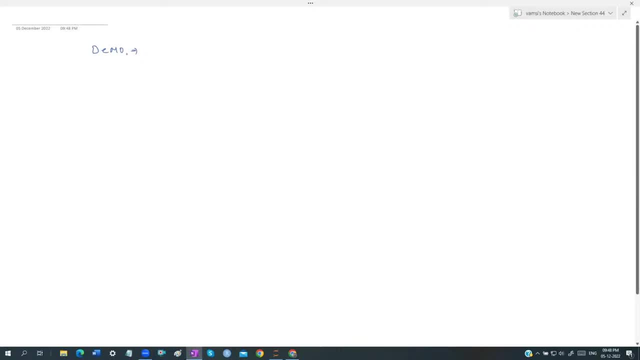 what is machine learning? uh, these are the some of the things, what i have been got discussed about that. so that has been happened for one week. one week means it is not too much time actually, guys. just hardly 45 minutes, 50 minutes class only i can see that actually we have been taken. 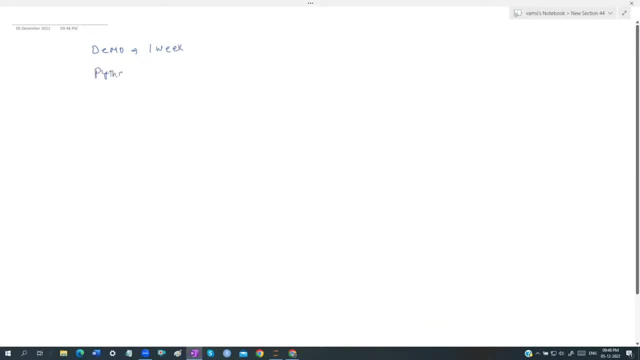 so in second week i have been started with the basics of python. we have been got started actually, guys. so this has been happened for some. another one week it has been what happened, but i can see some more guys has been joined now. so don't worry guys. um, i'm going to take some. 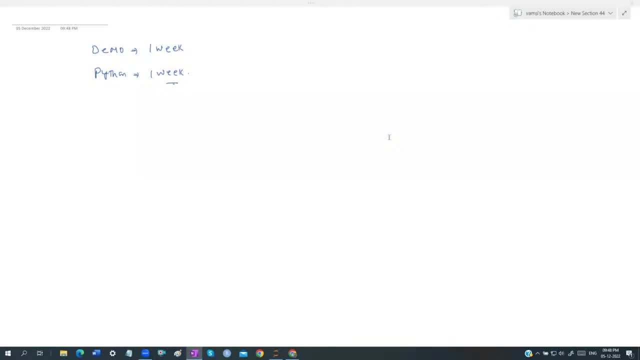 backup session actually. so i think i can say somewhere around seven to eight people has been joined for the today's class. i can see your names, like some names. i can see who has been joined for the today's class. somebody has been joined in the previous sessions- only but a very few people: seven. 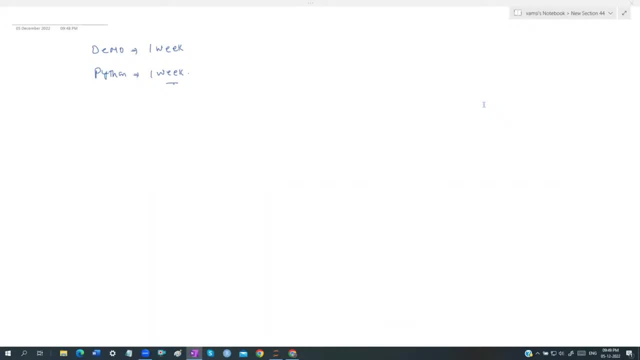 or eight people has been already joined. they have been already registered for the course. i can see another seven to eight people. i can see it actually, guys. so don't worry guys, because i thought that maybe one or two people may join, but i have seen a little bit more people has been joined, so don't worry guys. who has been joined for the? 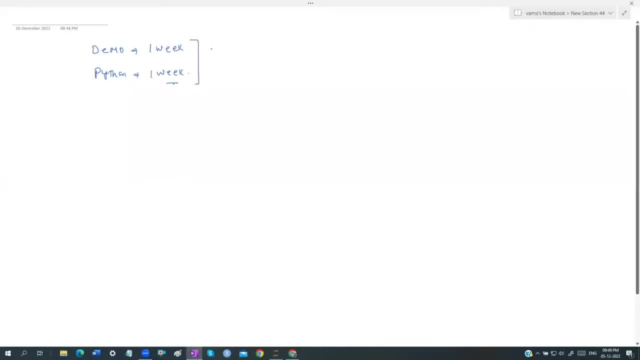 today's class, so don't worry about that, because, um, i didn't expect that these many guys will join. i that there may be some regular students. there are seven or eight students has been already registered. i expected that maybe somewhere around three to four people, but i can see somewhere around. 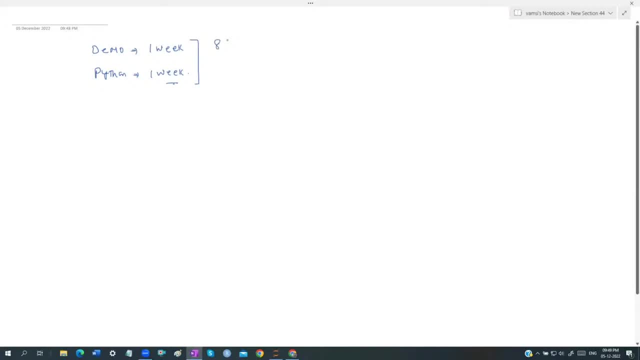 more than eight people, eight participants are there who has been joined for the today's class. so i'll do one thing: guys, don't worry about that, because what has been happened, don't worry about that. it's only basic things. if you are already having some core concepts of python, it's a very 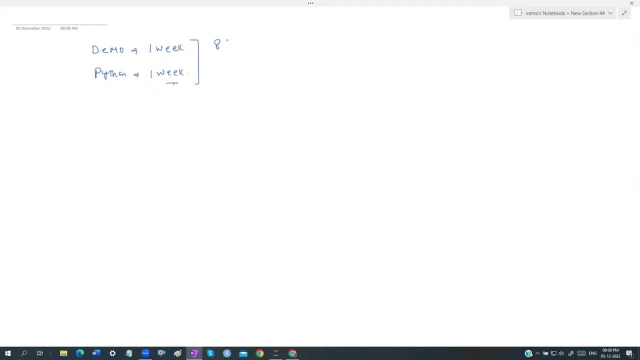 simple topics only, which you can understand them. don't worry, i'm going to take the backup sessions. guys, if you really feel that there is actually, i can give you a recorded sessions actually so i can take some kind of a backup sessions. i can take it actually, but just give me one or two. 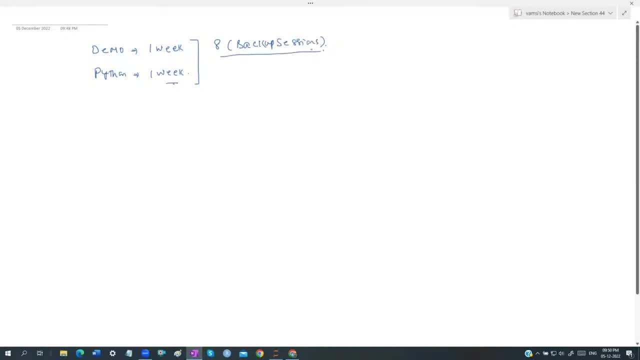 days of time. i'll arrange the backup sessions. actually, guys, okay, so don't worry about the completed classes. what has been already done, it's only basics and only some part of introduction only. we have been got started. so in first week, only only thing is: uh like what is data science? uh like what is machine learning, what we can do it in. 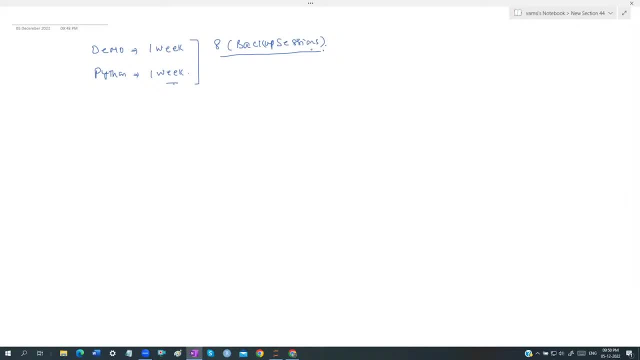 machine learning. it's only just an introduction part. actually, actual discussions will be there and actual explanations will be there whenever we start with our regular classes of machine learning, so that you can just go through the recorded videos and you can go through them and coming to the python also. guys, we are still in the basic concepts only, so don't worry within. 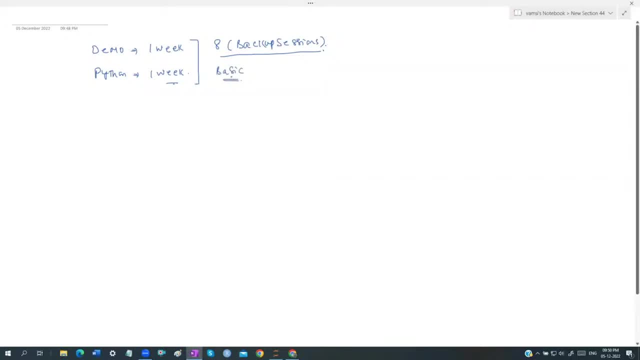 just two or three classes, hardly whatever. the basics i have been about discussed is hardly three, four days, concepts, only guys, not more than that. so what is my suggestion for the guys who has been joined for the today's classes? again, i cannot start from the introduction part in the today's class because i don't have a plan. i don't have a plan, i will. 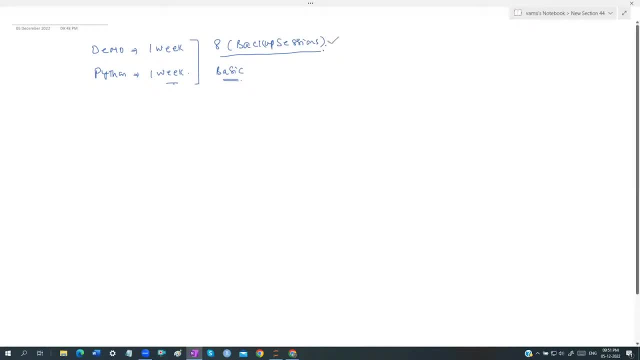 arrange the backup sessions guys. so, whatever the classes you have been got missed i am going to discuss as part of the particular backup session guys. okay, i'll plan it. i am going to plan those particular sessions and my team will intimate you about those particular sessions, maybe by the end of the week, or maybe some friday, saturday, sunday- even i'll take a sunday session. 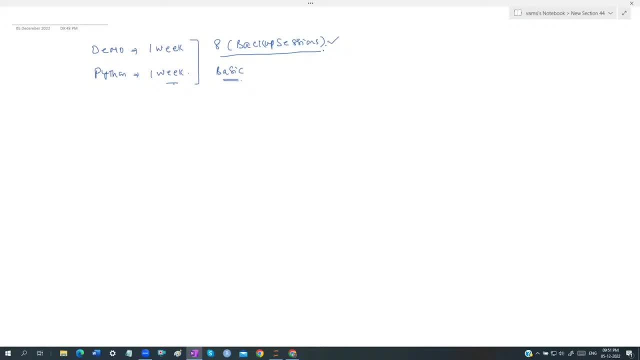 and i'll take some kind of backups and i'm going to make you understand whatever the missing classes are there. so we have not yet started with any machine learning concept. we didn't started anything about data science classes- actually, guys, actual classes. we have been not started about that. so don't worry about the classes. i just started with some introduction. 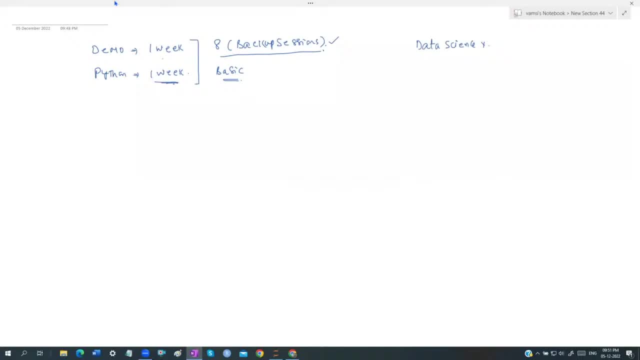 part of the data science and we have started with the one week of python classes only. we have been got discussed. yeah, i'll, i'll, i'll add them, we'll. we know, everybody's going to know about that. we'll have all that information. i'm going to do that, actually, guys. okay, fine, so don't worry about that. 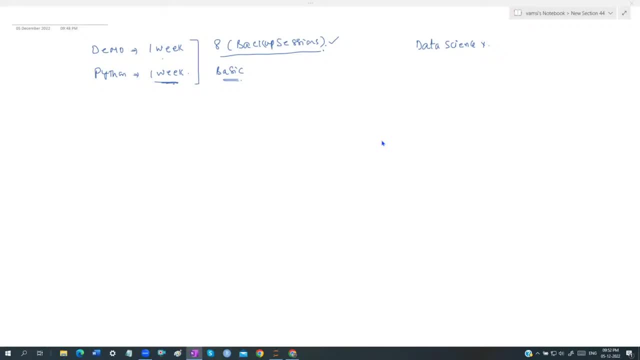 no, no, it's no worries, don't worry about this, guys. my backend team will have all your details and they will take care about that. okay, i'll add up everything in the backup session. who has been everything will will will share it with you. okay, fine guys. 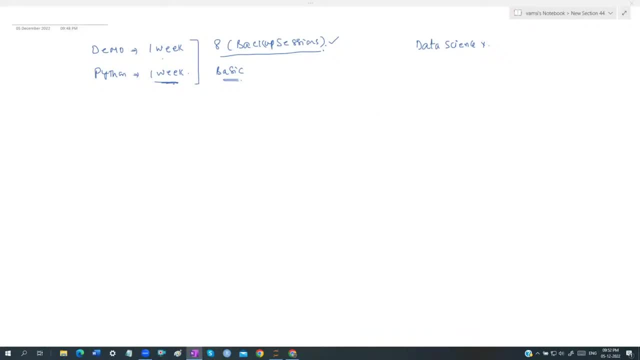 so we expected actually guys actually uh, initially only uh. we have some around 30 registrations are there, but very few guys are start joined for the last class and basically this uh session 9, 30 to 10- 30 we have been planned targeted audience are going to be employees, because so many people are. 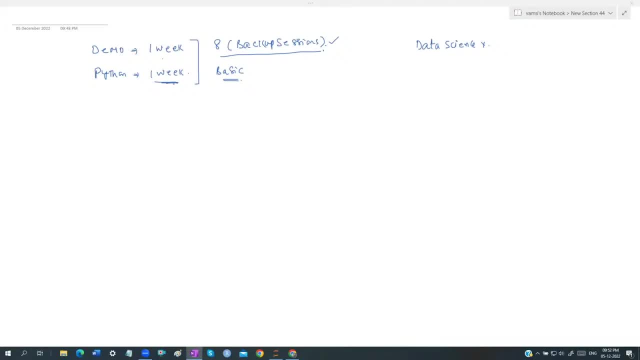 asking for the late night batches. we have been scheduled this. actually, guys, maybe i don't know what is the reason- it may be a short uh intimation or something like that. very few guys have been joined and we expected that more people will be joining uh as part of the registration, but i can. 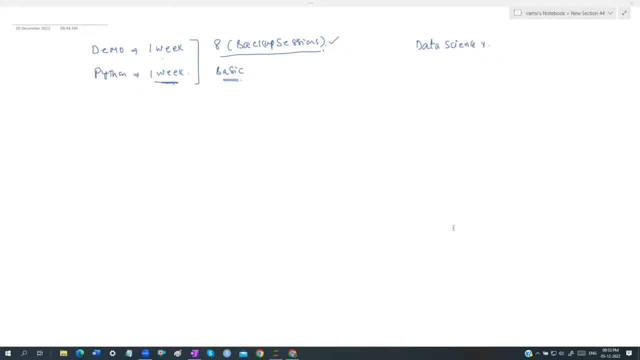 see, but today we have a good number actually, guys. so 20 people. i think 20 participants are there now. including me and my back-end team, it is 17 candidates will be there. sufficient guys: 20, 21, 22, 25 people will be there. so don't worry about the data science classes, guys, because everybody 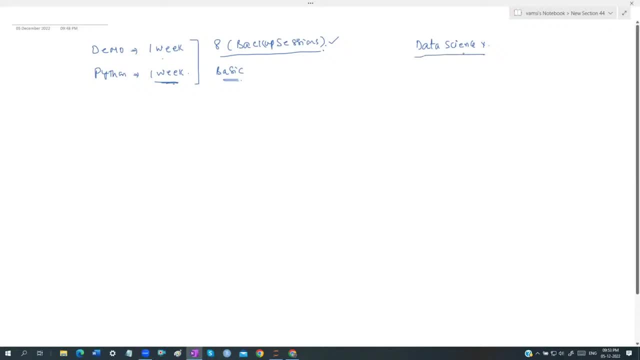 is having an interest. like they, we don't want to study with the python. so what? what we are going to learn as part of the data science? what are the techniques? what are the technologies we are going to learn? i'll arrange a backup session. guys, don't worry, just give me one or two days of time. i'll take a backup session. so today, 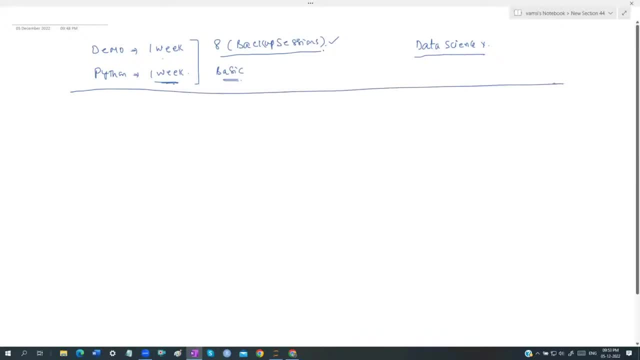 don't worry, even if you are not familiar with the concepts, whatever i'm talking today, don't worry about that, just go through the class. it is only just like a why do you? why, basically, the demonstration is required. guys like to know what is our plan like, what is our schedules like, how we are planning. 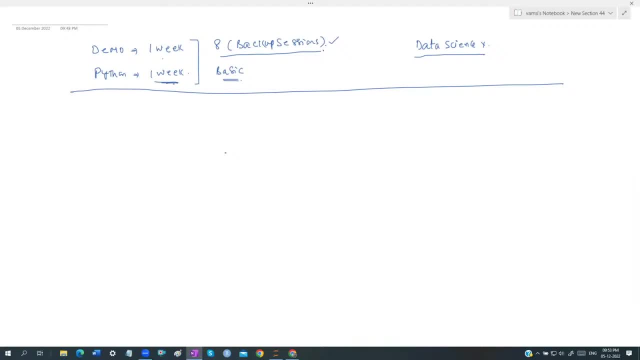 so how my lectures are. there is my. is i'm teaching in a proper way or not? so how is my explanations? can you catch up my accent or not? so to get some idea about that, we'll attend the demo classes right, so after that you will plan it, whether you want to join my class or some other x batch or y batch. 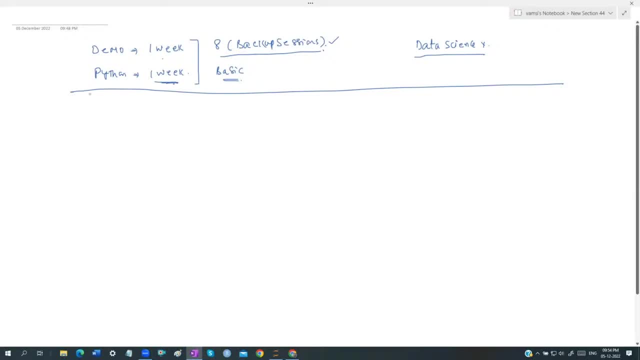 you want to join it actually so being, i cannot directly start with the two days. i don't have any plan for that. actually, let us happen today and tomorrow will just happen. we'll just plan further with the python classes guys, maybe today, tomorrow and day after tomorrow as of my plan, if the same. 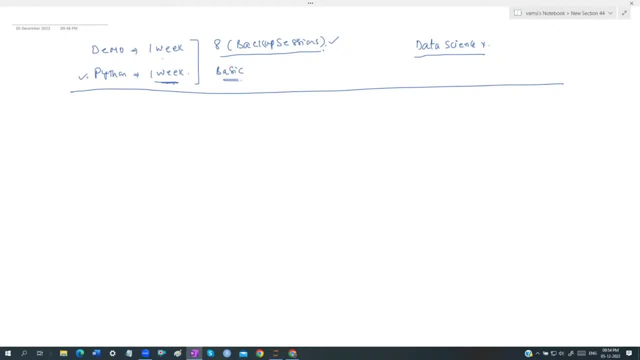 numbers are there: monday, tuesday, wednesday will cover them and i'll break the batch. and thursday, friday, saturday and sunday: i'll take the backup sessions. i'll cover all the things, actually, guys. okay, and being it is already a late night batch, i cannot extend the batch more and 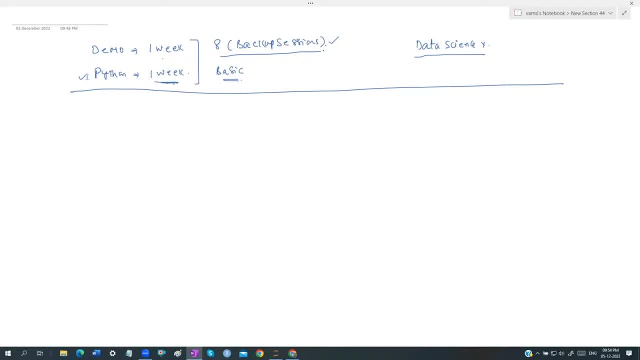 more. that is one of the reason. but we'll try to. we'll try to just make up the backup sessions so that everybody will be on the same page, but today, uh, everybody's not, is not on the same page. some of them are in advanced level, some of them are going to be in. 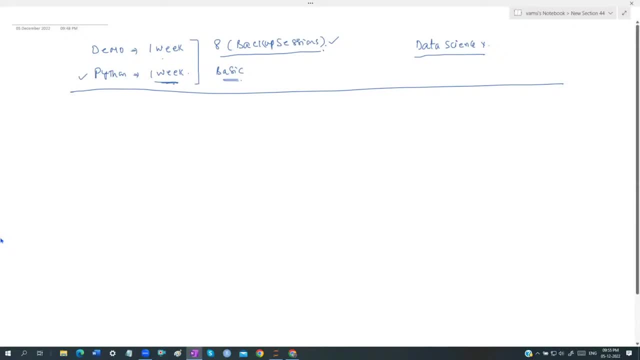 the beginning levels. actually, if you are already having the concepts of python, guys, you can handle that. we can just understand the concept, what i'm talking about, okay, so guys don't worry. who has been joined for the today's class? so please give me just one or two days of time because the batch 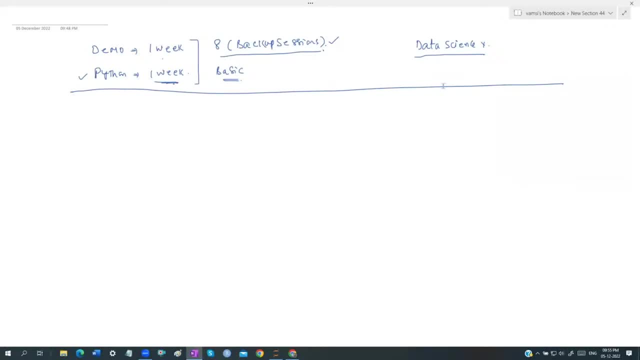 was already started. you may be having a little bit lagging is there for you, so don't worry, i'll take up the backup sessions and cover all that particular. whatever the missing topics are there guys? okay, i'll give you five, ten minutes, uh time i'll give you guys at the end of the class so that 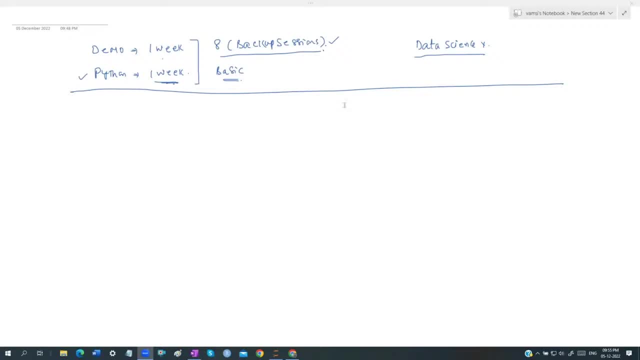 we can have some discussions. we'll have a discussions, guys. okay, right guys? uh, hope all of you understood what i have been explained. guys, fine, guys, so you can use a chat panel. guys, try to answer it. just try to make it interactive. just answer it as s or no so that i can know like. 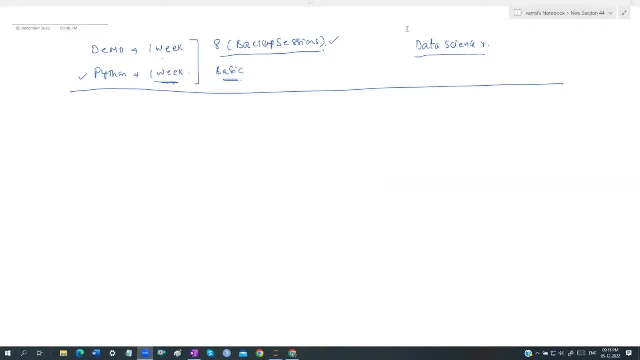 what you are feeling, uh, regarding the my discussions actually okay, so shall i continue, guys? will i continue with the regular class guys? right, i'll. i'll continue with the regular class guys. maybe some of you will already have any ideas about that if you're already having a python. 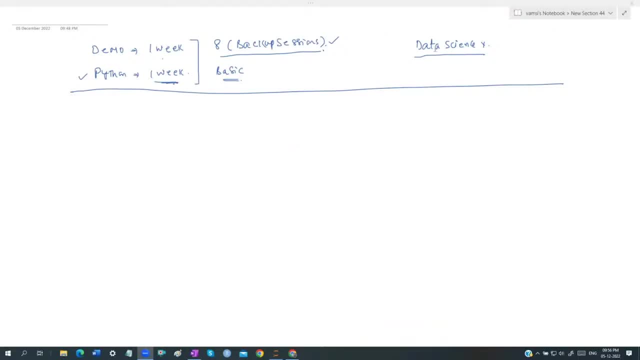 you don't find any difficulties, okay, fine. so, guys, we have been started with. uh. currently our discussion is on the a python concept, which is going to be in python, we have something called as n sequences. actually, guys, normally if you have an idea about a programming languages, 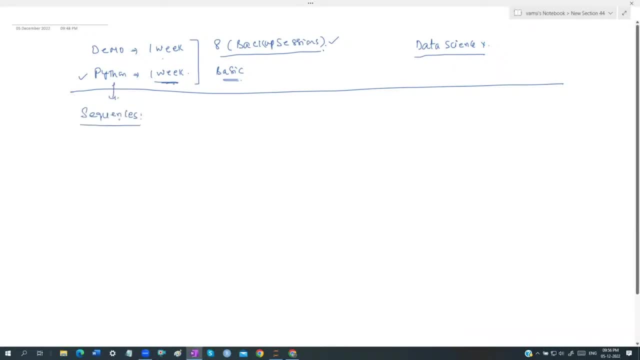 so it's not a python class. actually, guys, we are learning python for implementation of the data science concepts. so some little bit core python is required, guys. two weeks python is going to be required. the two weeks python is only what i'm trying to discuss it here, actually, guys. okay, so in python we have some concept called as n. 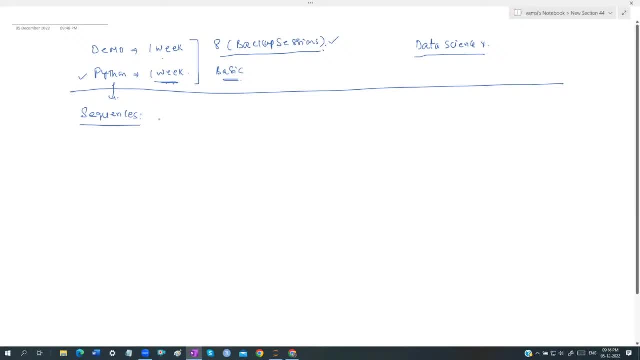 sequences, actually guys, some kind of a data structures which are basically to store multiple values. actually, like, we have something called as a list, we are having something like a tuples, we have a set objects and we are having something called a list and we are having something called a. 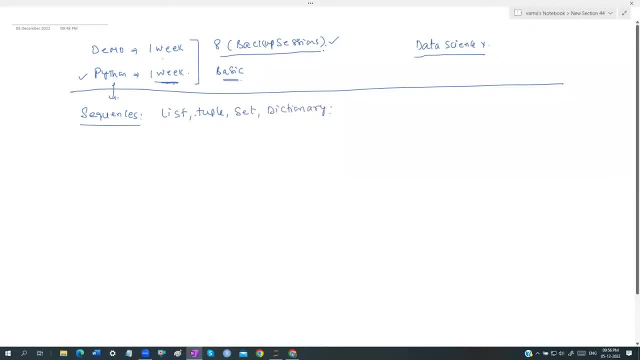 dictionary objects. actually, guys, these are the four basic data structures which we use it in python currently. we have started with the list concept. actually, guys, what is a list? actually, a list is going to be nothing, but it is a collection of some which is going to be some kind of an heterogeneous 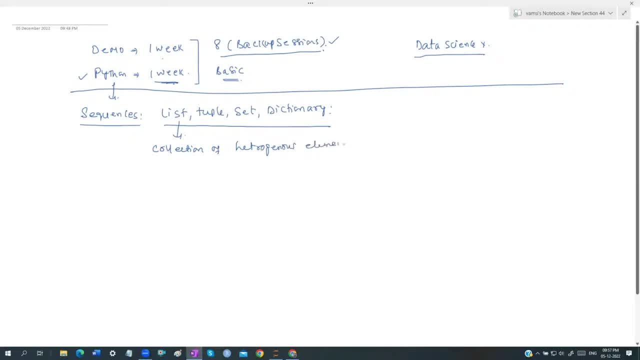 elements. actually, it is not just a single value. actually, guys, it can store multiple elements. those elements can be it. it can be of a different different data types, heterogeneous. how do you create a list? actually, guys, list is created just by enclosing within a square brackets, like in other languages. you need not to write something like list, integer, float, okay, string. 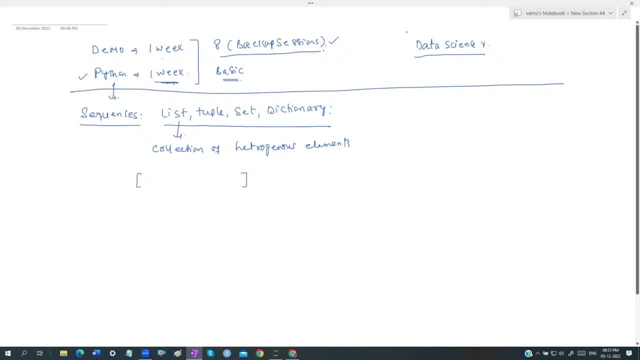 we need not to write it. actually, guys, simply, we are going to put some kind of a square brackets actually. yeah. yeah, i'm discussing, i'm discussing it actually it's nice. just i'm giving some idea about what the what has been happened actually, so list is going to be nothing but a collection of 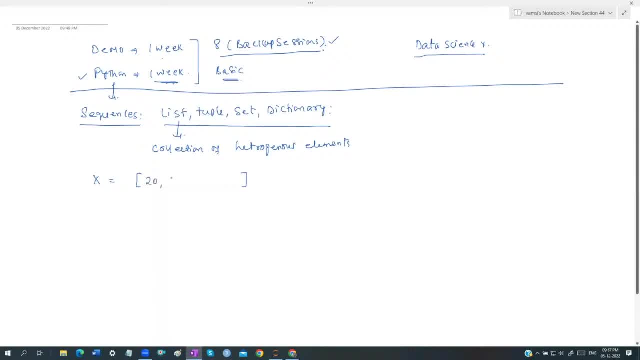 heterogeneous elements, what we are going to be having, actually, guys, an integer and we have a float, we can have a string, we can have a bool, etc. etc. we can have it actually, guys. so this is: how do you create a list to manage this list, actually to manage the list? what is meaning of managing of? 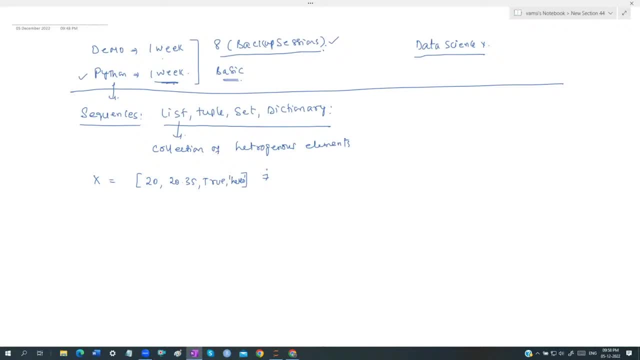 list. actually, guys, we can add some elements, we can remove the elements, we can modify the elements, so we have to require some kind of a methods that are required, actually, guys. so very simple guys. i have discussed only four methods as of now. i discussed only four methods, actually, guys. so if 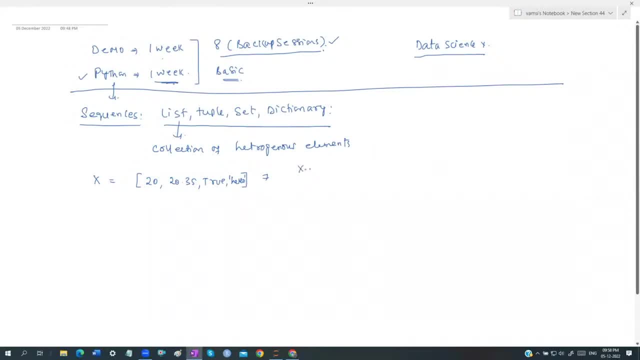 you are already having an idea about object oriented guys. well and good. who has already having the idea about object oriented? even if you do not have any idea, just understand them. i'm going to discuss about those particular applications later, actually, guys. so i have been got discussed about what is a method? actually, guys, method is nothing but just a function which. 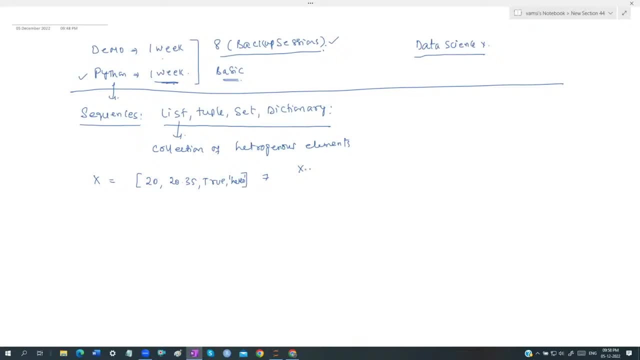 is used to do some management or a manipulation with that list of elements. so i have discussed, actually, guys, the method to do, whether there are elements or the list, which is not actually the method to do, I guess are not. deswegen, that is going to be a list, in case if a list actually 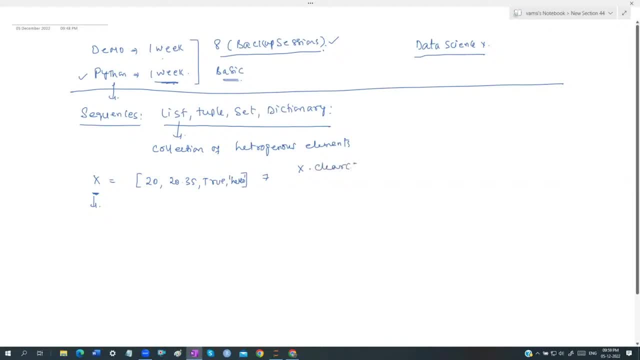 rescue. so here, next slide. i want to get into it. so in here we will talk a little bit further about the list: actually guys. I am writing down the numbers, that psi actually guys, and that siblings actually guys, for example. if si, is it? so this is a proposed example. i say: that if one line i take it away from 1 line, its required this number right the line i received. you guys and you remember i just used this one line with Favorl to correct numbers in the previous hunters樹 smart. so i don't think these two lists in your algorithm will pronounce. 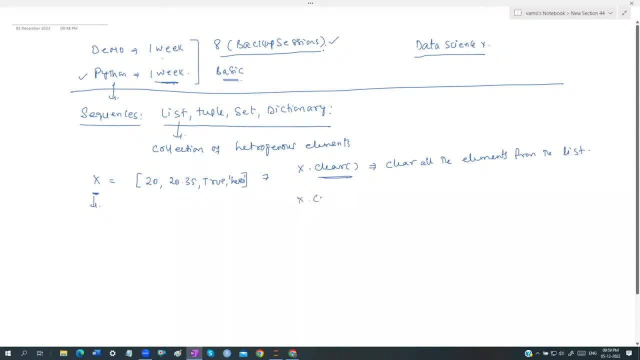 blank if any of them isn't there now. right now, here you can see the list, actually, guys. so, for example, call it as a clear method, and apart from that, i have been discussed about a method called as account. you have to give some input value. whatever the value we have been given, it will gives you the 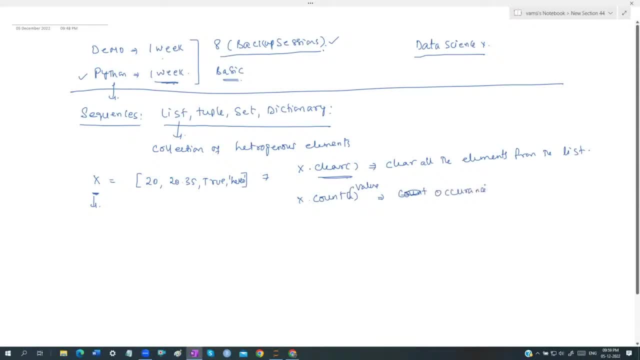 count the occurrence, how many times that particular value has been got. occurrence actually guys, the occurrence of the value in the list. so at least i'll expect guys like who has been joining for the data science, at least they will have some basic knowledge of programming concept. so at least i expect that at least we have some minimal knowledge of programming so that it's a. 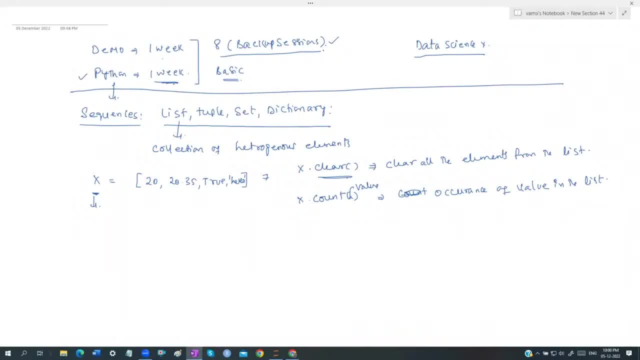 person who is completely without having any knowledge on computers. they don't prefer to learn a data science actually, because data science is completely a little bit higher level concepts, actually same as it is. i have been told about a method called as a pop method. actually, guys, pop is going to be nothing, but what it is going to do is it is going to remove the element at the 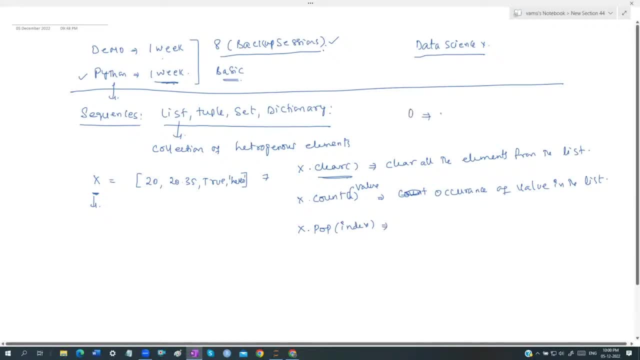 given index. normally, like a pop method is going to remove the element at the given index. like other languages index, start from zero to n, from the left to right. don't worry guys, it is also from right to left also. we can talk about them. don't worry about that right to left index also. 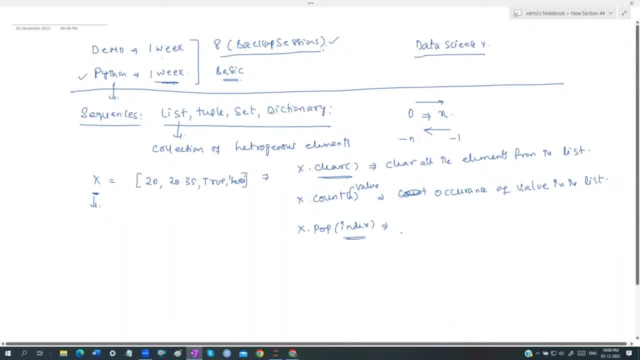 we can define it actually, guys, it is indexed ways: it is going to remove the element actually, yes, it removes the element at the given index, actually, at the given index. it is going to give: removes the element actually, yes. and then we have been got discussed about x dot remove. i'll just show you. 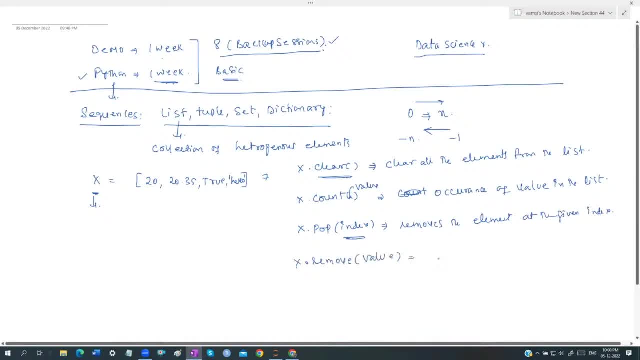 next number, we have a array of several different leaves of the list of scenarios. so now, the first time you remove the element, it removes the element d're. same lesson in is that if you give an alignment of, of of the first occurrenceotes, for example, one do when 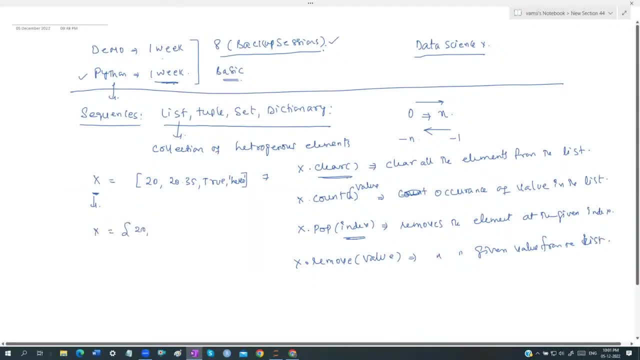 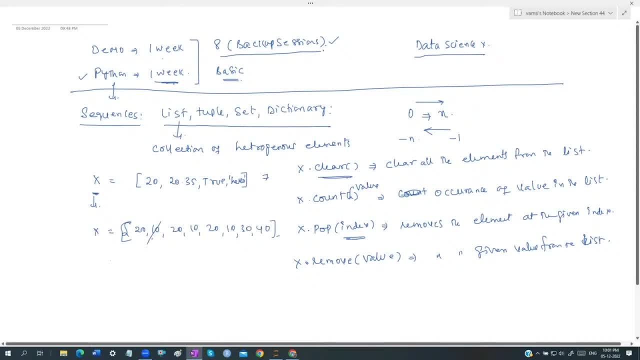 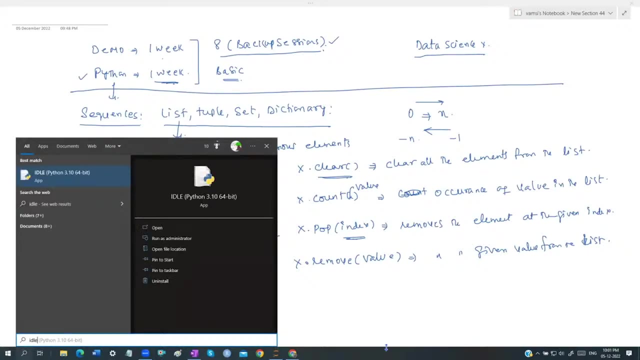 only this 10 will be removed, but not all the 10s. only the first occurrence will be removed. actually, guys, we are completely in the beginning, concepts only. guys, i didn't started with any complicated work. actually, we didn't started with any main work also. okay, so this is a very simple installation. 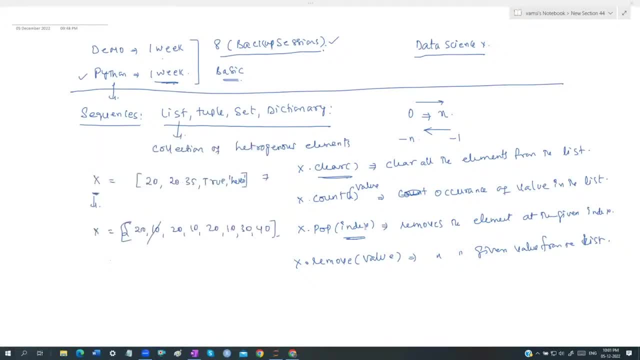 guys, installation of python is not a complicated one, so this is going to be a simple installation of python installation. i'll show you later the backup sessions, i'll arrange the backup sessions and i will explain it. actually, guys, i'll arrange the backup session, guys, as soon as possible, don't. 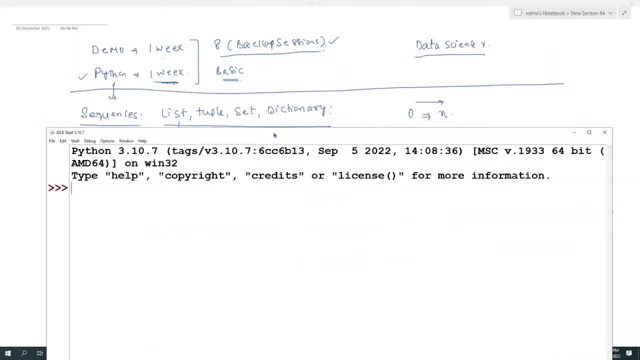 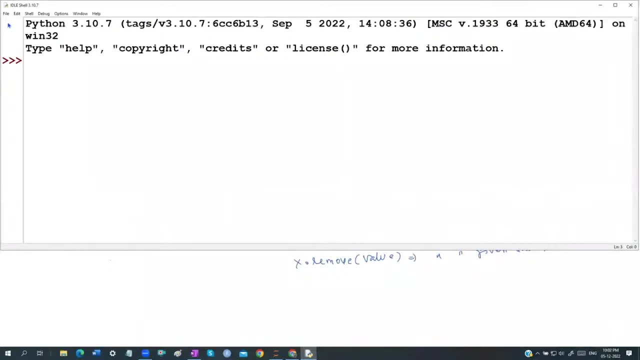 worry about that. okay, so fine. so this is going to be what i am going to call it as an ideal. actually, guys, i'll tell you about more, about the ideal which comes along with the python installation only, which i have done: the python installation, along with the python installation, only i have 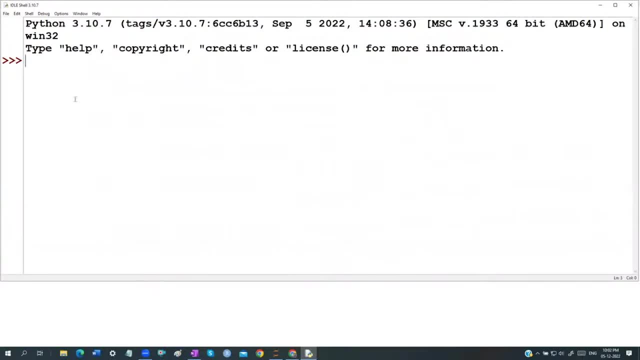 got this particular ideal. actually, guys, you can see a prompt like this. actually, yes, we can see a prompt like this, actually, guys. see, guys, how i'm creating: x is equivalent to nothing but 10, which is a true, i said, which is an hello, and which is going to be something like n 20.45. actually, guys, it's a list. actually, yes, i'll tell. 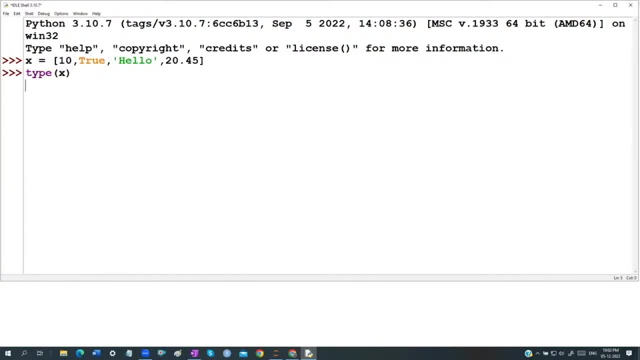 you all the things, guys, don't worry. just it's very simple, simple topics only, guys. i didn't started with any complicated topics actually, so in like in other programming languages, we don't require any declaration part in python, because python is a dynamically typed language. guys, like other, 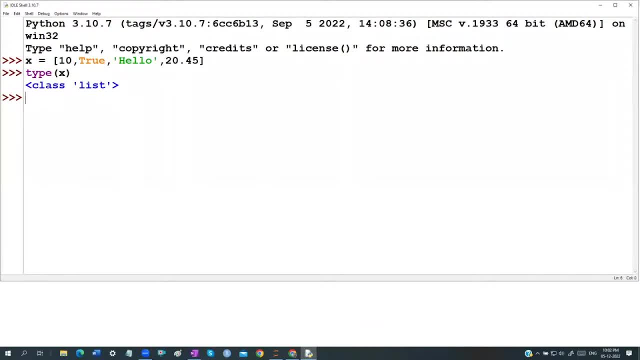 programming languages you don't declare in other languages. we'll declare it. no, guys, like: which is going to be something like an. it's an integer, it's a float, it is going to be a bool. we'll do it. no, guys, in python, we don't do it. actually, guys, i'll tell you guys, it's one of the feature of python which is: 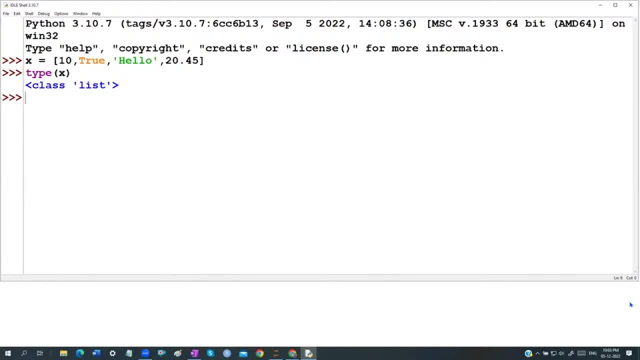 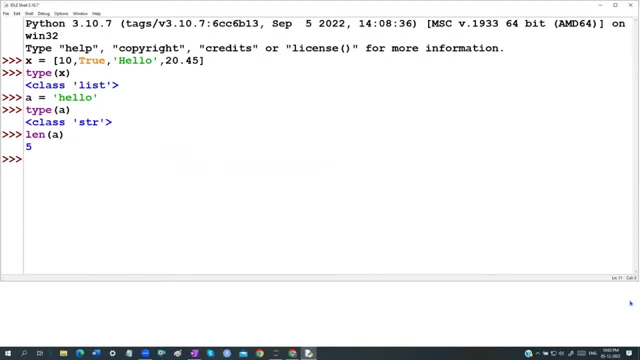 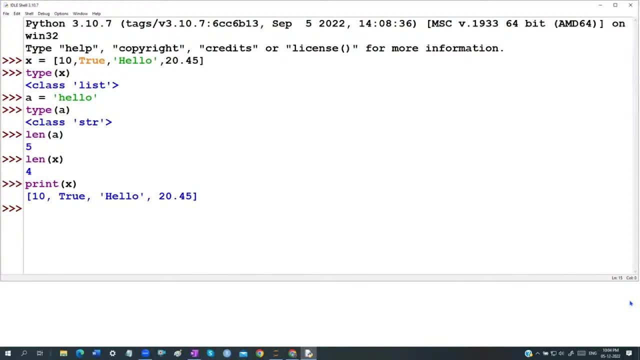 simply it is going to be x and print x actually over. you can see it actually, guys. so if you want to remove the elements, let me count it actually, guys. how many times 10 was there. you can see the count actually, guys. it was there for one time x dot count of 100. it is going to be there for. 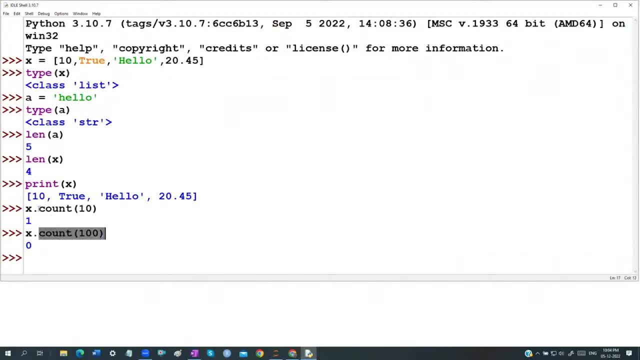 zero time. these are methods actually, guys. these are what we call it as methods. so the guys who are already having the idea about object oriented, they may knows about this. even if you do not have the idea, don't worry guys, i'll explain. i'll take a backup session, so i'll complete of that. 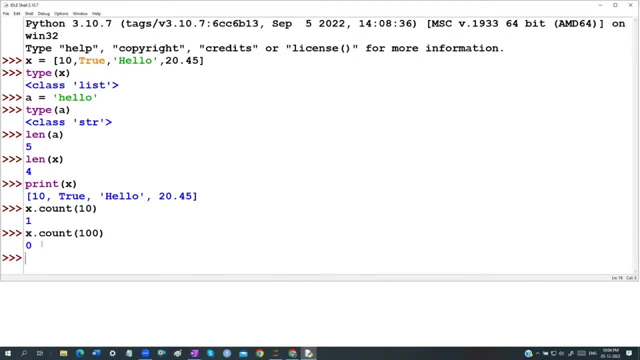 x dot count of 100. actually guess 100 is not there so we can see the zero value. i want to remove the elements. actually, guys, x dot pop pop is basically based on the index base. removing, actually guys, index base means which one? zero, one, two, three. like this, we can specify that zero, one, two, three, even. 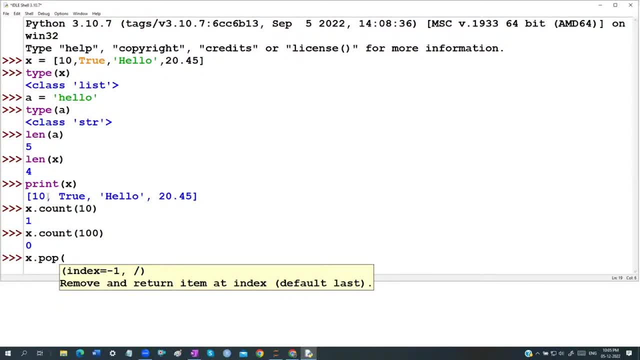 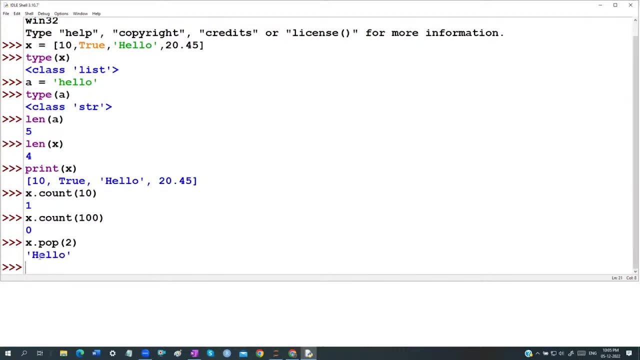 we can write in reverse order. actually, guys, this is minus one minus two, minus three minus four. it is from left to right, right to left, left index. is there? if i said x dot, pop of two? actually, guys, the second element will be removed. second index: 0, 1, 2. hello will be removed. actually, guys, it will tell you like what value has been. 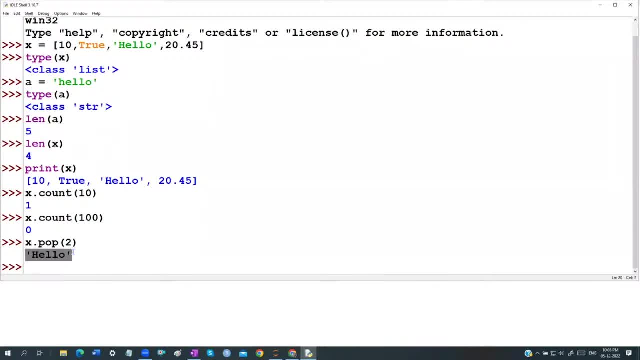 removed. also, it is going to tell you don't think that it is only returning the date. actually, guys, that particular 22, the element that 2 has been removed and written the value actually. so now, if we can see x, you don't see the hello. actually, guys, previously the length of the x is going to be 4, but 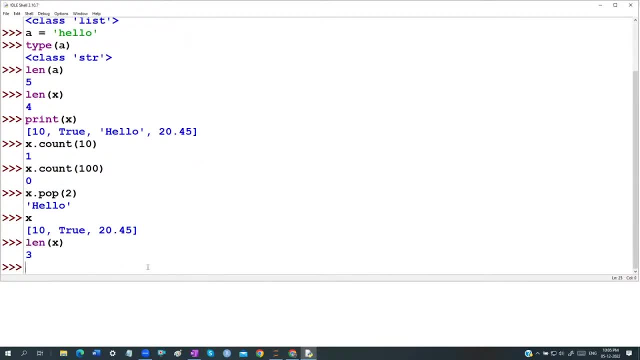 if we say length of the x is equal to 3, actually, guys, why? because you can see one element has been got removed. so pop is basically on the index. if i don't specify which value we have to remove, it automatically removes the last element. actually, guys, it automatically removes the last element, x. 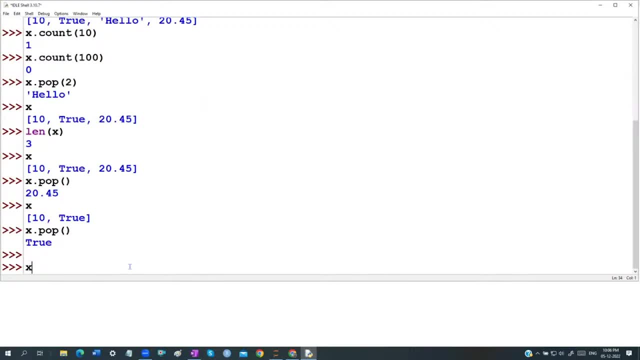 dot pop. it removes the last element. actually, that is going to be what we are talking about: the pop method. once again, i'll create it: 10, 20, 10, which is 30, 20 again at 10, 20, 20, 30, whatever you want. we can give it actually no worries. now i can say x dot, which is going to 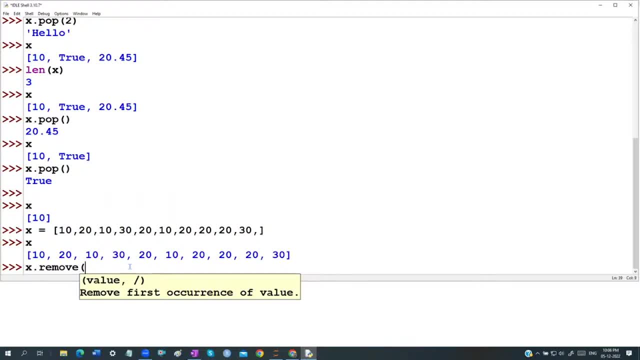 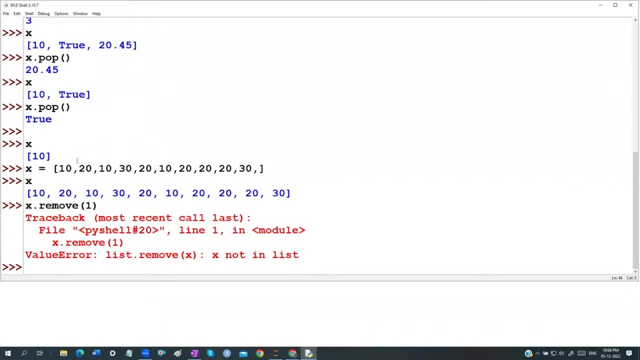 be remove. remove is not based on the index, guys. it is completely based on the value. if i say remove of one, you will get an error. actually why? because one was not in the list. index pop will can do that, actually, but remove can't do that because remove is value based. actually, guys, x dot. i said remove. 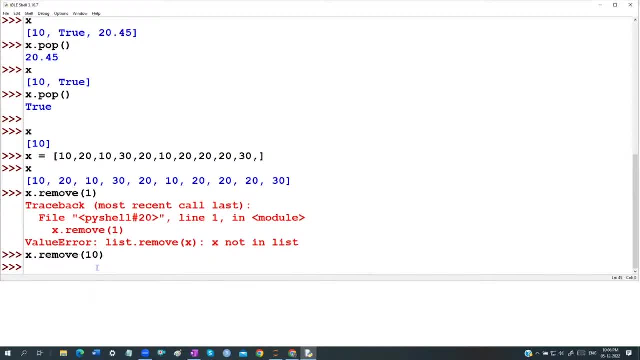 of which is going to be 10. only the first occurrence of the value will be removed. it won't remove all the 10s. 1, 2, 3 10s are there. so out of the 3 10s, 1 10 has been got removed. 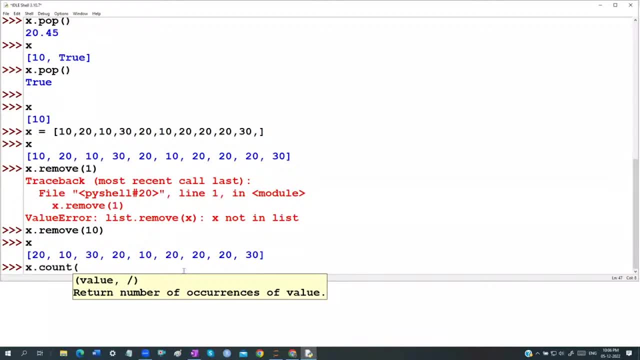 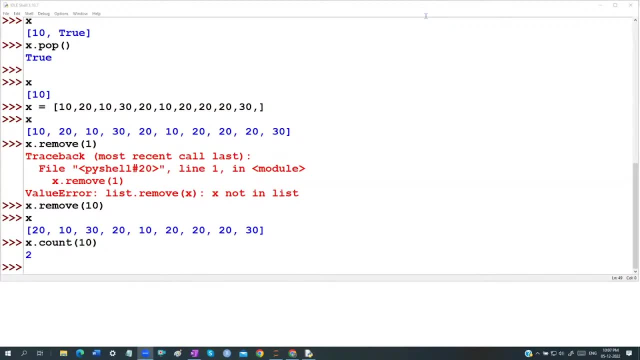 now, if you want, we can count it. actually, guys. x dot count of 10. we can see the result is going to be 2. is the result what we can see? it actually okay, so something like that. we can see that. so these are the four methods i have been got discussed actually on saturday- very few guys.